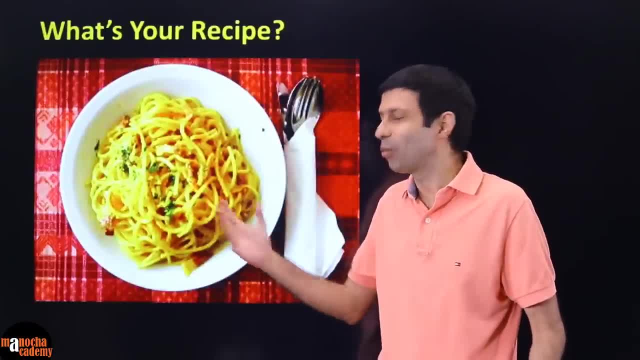 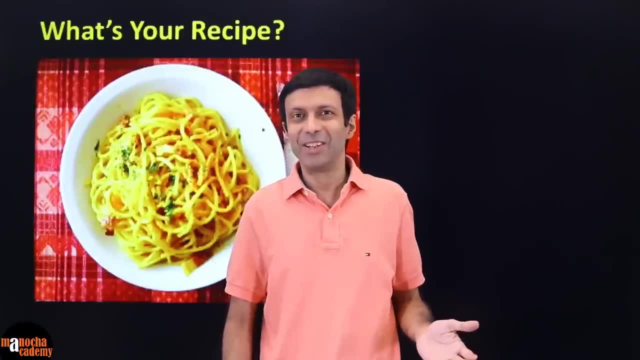 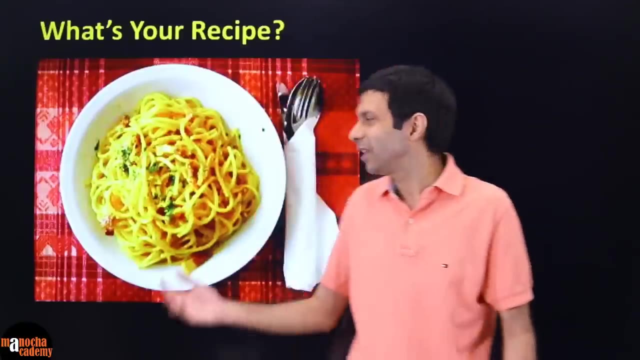 looking at this picture, I am feeling hungry. but if you are feeling hungry and you quickly want to make some noodles or your mom is making noodles, she, you or she follows a recipe right so to everything that you do in the kitchen, there is a recipe. or if you are baking a cake, there is a recipe. so what is the? 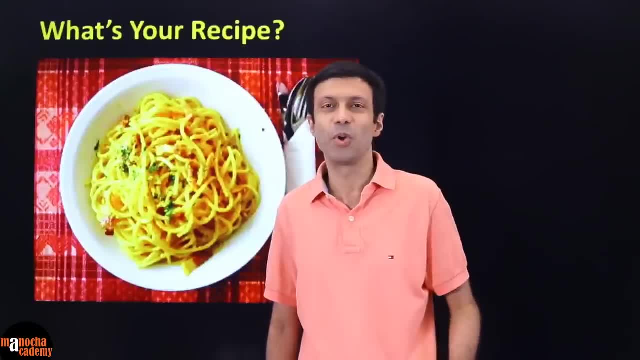 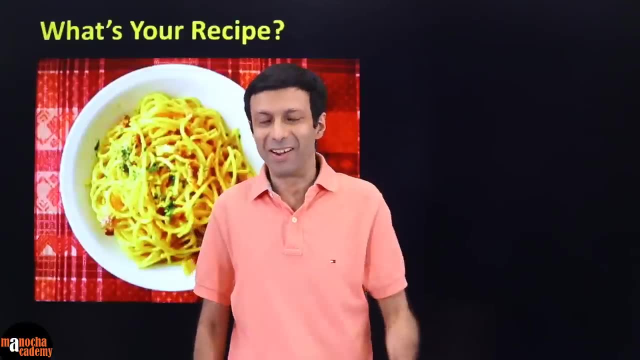 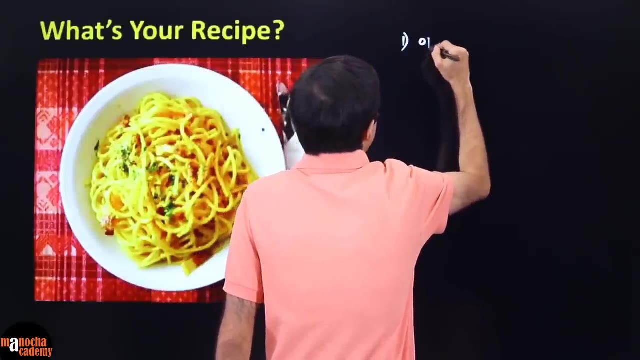 recipe when you are making the noodles. can you guys tell me? so what do you need to do here? so let's say you're making these instant noodles, so what is the first step? obviously you will cut the packet and boil the water right, so we can say: we open the packet. 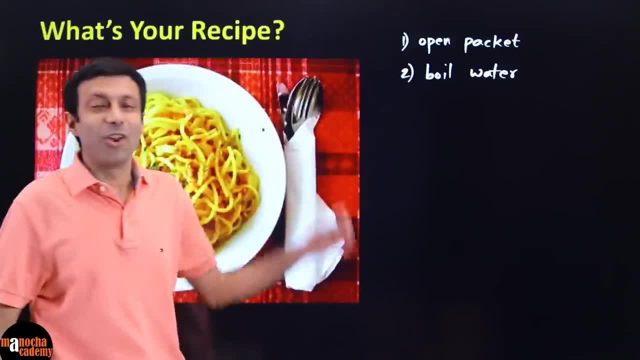 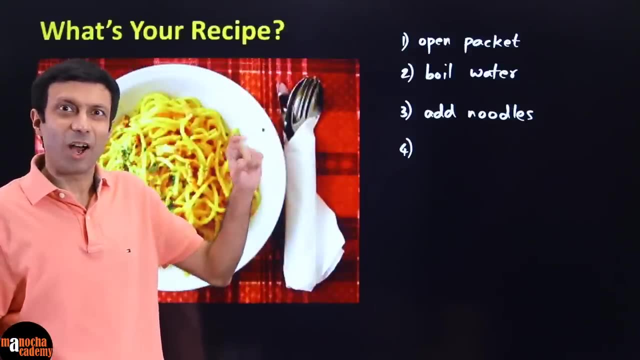 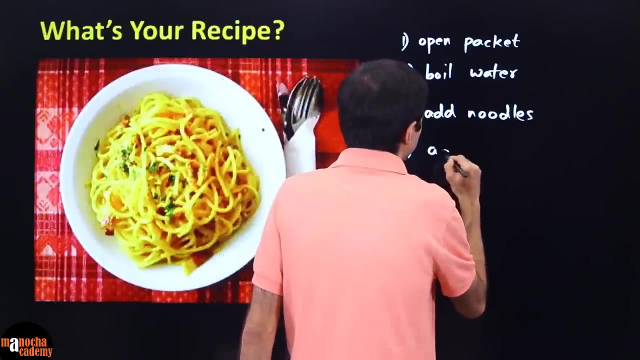 we boil the water and then obviously you will add all the noodles in the boiling water and then you, after its mixing. now you put in the masala, the spices, right, so it's more like a cooking class today. so then you add the masala or your spices. 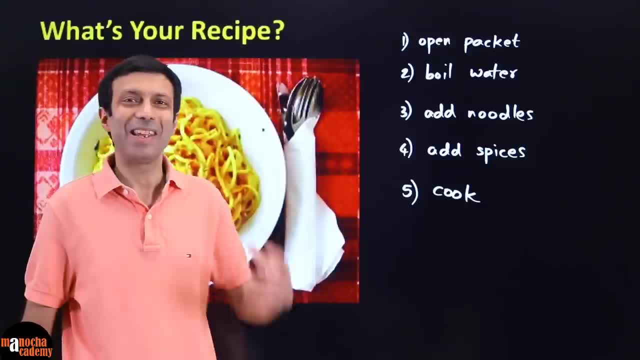 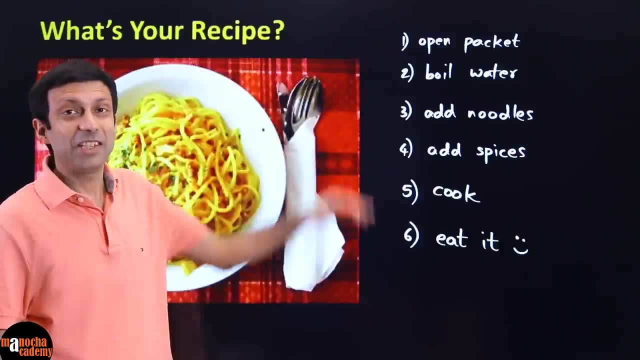 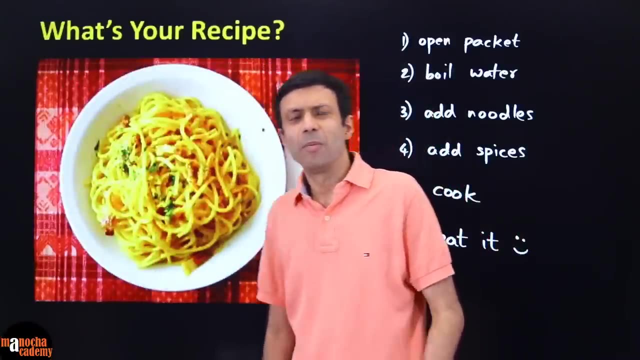 and you keep cooking it till it looks nice and yummy and you stop it and enjoy the noodles. so this is the recipe, right? these are the steps that you follow while making noodles or instant noodles. but suppose, can you change these steps? can you, you know, add spices first, then open the. 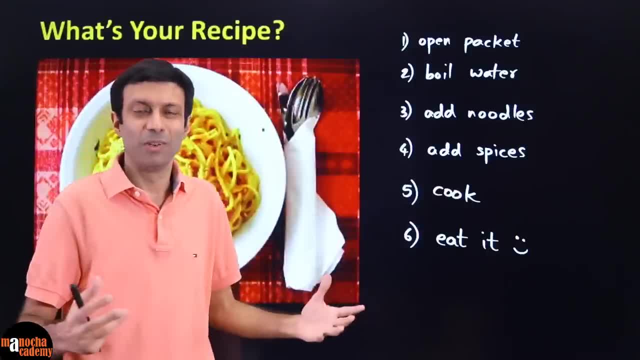 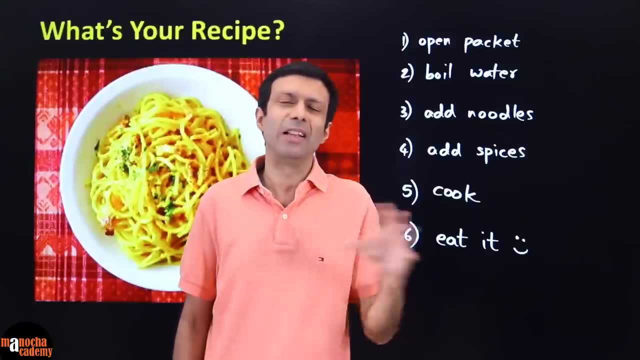 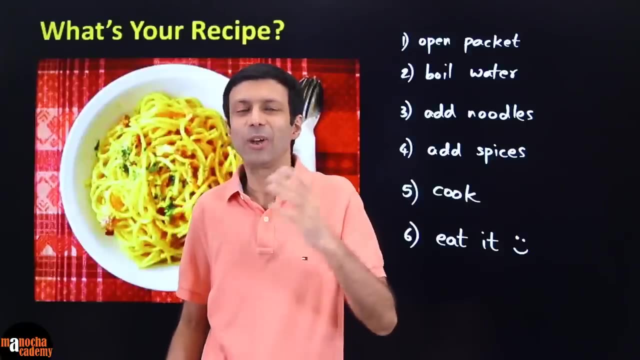 packet then boil the water. you know if you do that you won't get these tasty noodles, and especially in cake recipes. if you make one small mistake, either the cake turns out to be hard or you know there's no sugar in the cake. it's not sweet. so any ingredient or any step you miss. 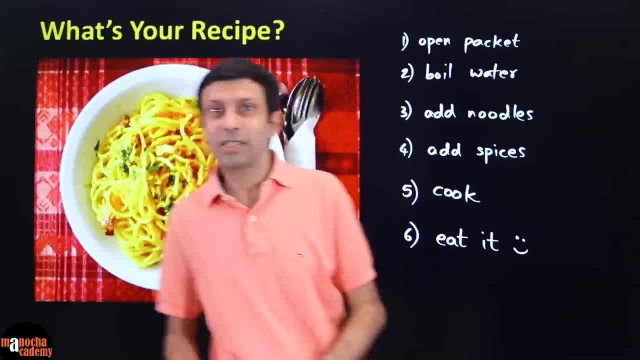 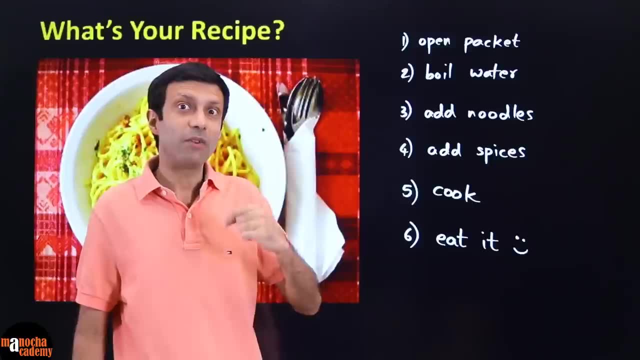 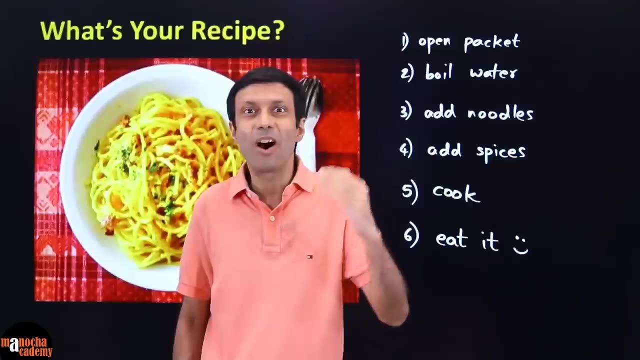 the recipe is gone right. so that is why, just like in the the kitchen, you follow a step-by-step procedure, a recipe. similarly, when you're writing code, when you're writing what is code- code is instructions to a computer to do something- you are giving the computer the recipe or you are writing the recipe for the computer. 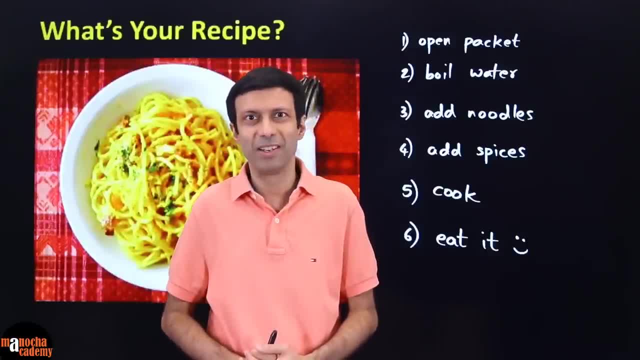 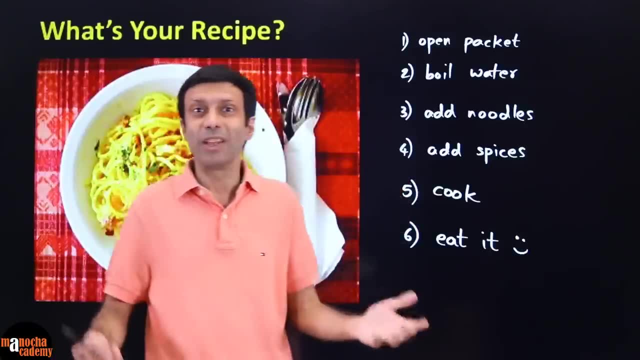 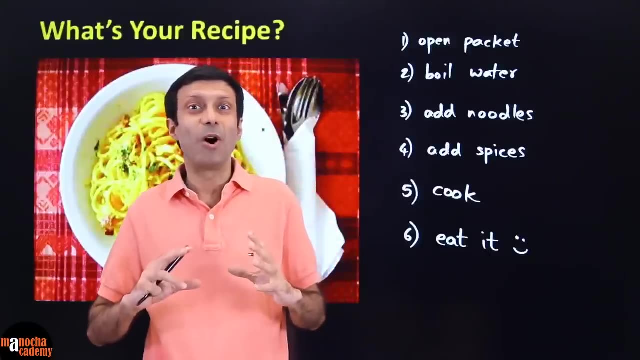 so that it does exactly what you wanted, right, just like exactly what you expected to the noodles to taste. you get it if you followed the recipe. or you know, when the cooking thing goes wrong, mom will say: you didn't follow my recipe. similarly, we are going to learn how to think about not cooking. 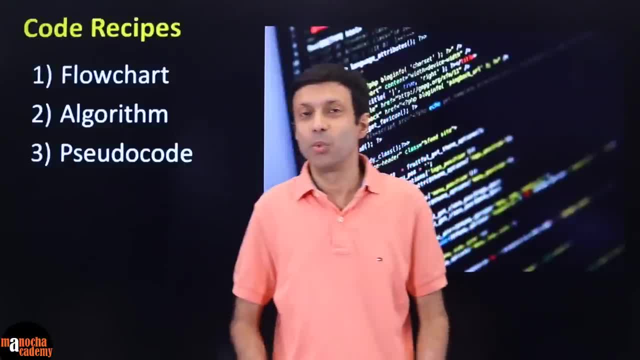 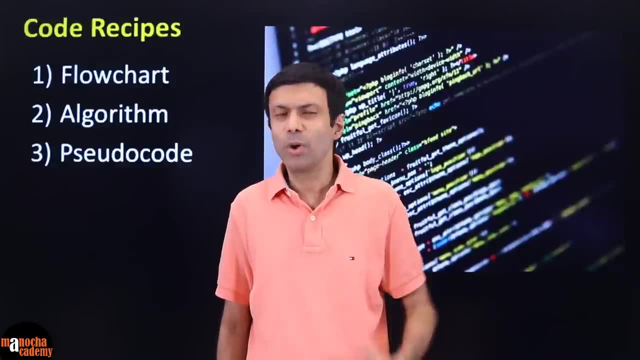 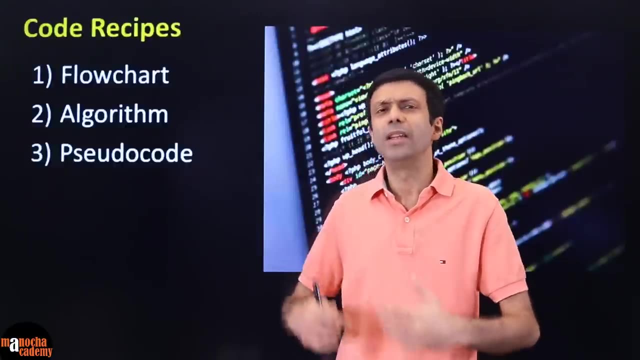 recipes, coding recipes today. so we are going to talk about code recipes today and code recipes can be written in different ways. what is the meaning of a code recipe? so the moment you are, you know, let's say you want to design a program, whether it's a game, 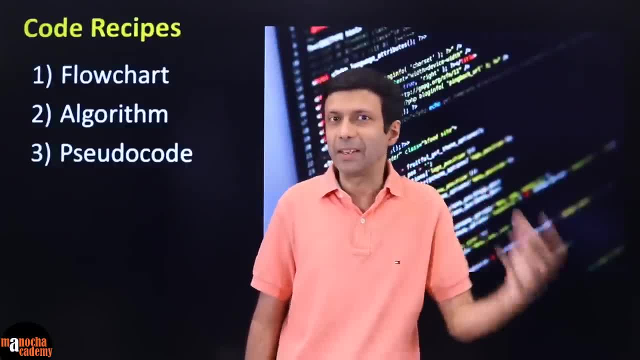 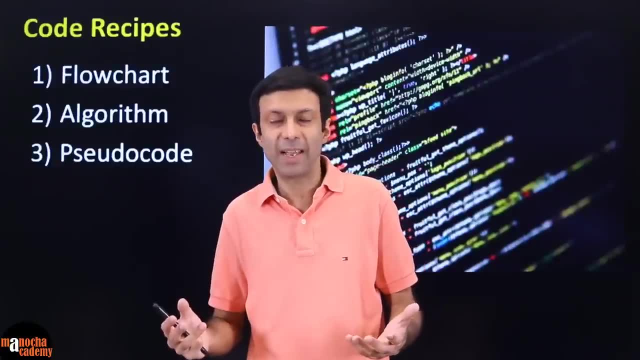 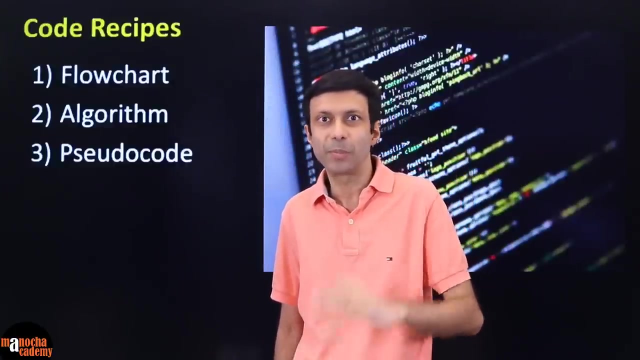 with rolling of a dice, or whether it's you know, doing some income tax calculation or finding out you know the average marks of a test, any of these things. always, you don't immediately start writing the code, especially the program is a little complicated, right. what you do is you think of what will be the steps, you break down the code into steps and 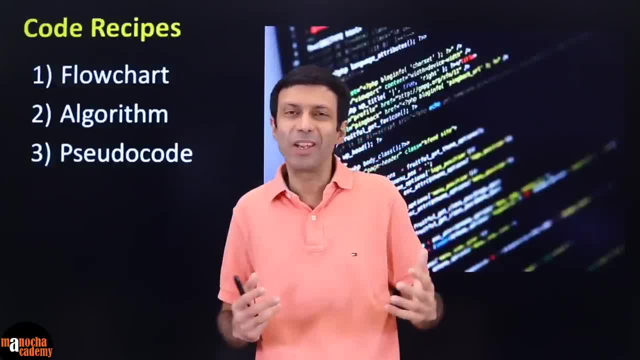 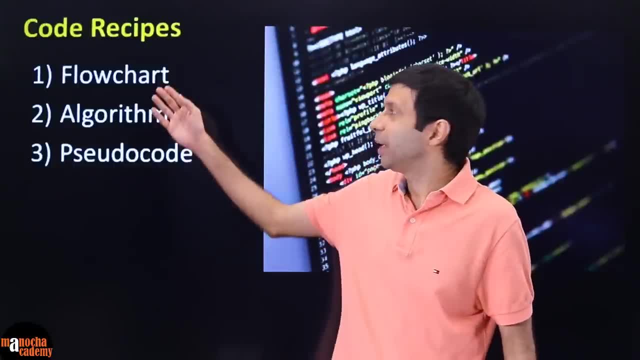 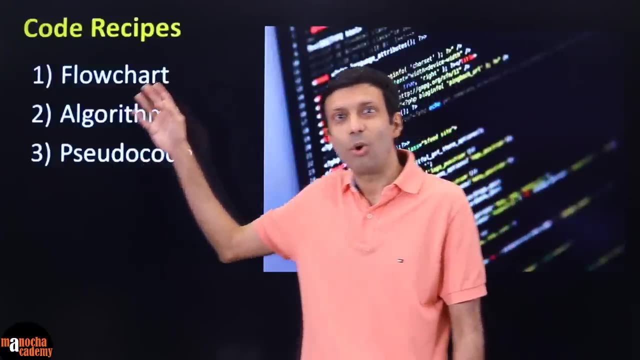 those steps need to be in the correct order. so that is what we call in, you know, informal way, as code recipe. now, code recipe can be written in different ways. it can be expressed as a flowchart, you can write it as an algorithm or as pseudocode, and we are going to discuss all these three styles. 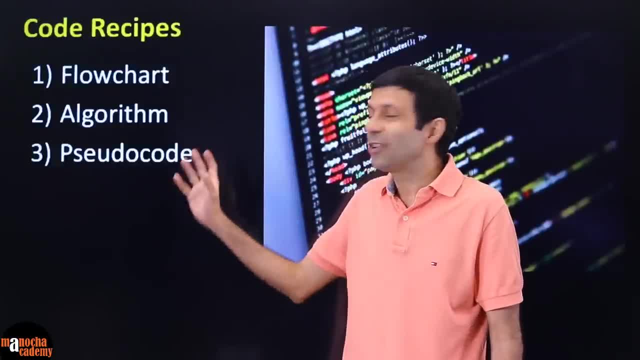 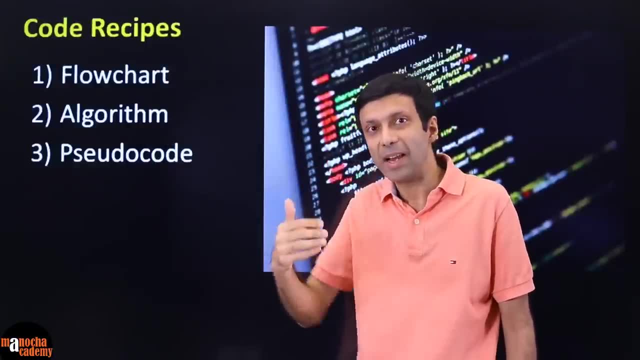 of recipes today, so very, very important class. so at the end of the class you will learn to think like a coder, like a programmer, and these techniques will help you plan out your recipe before you write the code. so what we are learning today is not just about the code, but about how to write the code. 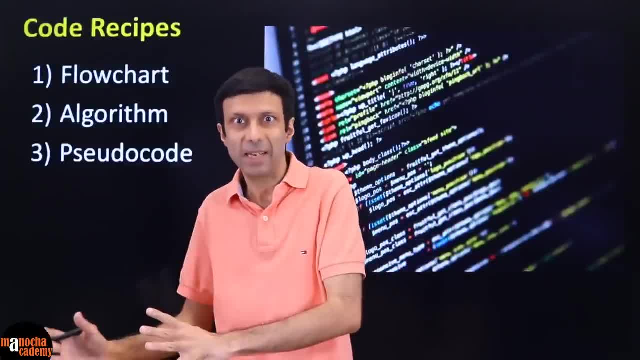 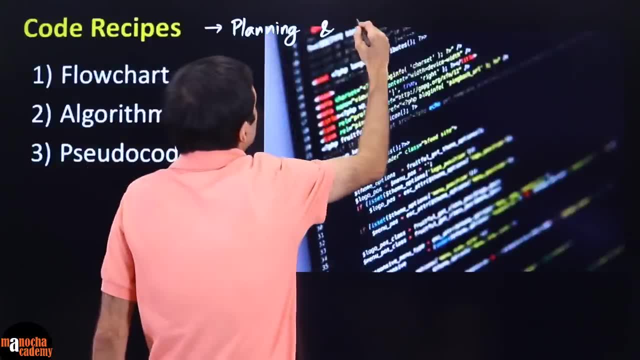 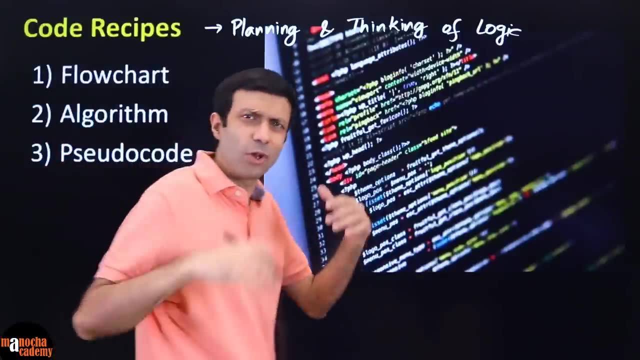 not coding. we are learning the thinking, the planning step. so in code recipes, what we are learning is planning and thinking of the logic. and you think this is important. this is super, super important, because if your logic is wrong, just like if the building plan is wrong, the 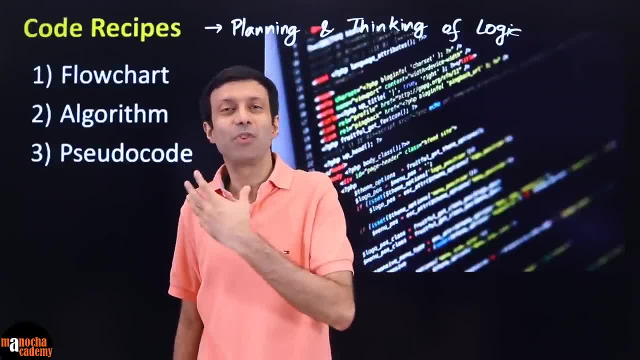 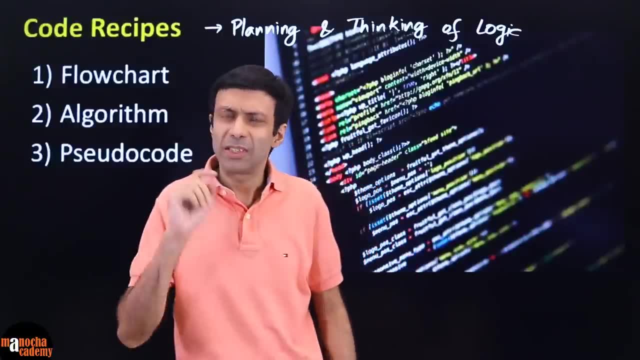 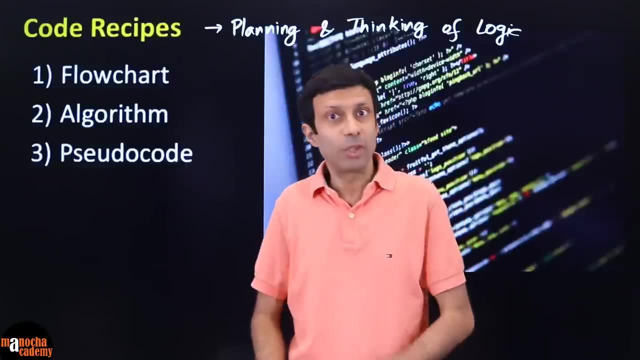 architects plan is wrong, the building is not right. same way, if your logic or your plan is wrong, obviously the code will not do what you want it to do. so thinking like a programmer is very important, and let's learn these techniques, which will help us express the recipe. so it's important for us and for anybody else who wants to know what. 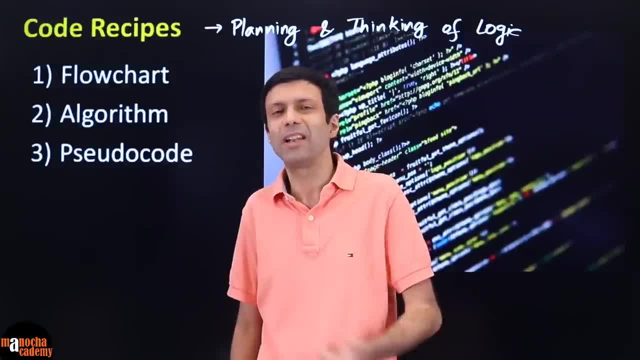 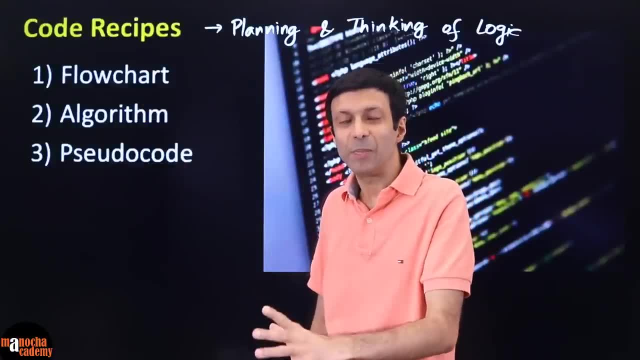 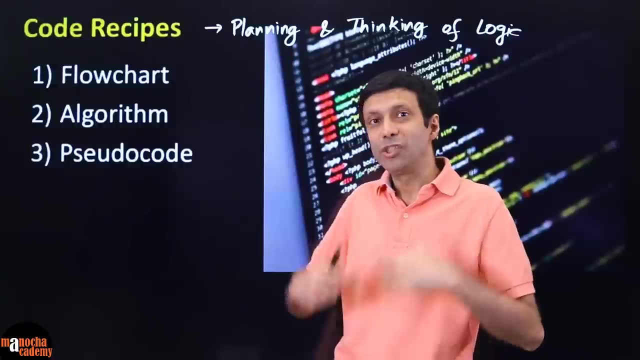 our program will do. he may not know the language that you're coding in, like, for example, he may not know Java. he may not know Python. same way here: if they look at your recipe, they will get to know, even though they do not fully understand your code. it's just like you know when. 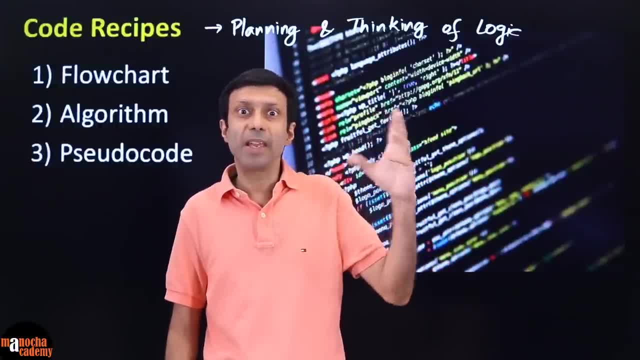 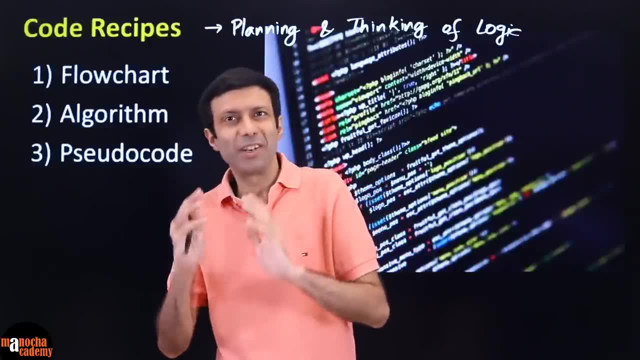 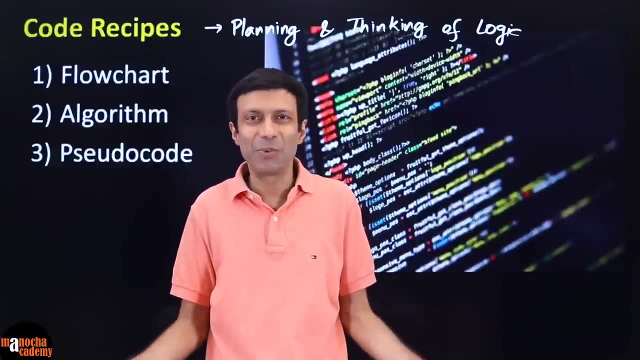 JK Rowling was writing Harry Potter. she was brainstorming and thinking of the ideas, what story to write. it doesn't matter whether she wrote it in English, whether she wrote it in Hindi or, you know, Spanish, German, because now it has been translated in all the languages of the world. 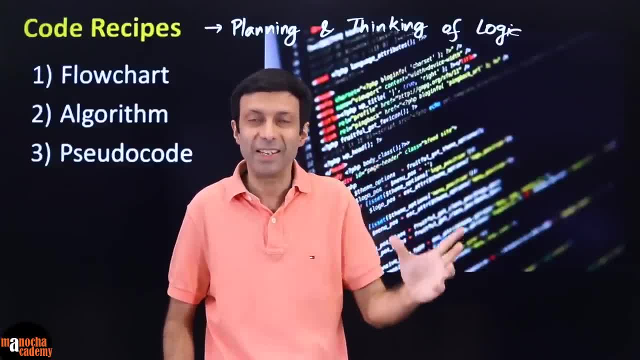 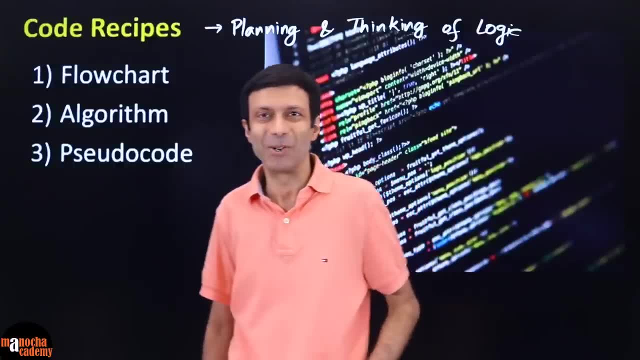 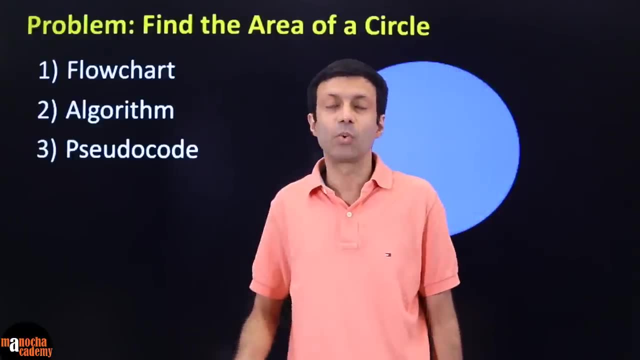 right. so the language doesn't matter, it is the thought, the ideas. so same way here. it's not the coding language, it's the recipe that matters, and we are going to discuss about it. so we are going to understand what is a flow chart, algorithm and pseudo code. with a very simple example, let's say: 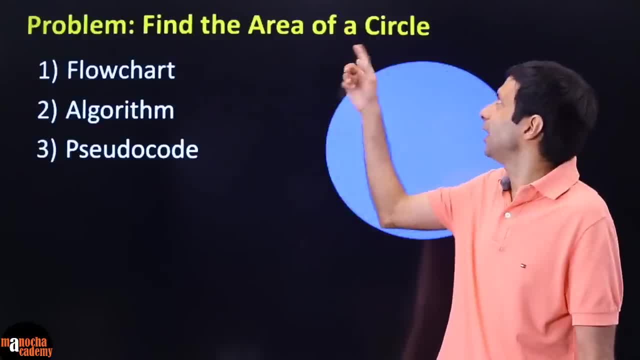 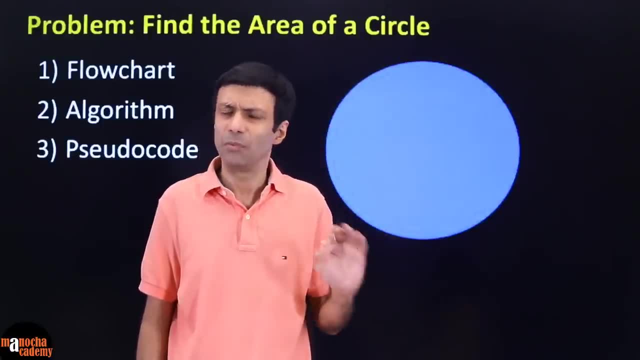 the question given to us or the problem given to us is: find the area of a circle. so we want to write. the goal here is: we want to write a computer program to find the area of a circle. we'll start with a very simple example. now, when you want to find the area of a circle, what does the computer? 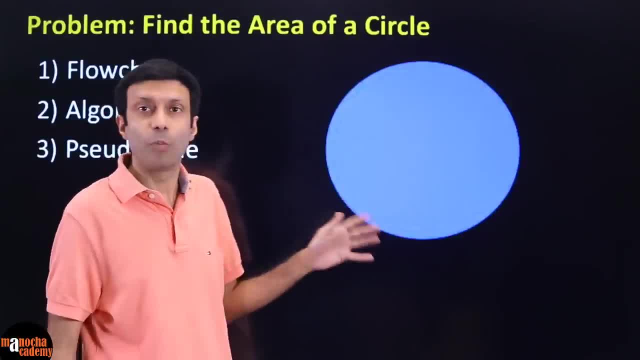 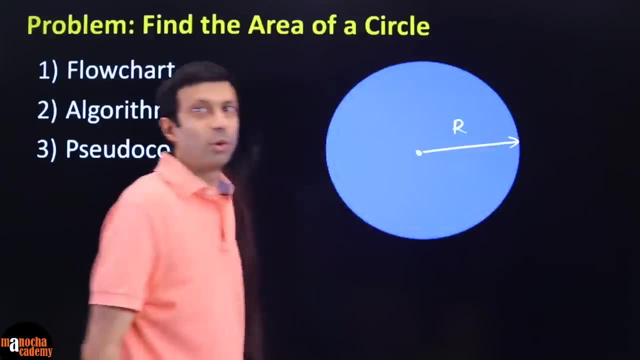 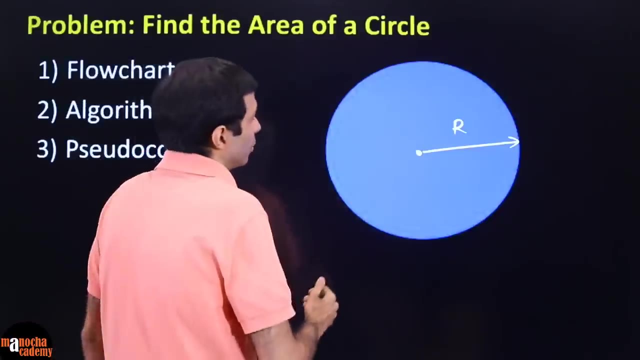 need to know. first of all he needs to know how big is the circle. so what is the radius of the circle? right, the computer needs to know what is the radius of the circle. so that must be supplied to it and then you calculate the area. so the radius of the circle has to be input to the computer and then it will. 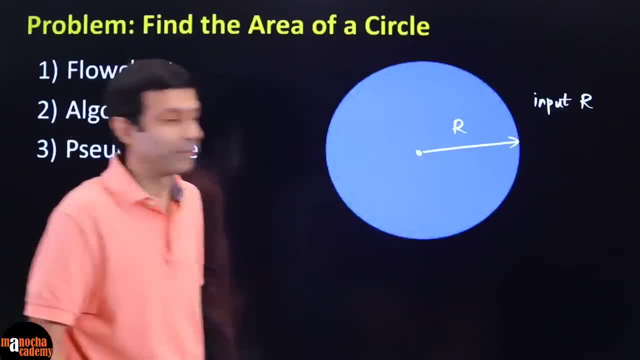 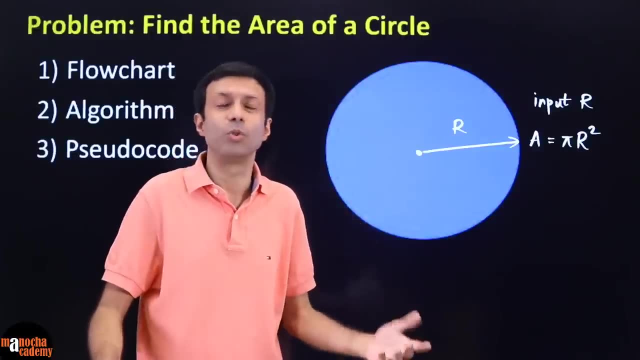 work out the area using the formula. area is PI R square. but does the computer know what is the value of PI? computer doesn't know. we have to supply it. what value you want to use? 22 by 7, 3.14. what value you want to supply here? usually in the computer you have to supply it to the computer. but in the 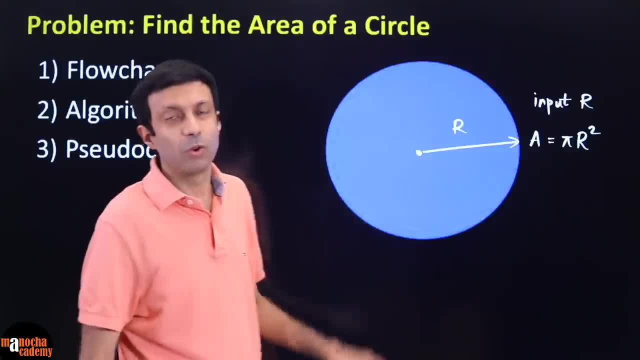 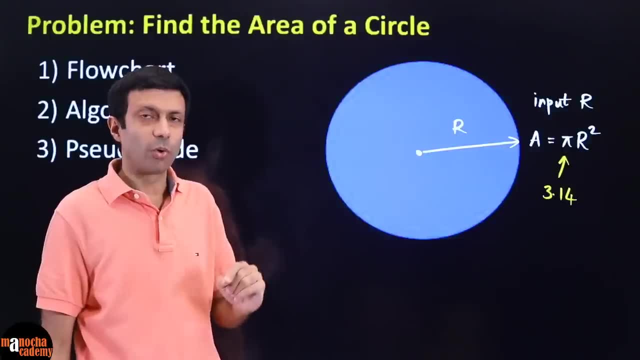 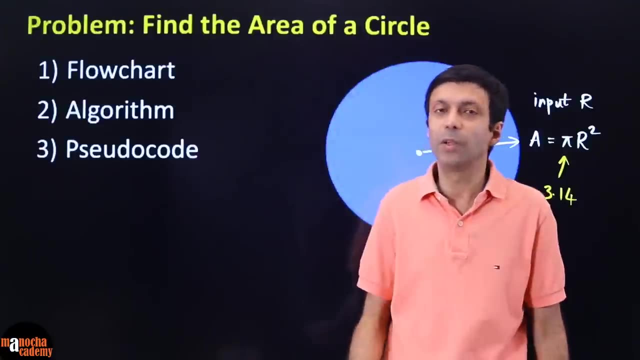 computers we use decimal values rather than fractions, so maybe you'll be substituting 3.14 here. so the goal is clear: we need to write a code or a program to find the area of a circle. but we are not going to do the coding, we are going to do the planning of what will the program do. 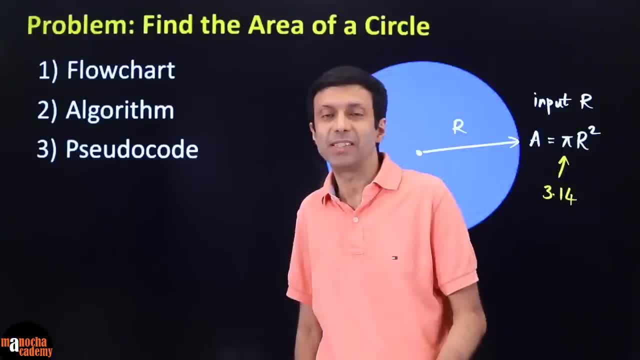 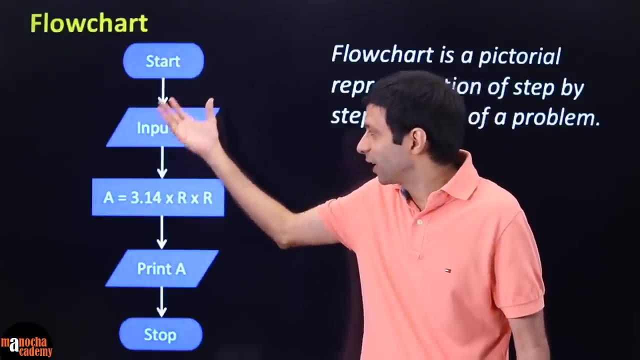 using flowchart algorithm and pseudocode. so let's take a look at, because these are all different styles of writing, the logic, the recipe of the program. so let's understand the logic of the program. let's understand what are flowcharts. so, as the name suggests, it's a flowchart, which means it is like: 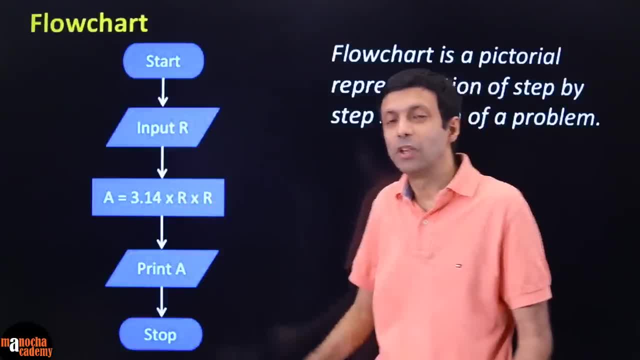 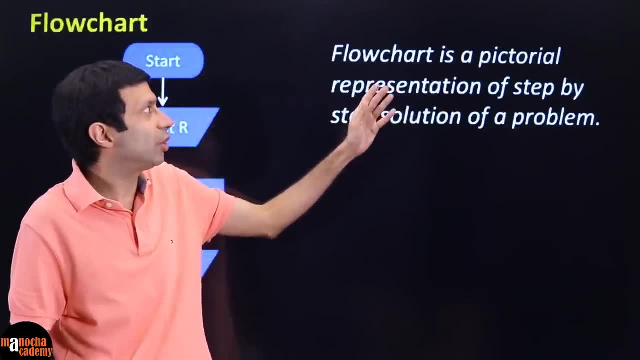 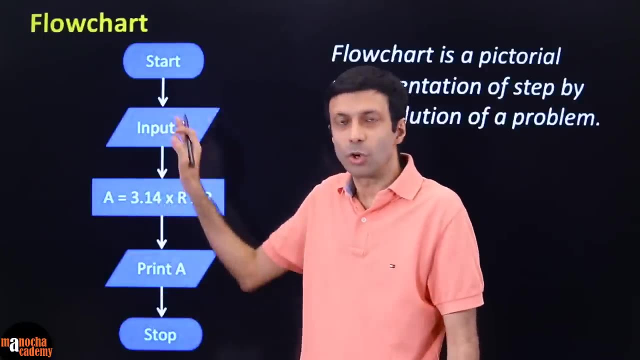 a chart where you can see the flow of the program. so what is the formal definition of flowchart? it is a pictorial. it is a pictorial representation of step-by-step solution of the problem. so pictorial means graphical, so you can see you're sort of drawing a picture of the steps, showing it like a 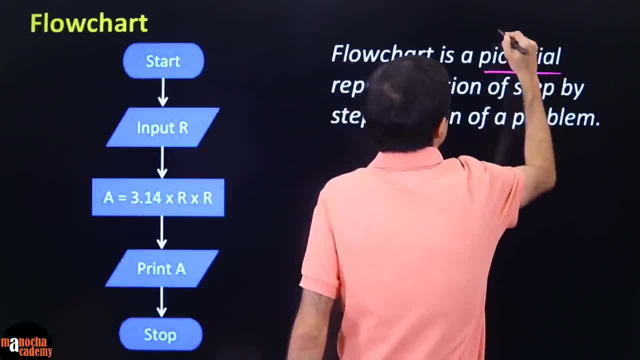 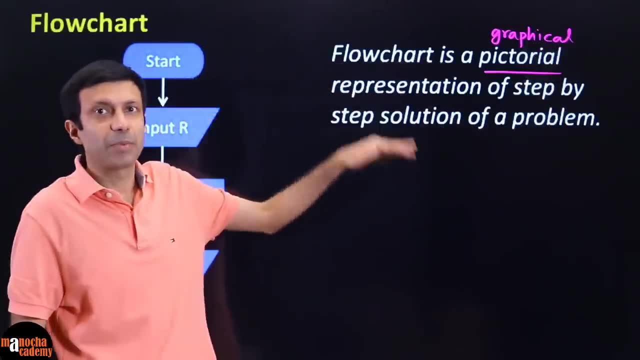 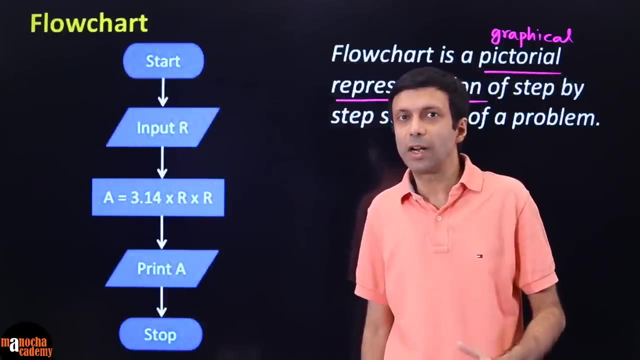 graph. so it is more of a kind of graphical representation or a pictorial representation of the step-by-step solution of the problem, and this is what we call as a flowchart. now, when you're writing a flowchart, there's one interesting thing: that you use different shapes or different kind of boxes. here you don't just 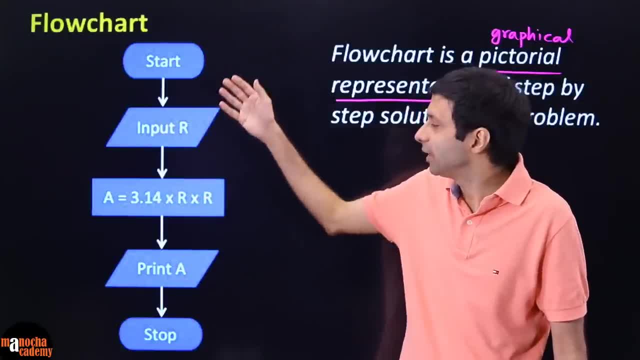 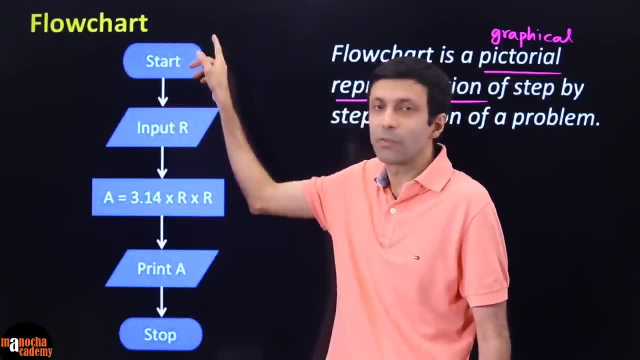 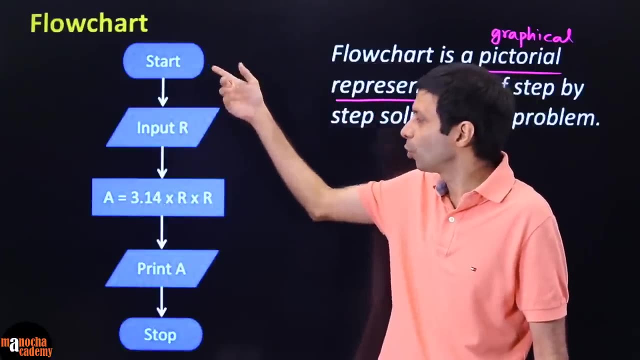 put everything into a rectangular box. you can see there are different kind of shapes here. for example, can you see the start and stop is kind of rectangular box but with kind of curves at the end, so it looks like an oval almost. so start and stop is there and this signifies the start of the program and the end of the program. stop then when you want. 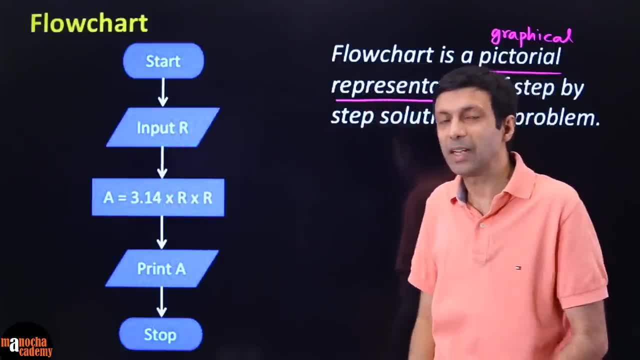 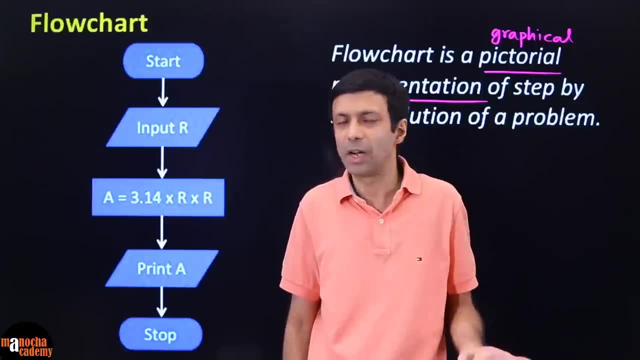 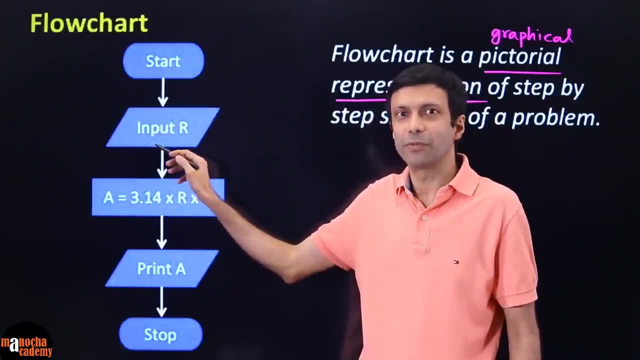 to whenever you want to take input. remember we said: for the computer to calculate the area you need to supply the radius. and let's say we are taking user input, what you have learned in Java or Python, you can take user input. so the input box we represent with this parallelogram kind of 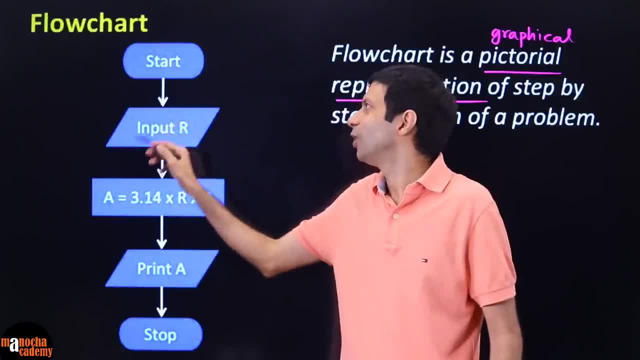 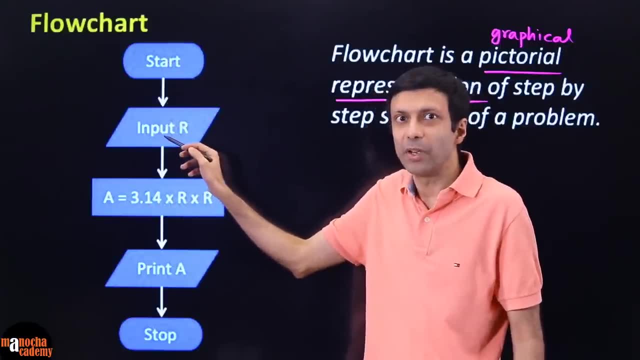 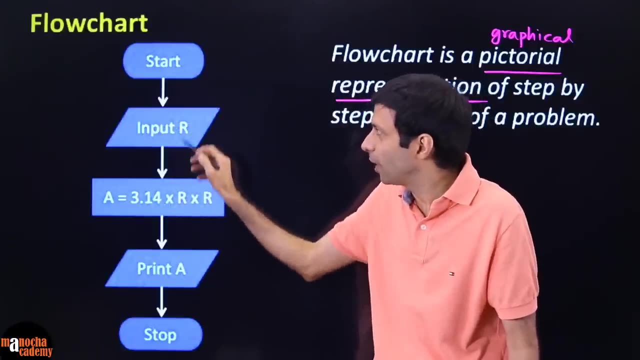 symbol. ok, we don't use a simple rectangle here, we use this parallelogram to input the radius. so you can see start. the first step is to input radius, because you cannot do first step area if you don't know the radius. how do you calculate the area then? so the next step, we represent, we draw this arrow. 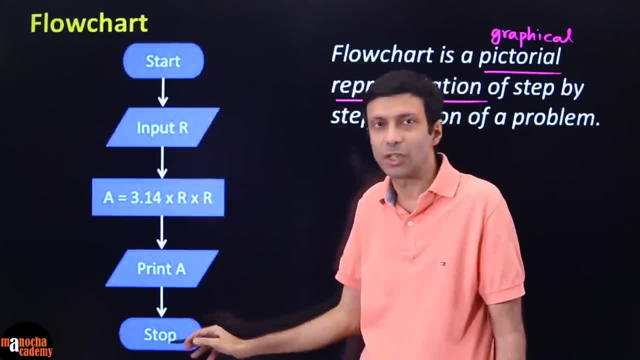 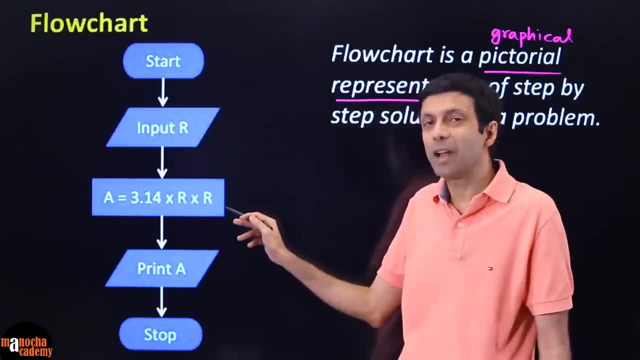 so the program is flowing like this, so you can clearly see the direction in which the program is going: area. so you put down the area, formula three, point one, four, multiplied by R, multiplied by by RC. now you're getting a little more computer specific, because computer may. 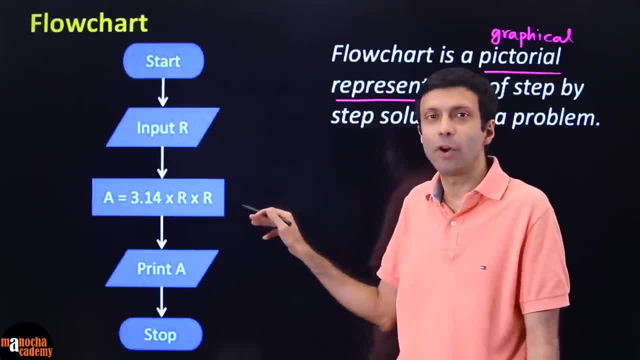 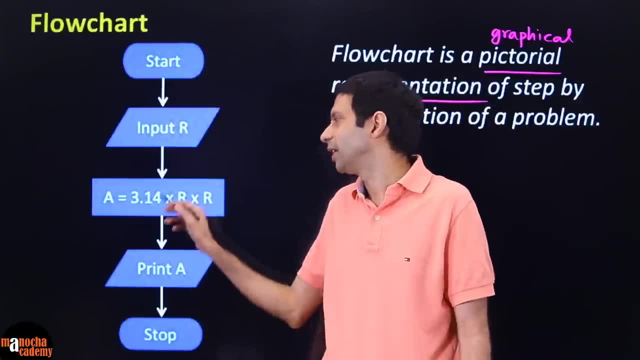 not know what is our square right. so you're writing the clear formula for the computer. so in these kind of things sometimes you keep the computer in mind. sometimes in the books you will say they are simply writing pi R, square in mathematical terms. so whatever convention is being followed in your 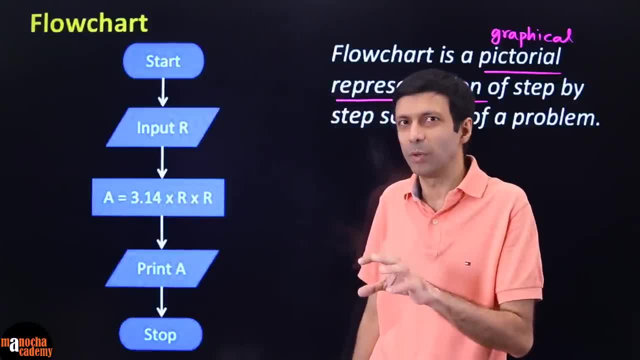 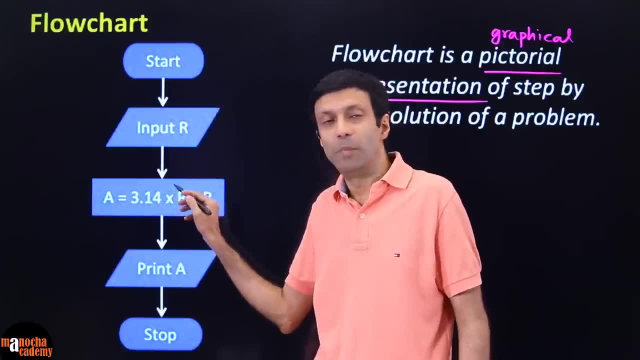 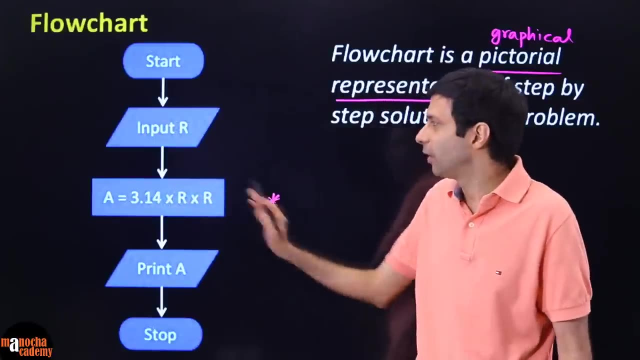 school or your book, but usually we try to write it close to the computer. here. sometimes you might want to use multiplication, because you know in computer the the multiplication is represented with the star symbol. but for here I have ignored that detail, we have just written it as a normal. 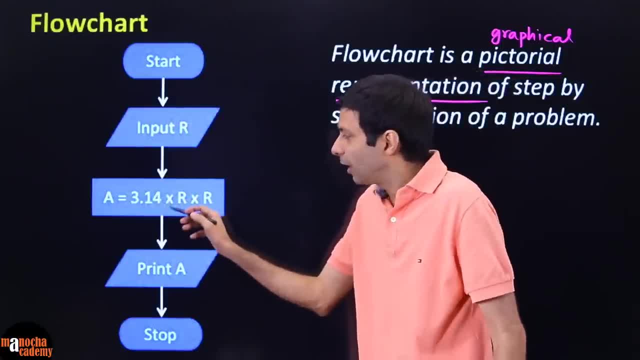 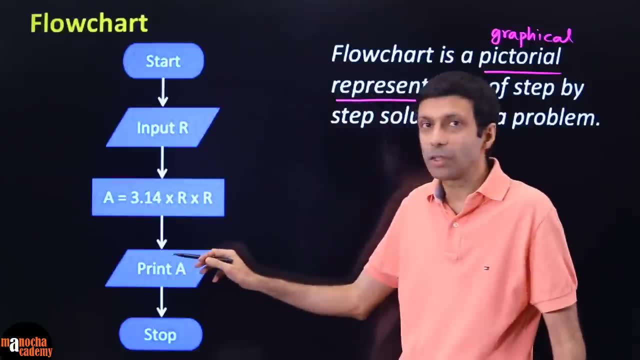 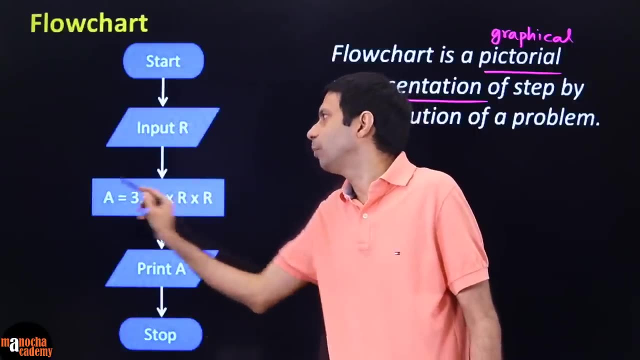 multiplication. so that's your area calculation, and then finally, you go to printing out, printing out the area. so can you see again, you have drawn a kind of parallelogram box, why? because this input and output are drawn, represented with this parallelogram, and any processing or any. 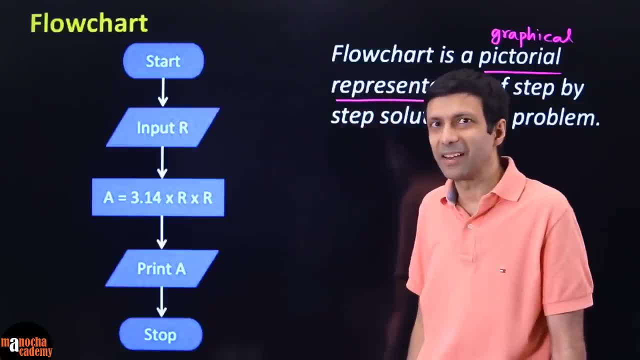 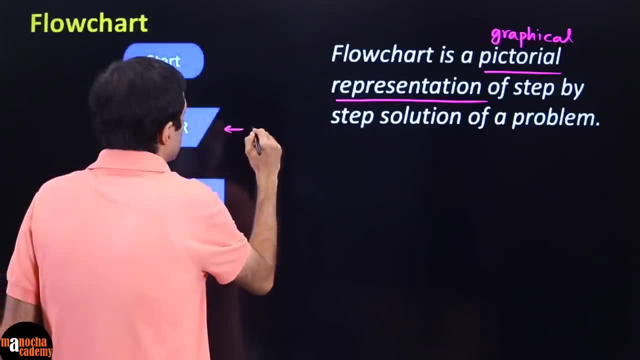 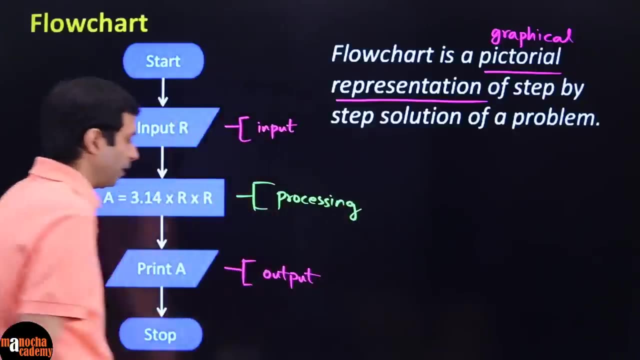 processing is represented with this parallelogram and any processing or any computation that happened represented with a rectangle. so clearly you can see. this is the input and output steps. so this is a input step, this is a output step and this is the processing step, and then, finally, you end up with the stop. 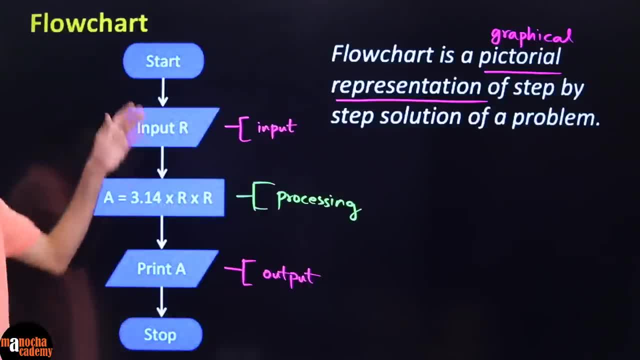 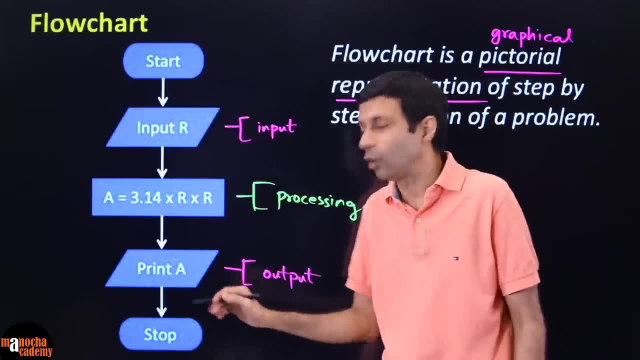 where you write stop. or sometimes you might see the word end here to show the end of the flowchart. so these are the standard flowchart shapes and symbols and when you're writing the flowchart, you're going to have to write the flowchart, you're going to have to write the. 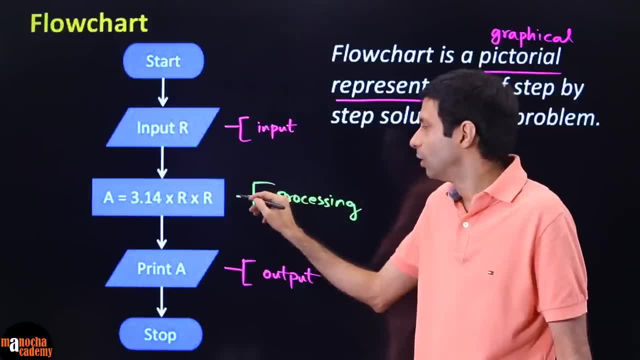 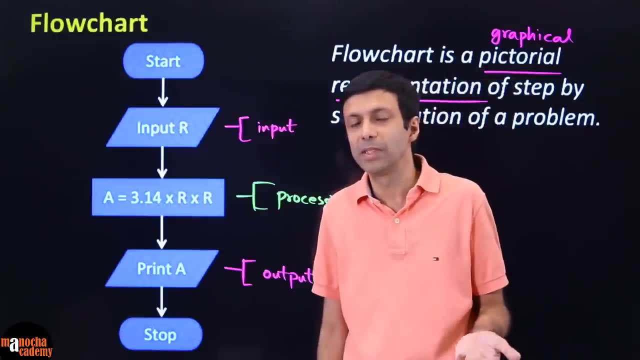 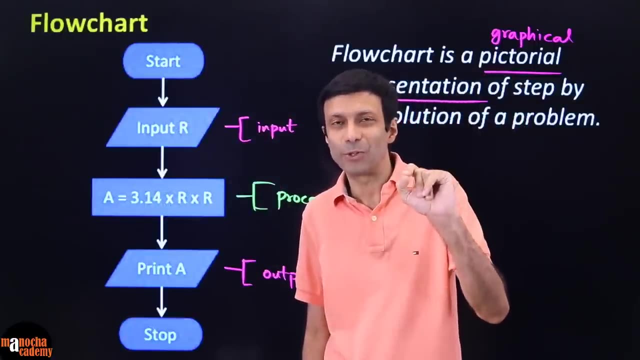 comments. you write this annotation with this kind of you know line and then this kind of bracket, so these are your annotation or comments. in the flowchart we look at some more symbols. these are usually standardized symbols. in fact, I pulled these symbols using the. there is a flow chart tab in PowerPoint also, so 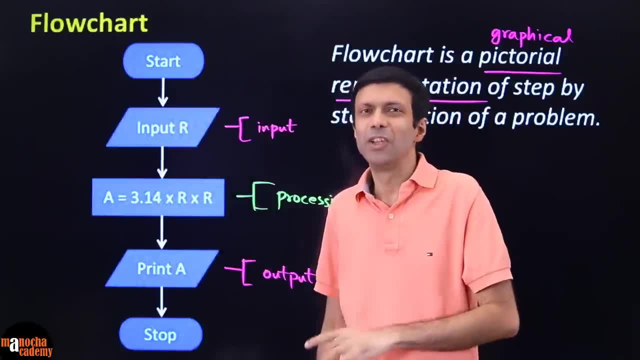 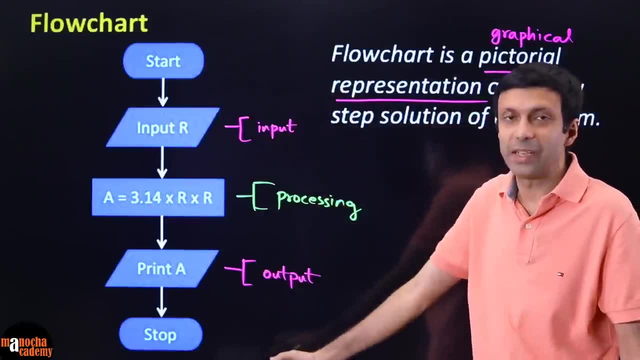 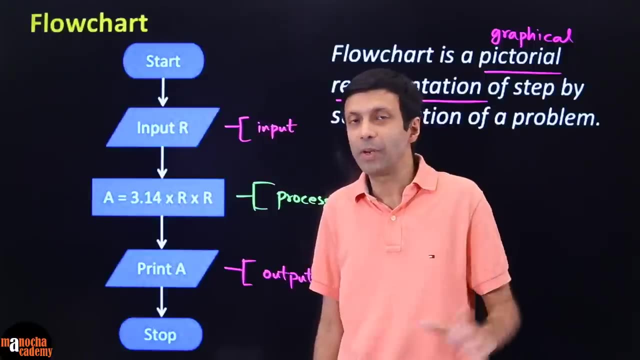 these have been drawn using powerpoints, flowchart shapes, so they are pretty much the industry standard today and, as you can see, it is a pictorial representation of the solution to your problem. this is how you write down the flowchart. flowcharts are very popular because it's very easy to read, very easy to understand the flow of logic, and it is one of 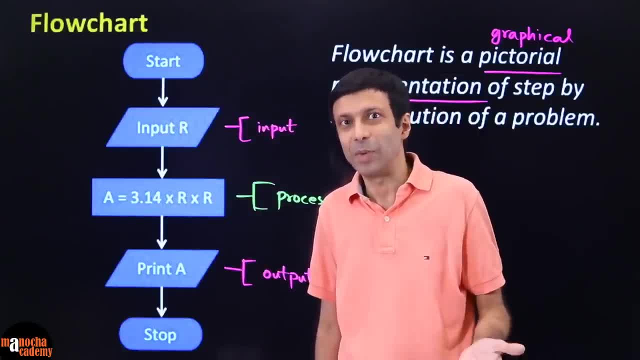 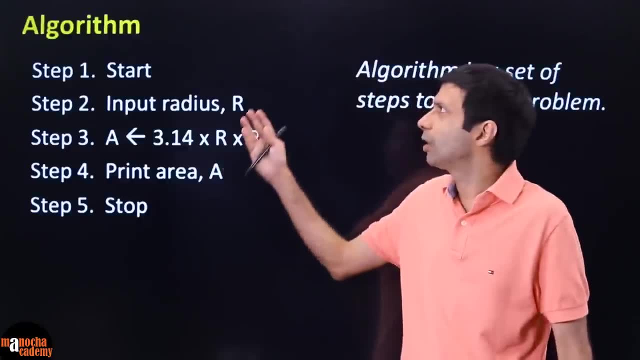 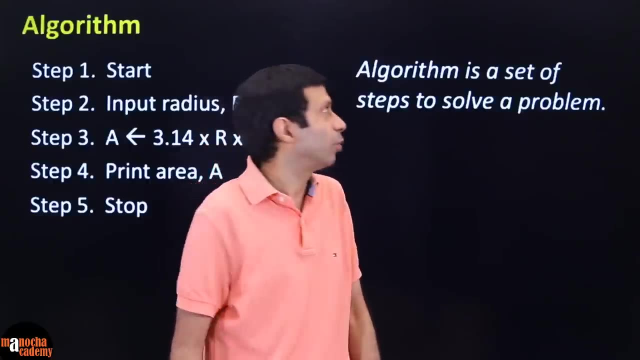 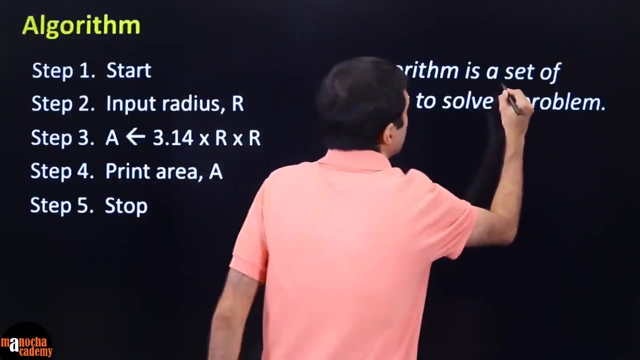 the most popular ways of representing a recipe or your logic, so we saw an introduction to flowchart. next let's look at what is an algorithm again. it's another way of representing your recipe or logic. so what is an algorithm? it is a set of steps to solve a problem, so algorithm is nothing. 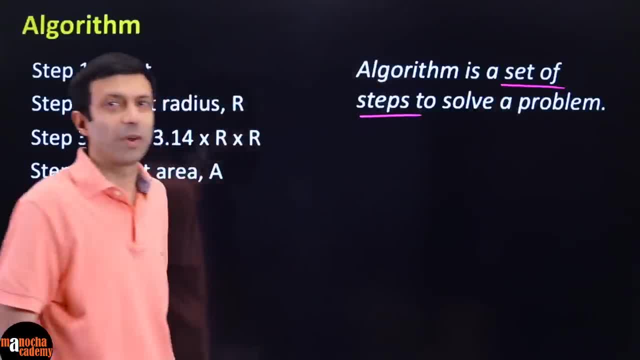 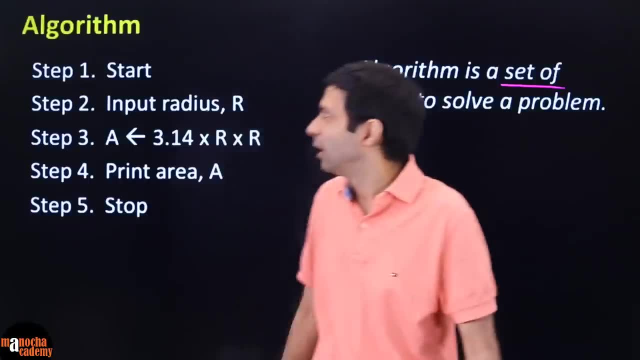 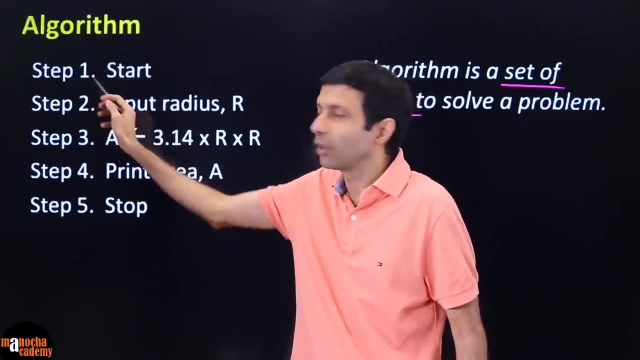 but a set of steps to solve your problem, just like we saw the algorithm for cooking the noodles right, step-by-step procedure. and here you listen down very clearly like one, two, three, four, five, just like recipe steps. you can just write one, two, three, four, five, or you can write the word step, one, step. 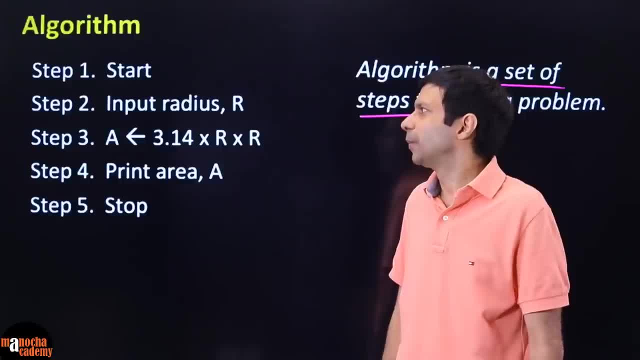 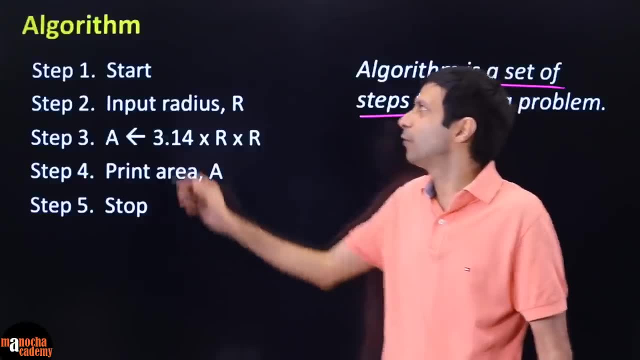 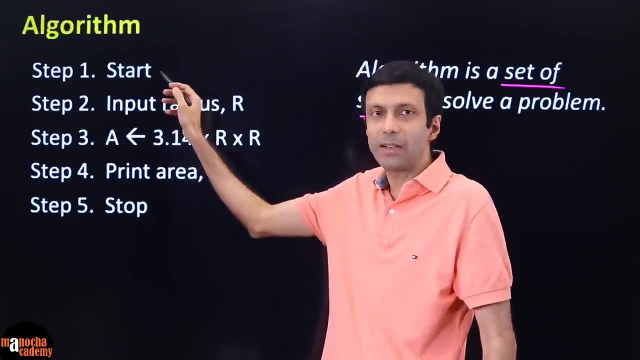 two, step three: whatever convention you are following, these are not written in stone. you know you might change your, you might see changes in styles in different books. so what is the first step? again like a flowchart. so this one is not pictorial, it's more like a step-by-step statements so you can see start and the ending one is a stop, then 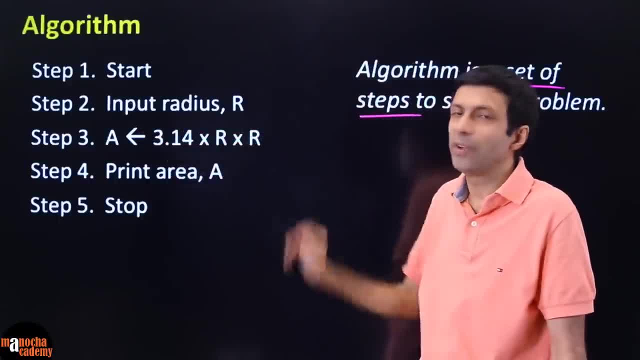 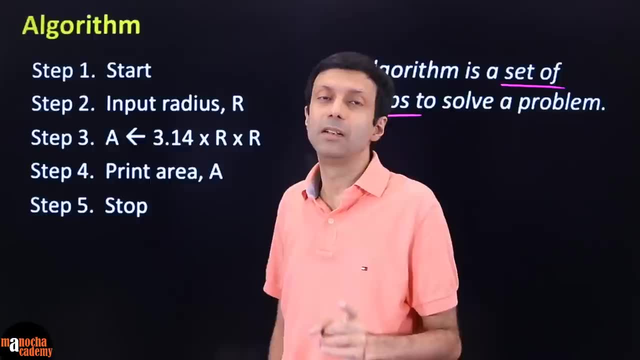 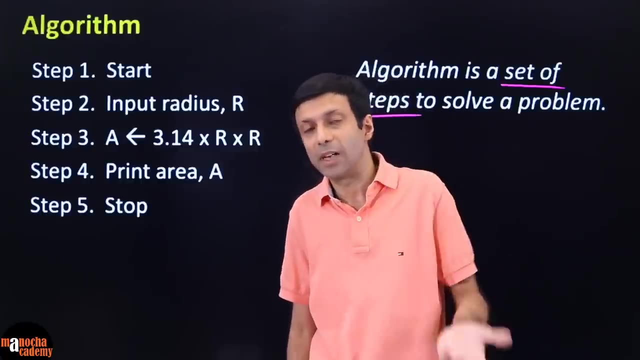 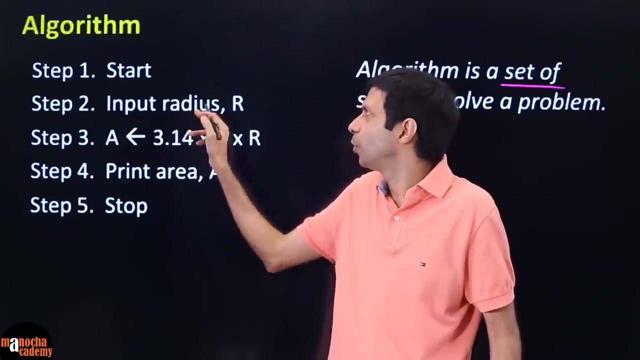 what do you have? you say input radius and you give your variable name here comma R. so this is more a input statement. so, like in Python, the input could be different. in Java you use scanner, in a C++, you use C in, so we are not bothered about that. we are writing it in simple English: input radius. 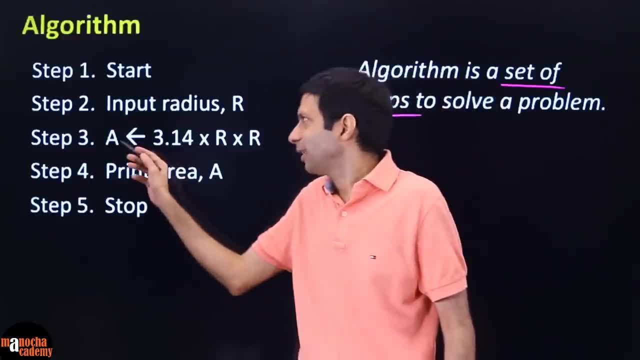 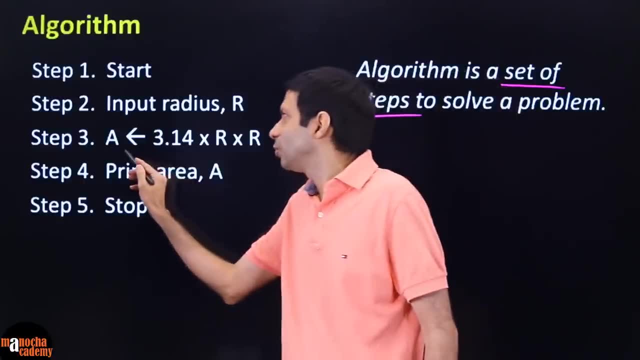 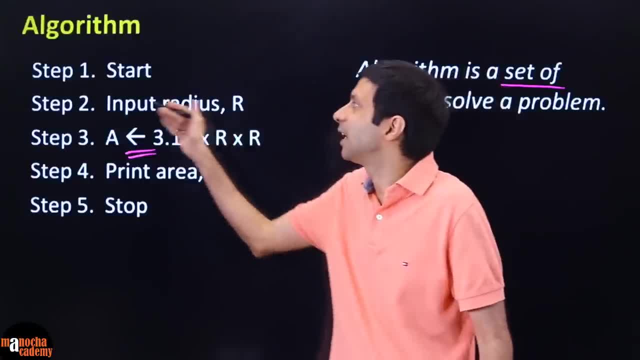 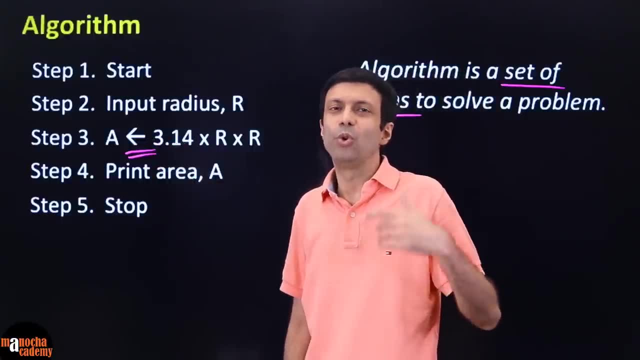 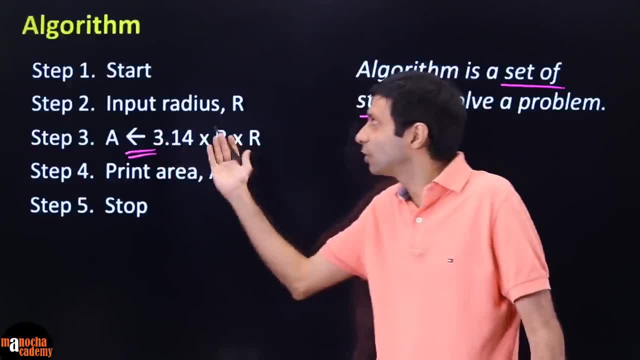 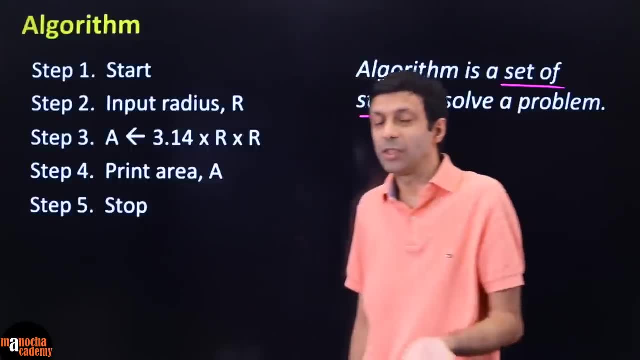 but usually the arrow symbol is popular and the arrow is from right to left. okay, and then you go ahead and print out the area, otherwise the user won't be able to see the output. so you can say print area and your variable name a. so you can see all the variable names are clearly mentioned. 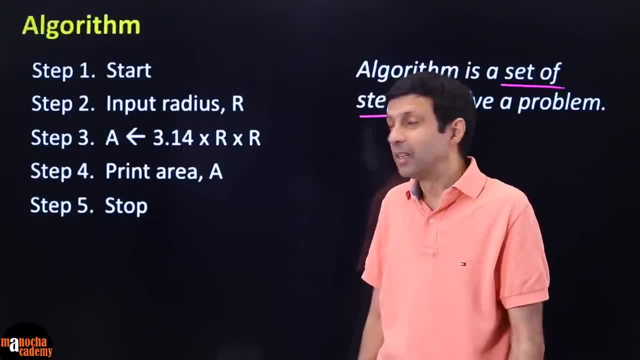 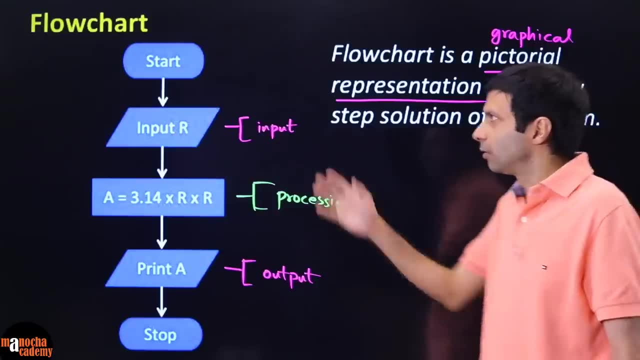 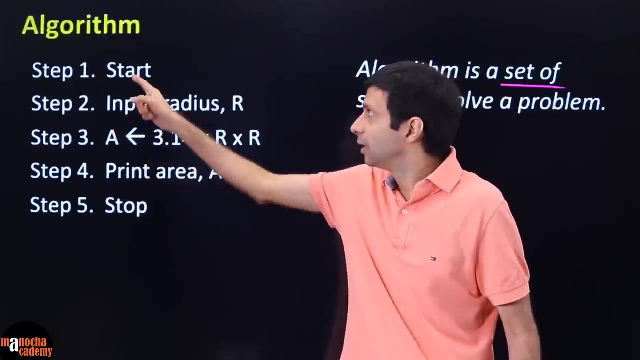 and then you stop. okay, sometimes this arrow symbol is also used in flowcharts, so you can see it's very similar to a flowchart, very, very similar. the main differences are: we don't draw diagram, we just write it in terms of clear steps. steps have to be numbered- very important, because you might 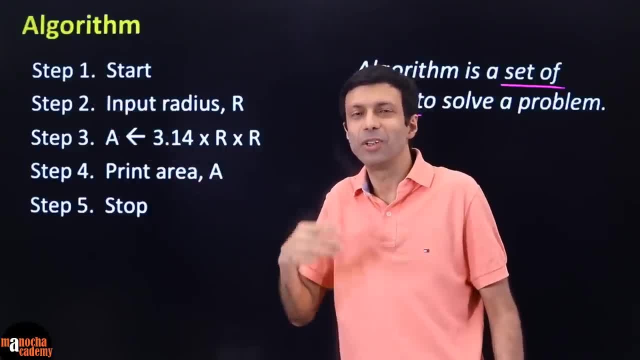 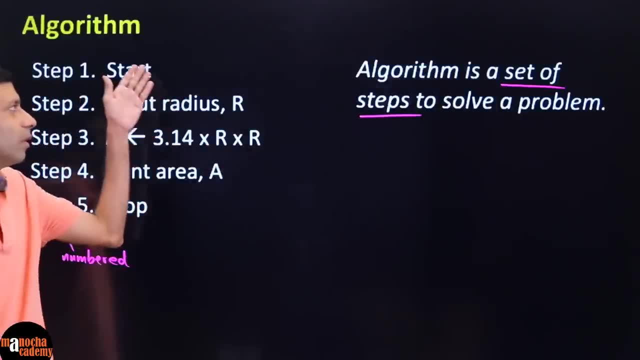 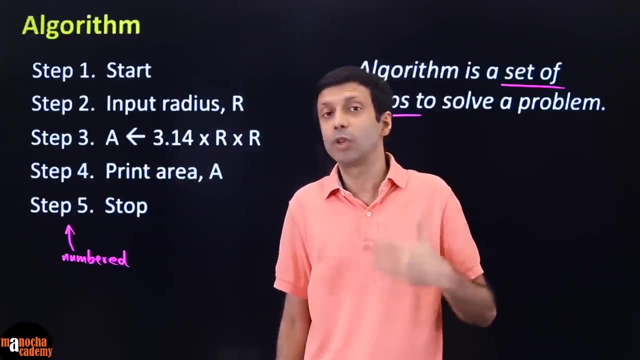 say: now go to step 3, just like in a recipe. you know, sometimes they say: go back to step 2. so step numbering is very important. and then you write it in very simple English. you are not writing the actual code like python or Java, because maybe your friend does. let's say, you know python, but your friend knows Java, so we want. 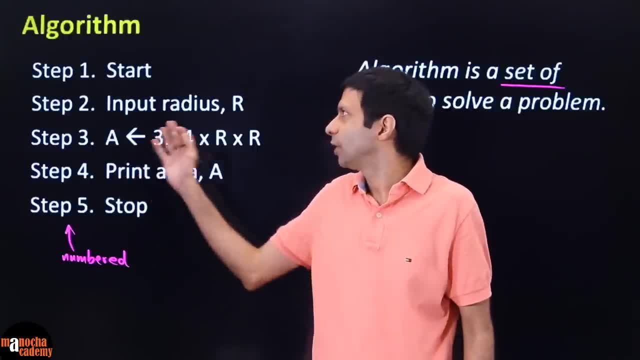 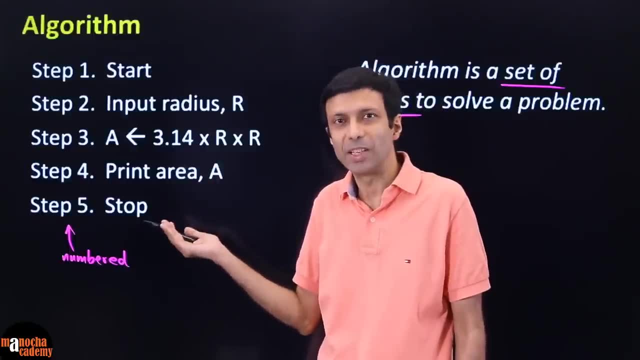 to write it in a simple, friendly, neutral way. so that's why you write it in these kind of sentences and this kind of arrow, and some conventions are used, and you clearly mention your variable names. so is this simple algorithm clear to you? so we have looked at flowcharts and algorithms. 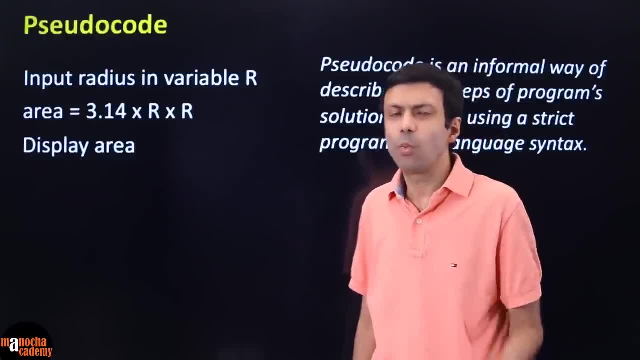 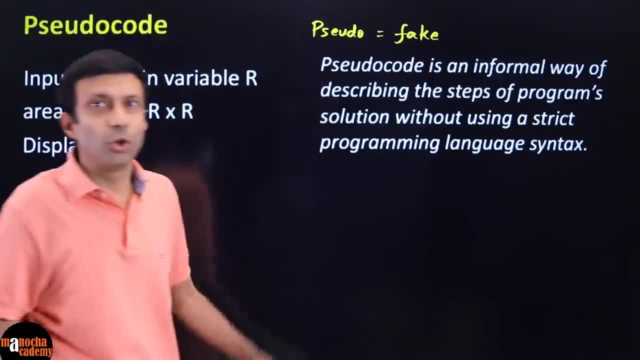 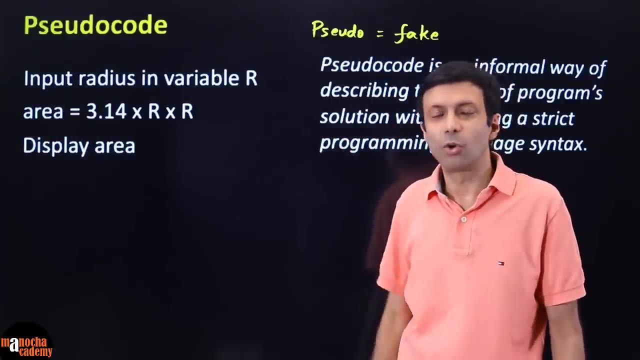 next let's look at pseudo code. what does the word pseudo mean to you? do you guys know the meaning of the word pseudo? the word pseudo means fake or false, right? so this is like fake code, almost like you know, not the real code. but the advantage is it looks very similar to code, so we can easily 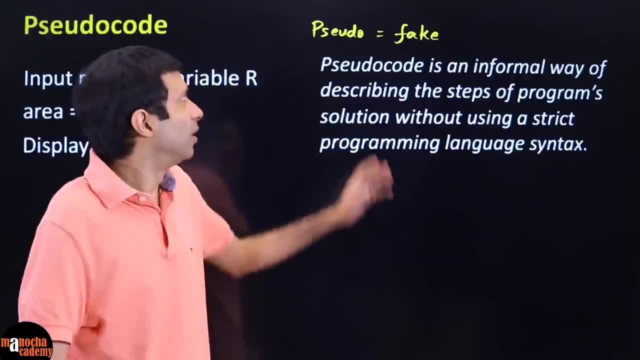 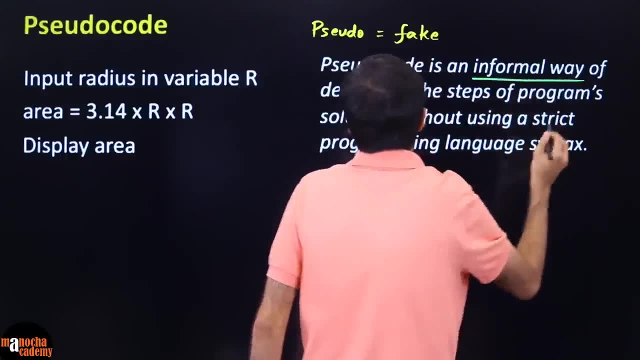 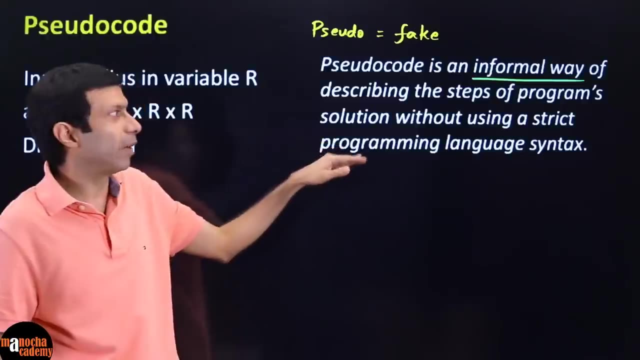 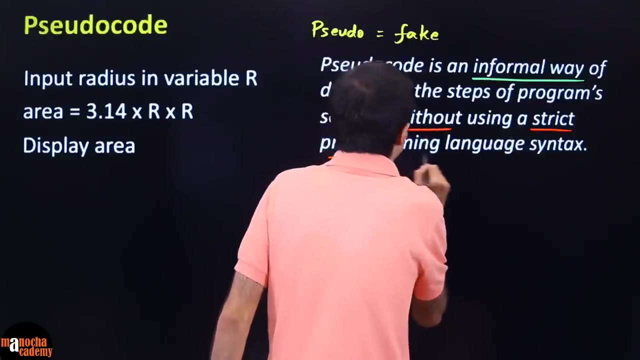 translate it to another language. so what exactly is pseudo code? pseudo code is an informal way- see the keyword here. it is an informal way- of describing the steps of a program solution without using a strict programming language syntax. so it says: without using a strict programming language syntax. what does this statement mean? so you're not writing real code. 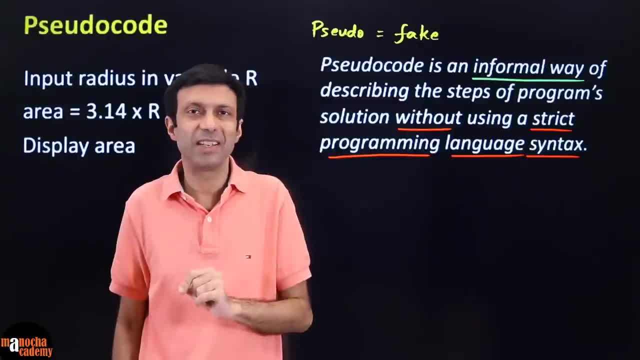 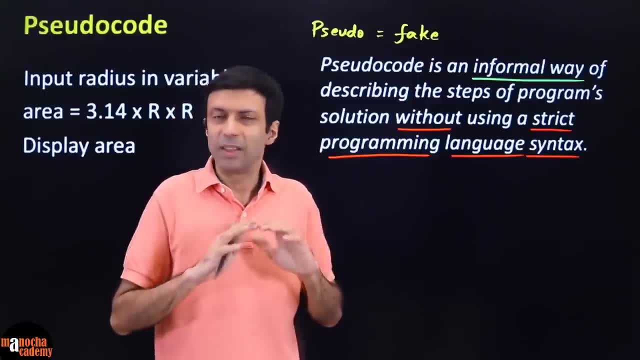 because real code, you know, is very, very. it has a very strict syntax. if you are writing Python or Java code, you have to write it perfectly correctly, otherwise the compiler will give an error. but this is not like that. this is just writing. this is like. pseudo code is more like. 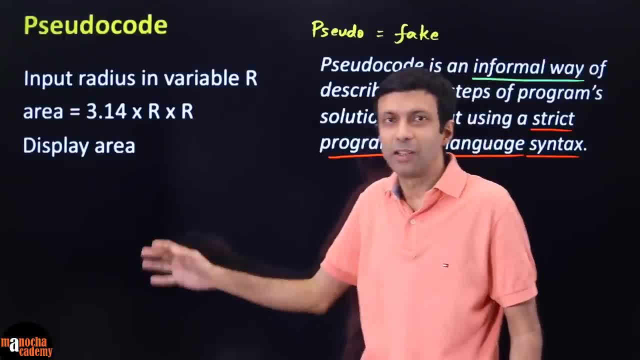 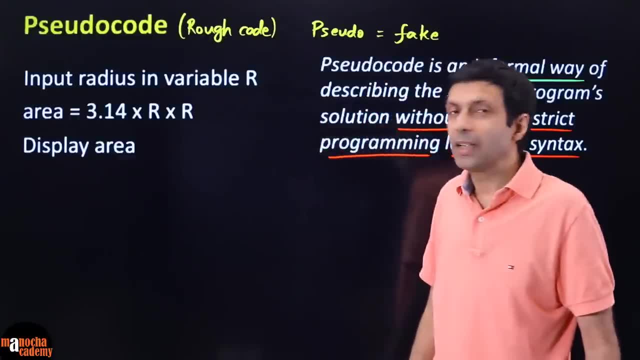 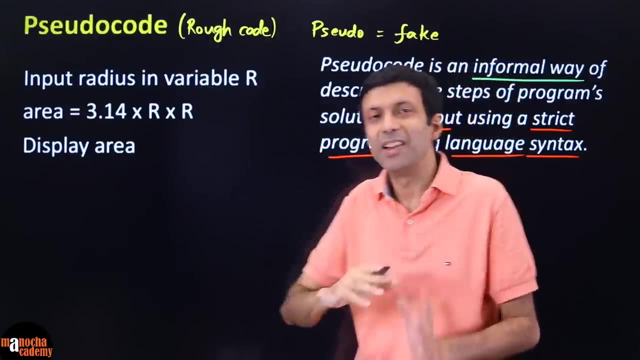 rough code. okay, so you're just writing it roughly so we can say pseudo code is like rough code. you're just writing it informally. the advantage is that you can quickly write it down like you know rough code and then translate it once you're satisfied with your logic. now you write the actual. 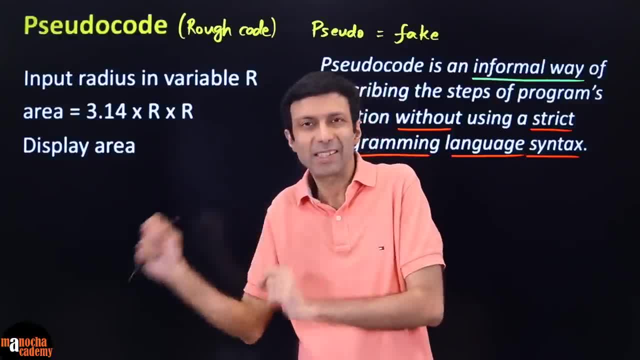 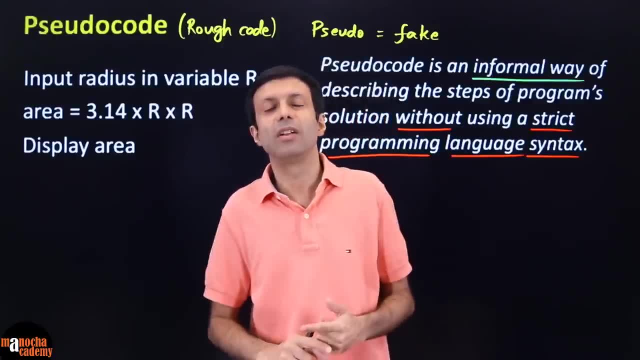 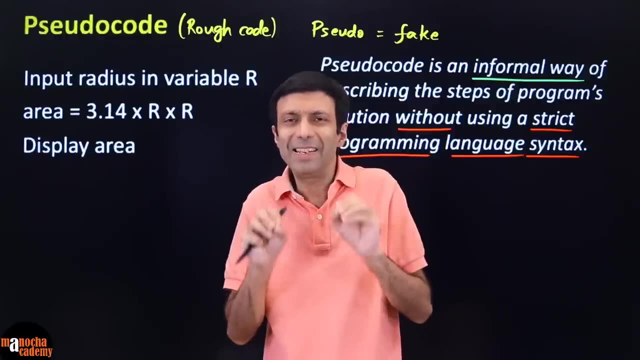 code and that will save you time, because you are not wasting time thinking about the syntax and details of the language. your focus is on the logic. so that is the whole importance of this class: that when you are learning flow chart algorithm pseudo code, your focus is on the logic and not the details. 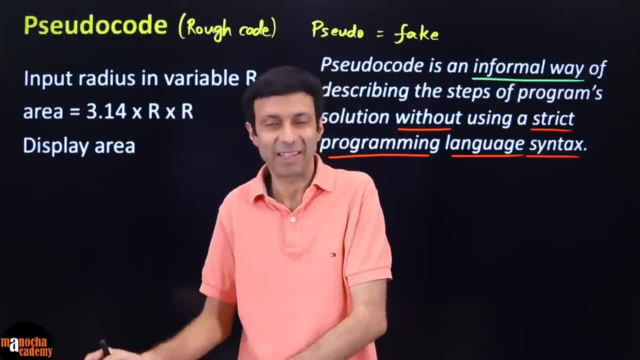 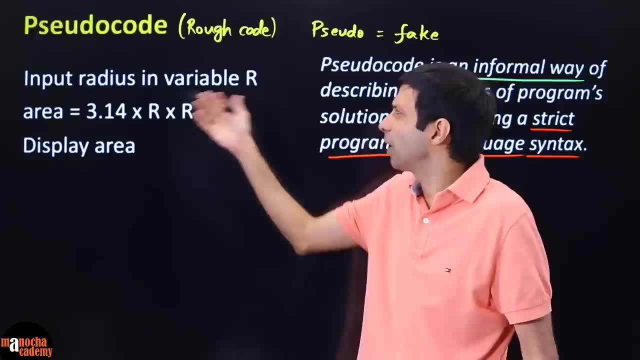 and nitty gritties of the language. okay, that comes next. you are in the planning stage, right? so same way. here you are saying input radius in variable R. okay, this is one way of writing. you may use different ways. sometimes they'll just say input radius, comma R or invariable R, whatever style. 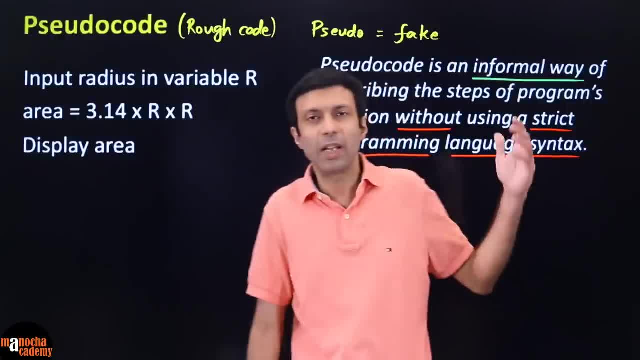 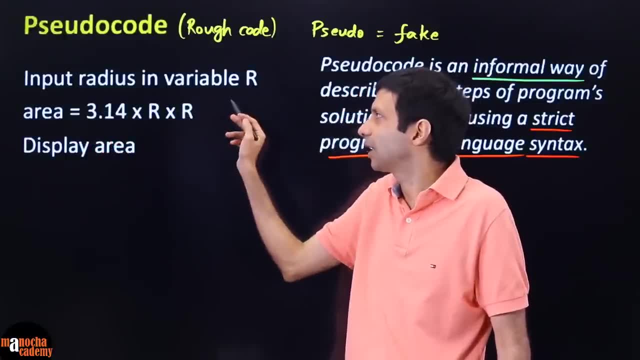 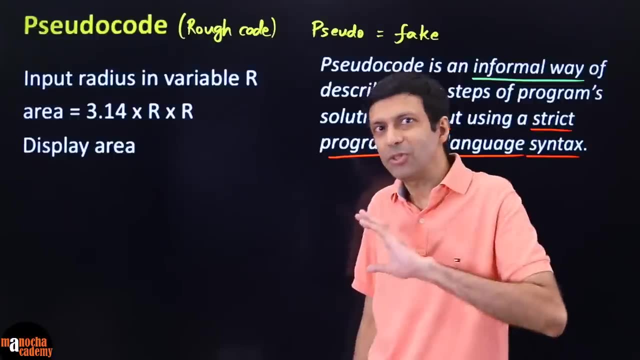 you're seeing there are different styles of writing pseudo code, because it's all informal, there's no right or wrong way. similarly, you can say: area equals 3.1, 3.14 times R times R. so you have clarified your calculating area. or you can maybe just write capital, A display area, so can. 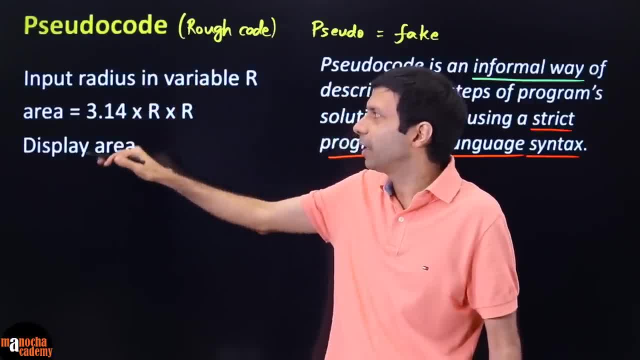 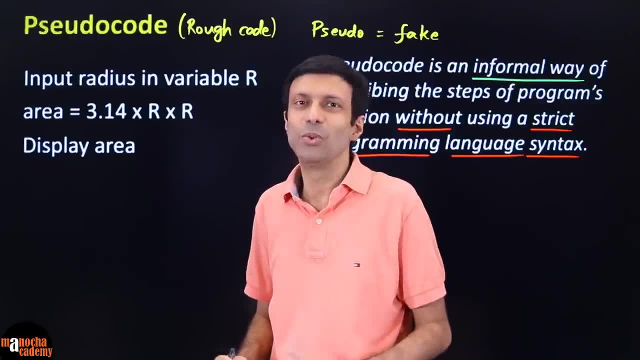 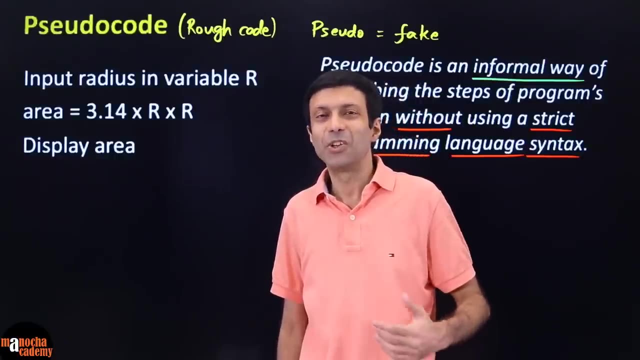 you see, the logic is very clear that we are doing input, calculation of area and display. this is called pseudo code. so are all the three styles clear to you: flow chart, algorithm and pseudocode. we'll, of course, look at some more examples to really understand these concepts, but the whole goal. 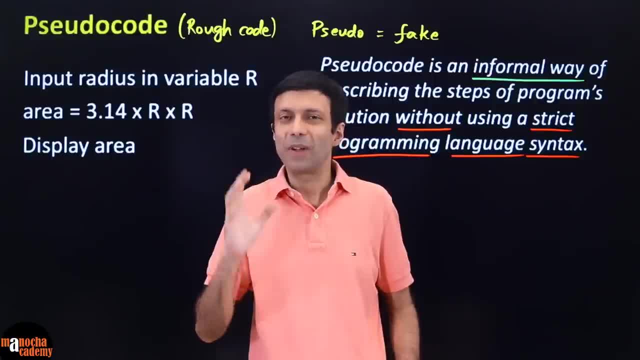 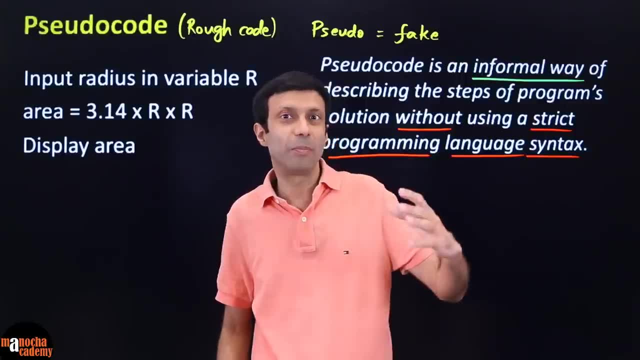 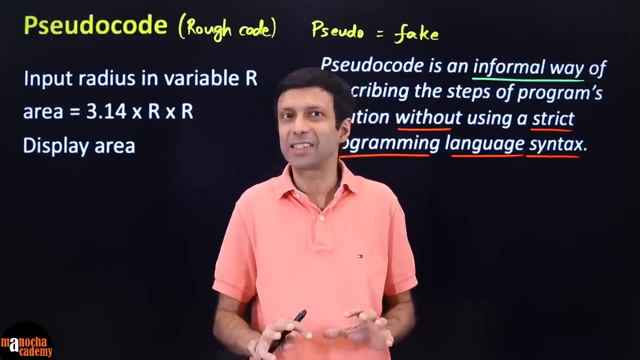 is to plan out your logic, to brainstorm and decide your logic, and especially if the program is complicated. so you do this, and this is what professional programmers do. they plan it out using either flow chart algorithm or pseudocode. then they go to the actual coding, because actual coding takes time. it needs to be perfectly right, but before that, 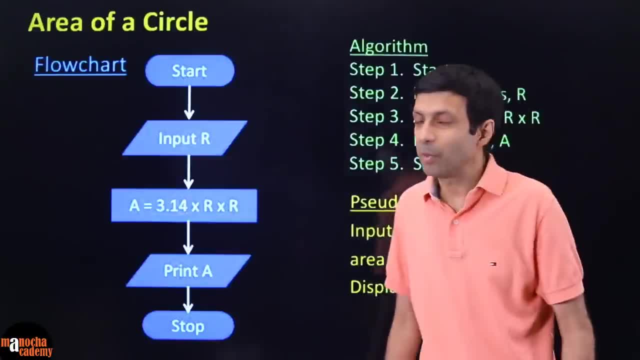 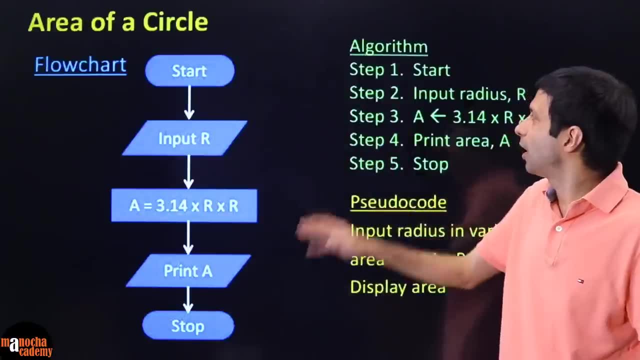 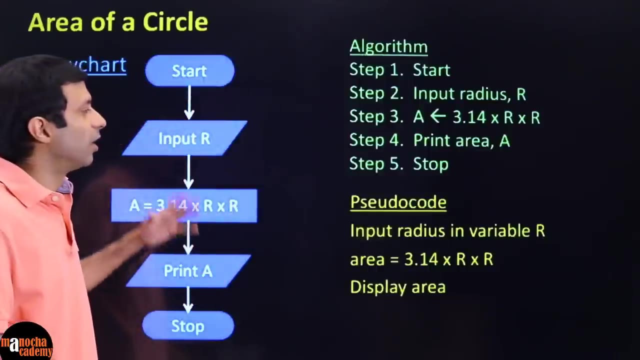 your logic needs to be right. so, in summary, this is what we have learned: that using the example of area of a circle, you could use flow chart algorithm or pseudocode. so I put them all in one slide for you to see that the whole goal here is to represent the logic. so what we are trying to show here, 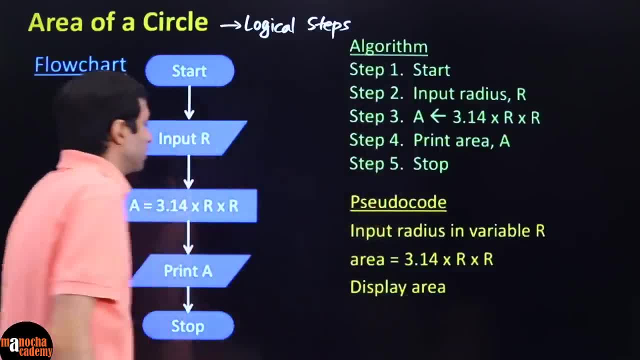 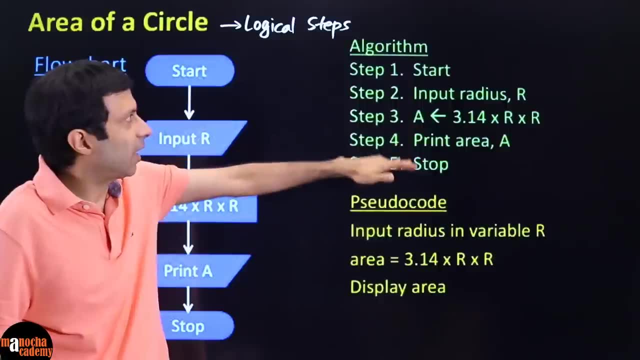 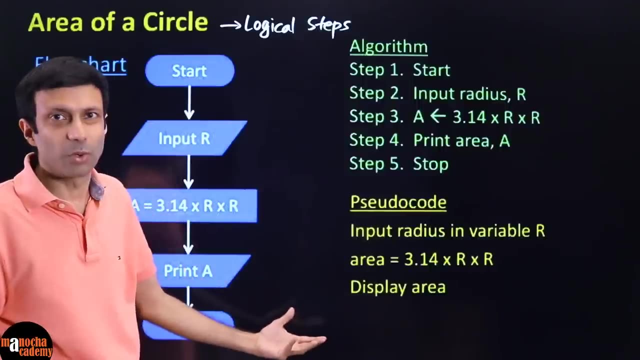 is the logical. so flow chart, as you can see, is a pictorial kind of representation. you could write an algorithm which again has start- stop, but you're writing it in a stepwise fashion and pseudocode is like your rough, informal code. so sometimes your school will teach you all these different styles, or 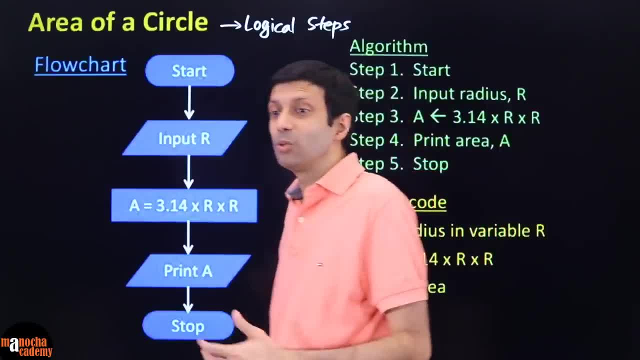 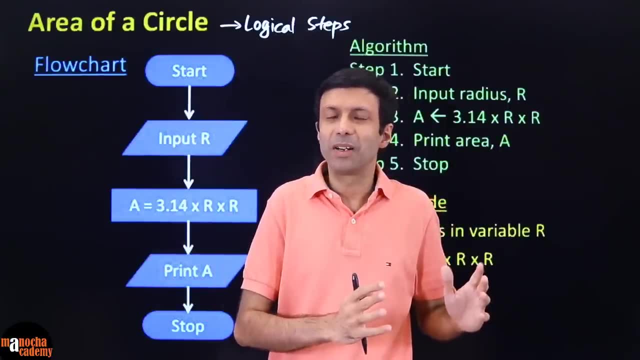 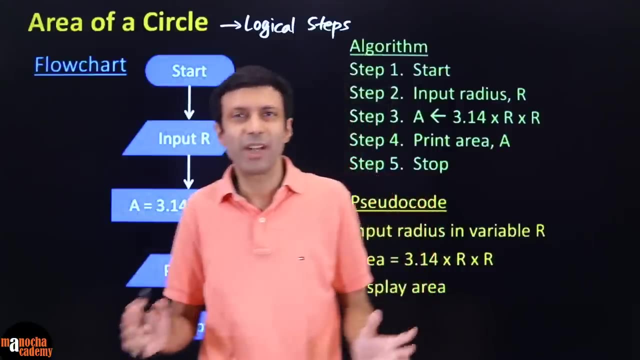 sometimes you might be following one style many times, you know. sometimes people find it easier to first draw the flow chart then write the code. sometimes even some people find it easier to first start off with the code and then start thinking of the flow chart, then again come back to the code. so there's no perfect right or wrong way. it is what style you. 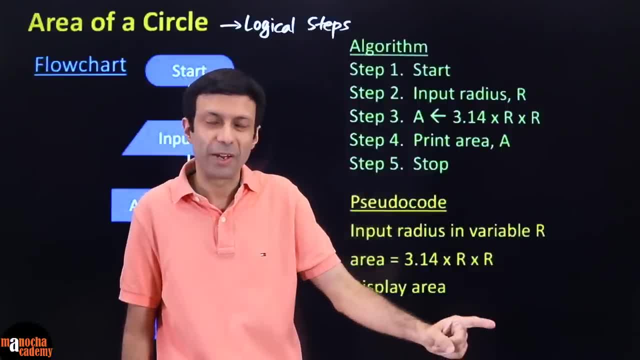 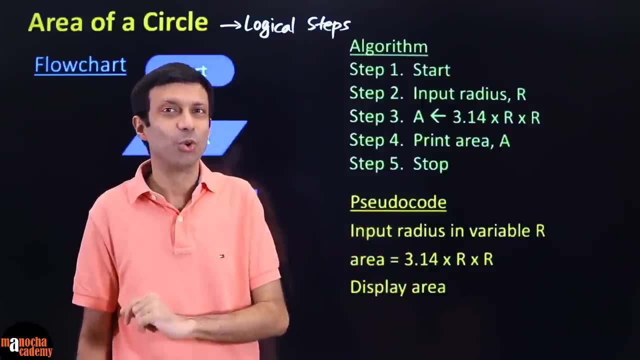 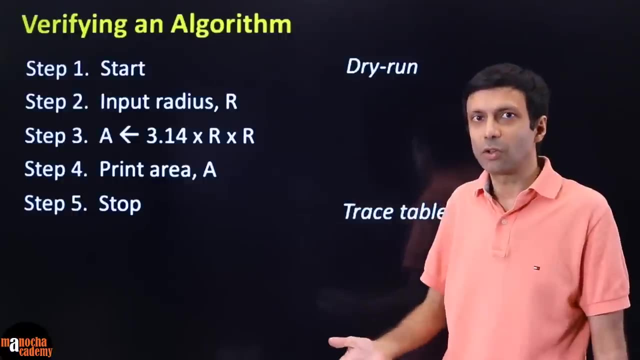 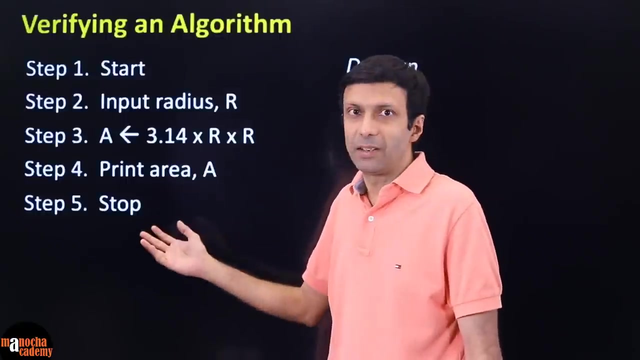 like, but always they recommend that do not jump to coding first. do the planning on paper first, or at least in your mind, before you go to code. another very important aspect is verifying your algorithm, or your flow chart or your pseudocode. what does this mean? so let's say you have written an algorithm. now you may think that it's right and you'll say: okay, I've. 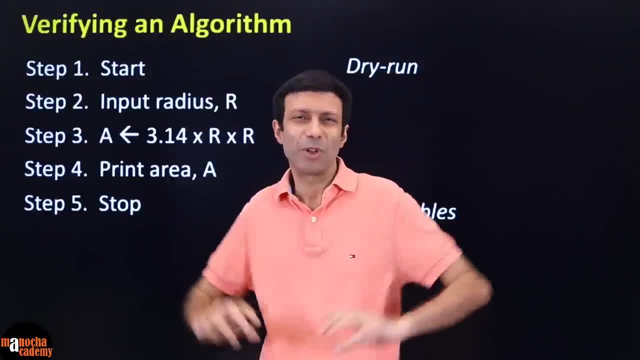 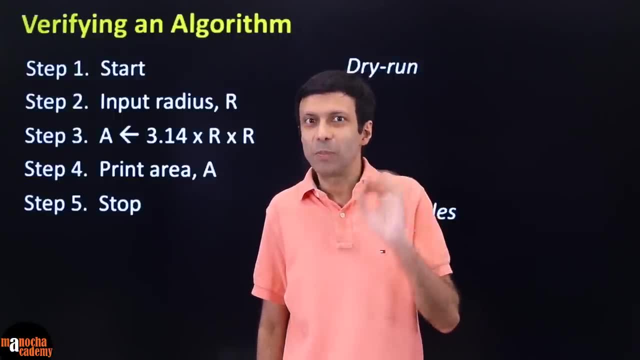 written my algorithm. now let's go to the computer and start coding, because we all love to code, right? we want to get our hands on the keyboard and write the code, but wait, there is a smart way to first verify your algorithm on pen and paper, using pen and paper, and then code. so this is what we call as. 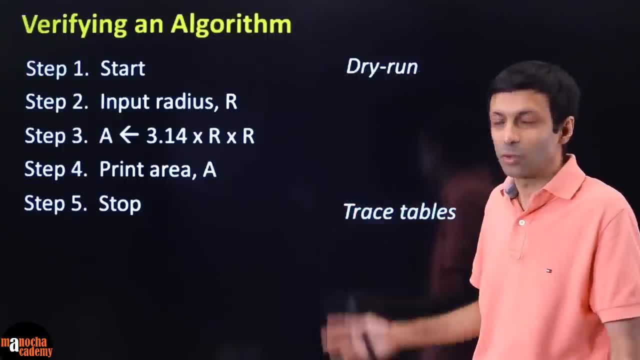 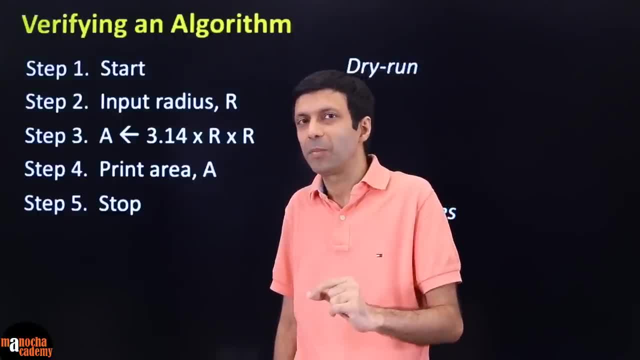 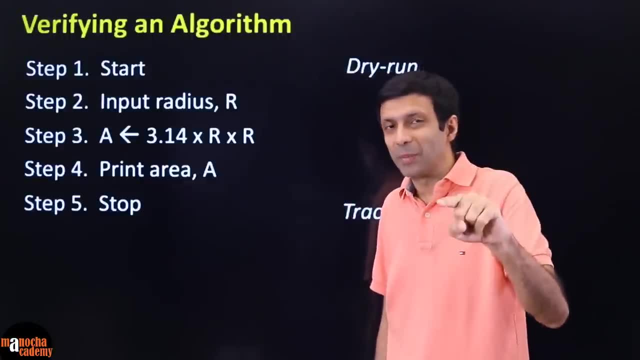 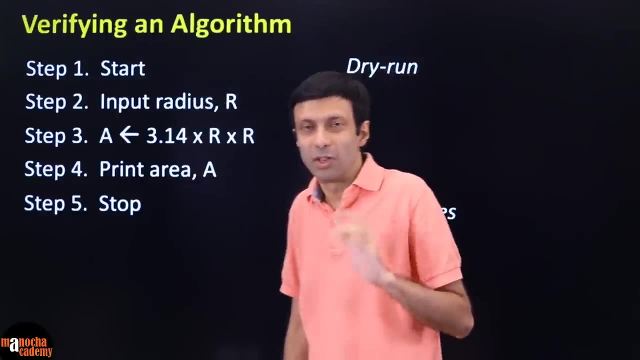 you have written, you are doing a check of it on pen and paper before you write the actual code. so how do we do that? very simple, you become the computer now and go step by step in the algorithm and check if you're getting the desired output. so, for example, let's start with step 1. so step 1 is simple, start. then we 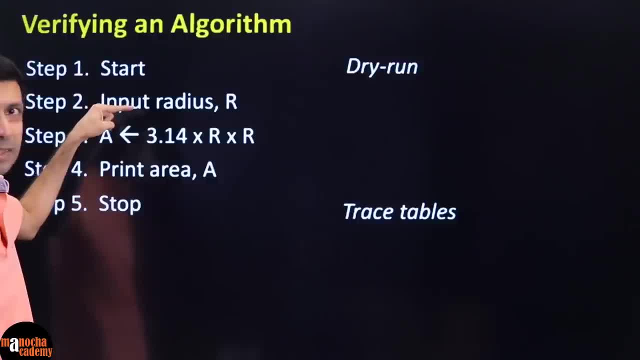 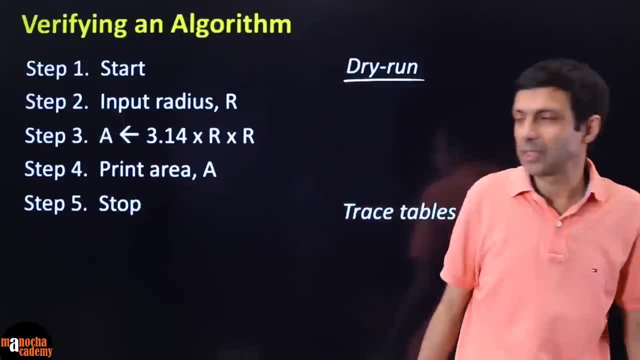 say: let's input the radius, so step 1 is simple start. then we say: let's input the radius, so you keep your finger here, you're in step two and in the dry run we will say: we are going to input the radius. so let's take some example. let's say the radius is 10, okay, so we have. 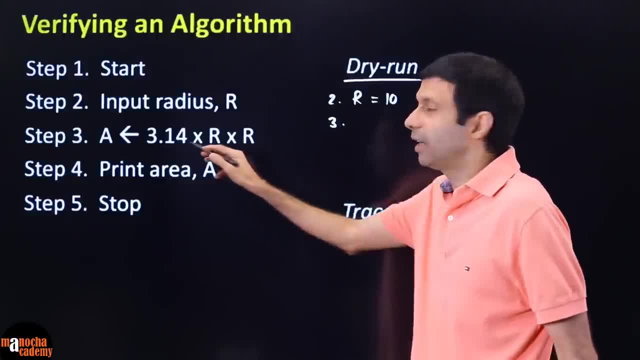 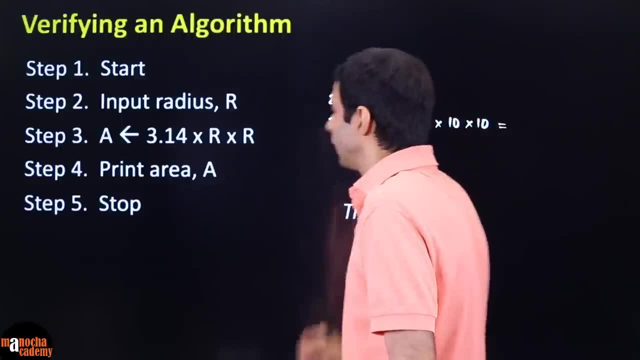 come to step 2 here. then step 3 area is 3.14 X 10x10?. so what is this going to be equal to? 314? value? what is this i was putting down to be in my mind to annexjis: area is 3.14 x, 10 x, 10 x x isn't there To get this. we have come here and this level of where the point is that if you get a mark on x 2 in order to get an Я HELP, than the area you are going to get from here when you going to. 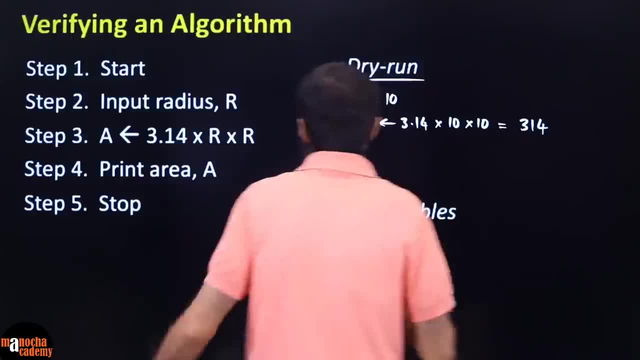 cancel it, crisp this example, anything that will matter later. but if you have written the opera D B, then follow the training. you will receive the errors done, this algorithm, then the next step, step number four. so please go step wise. we have finished step 3. we are going to step 4 here now. 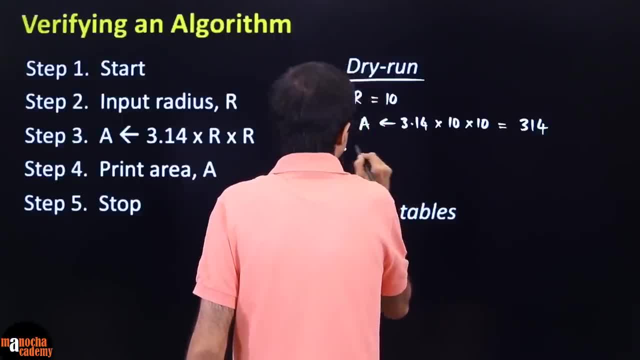 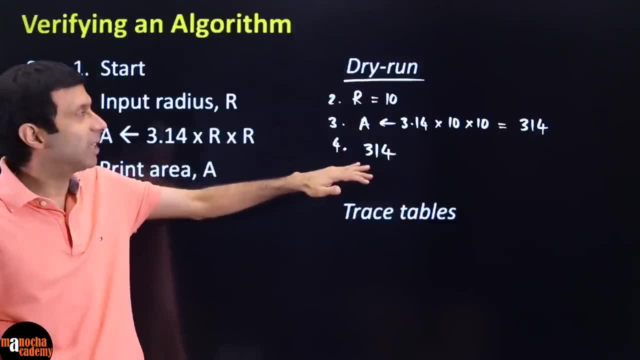 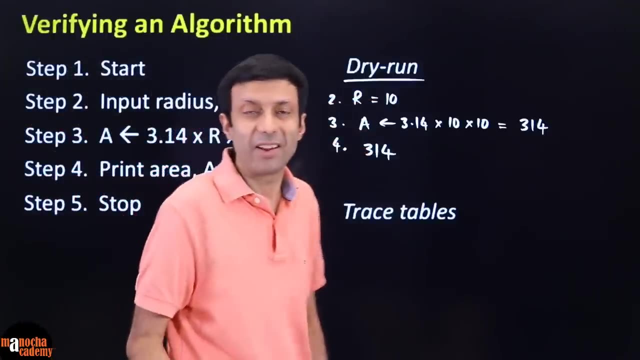 step 4 is to print the area. so the computer is going to print 314 here and then we stop. so can you see the program is working exactly as we expected. let's say, we input 10, it calculated the correct area and printed it out. so this is known as dry run, doing it on. 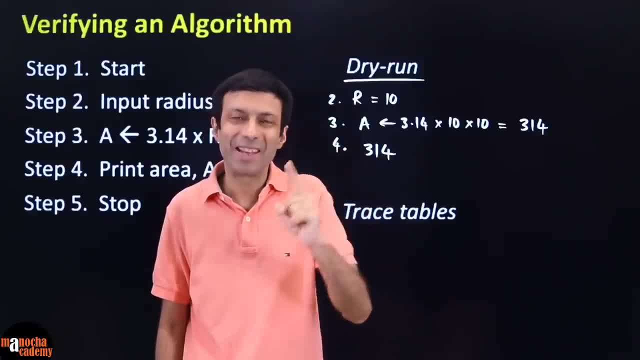 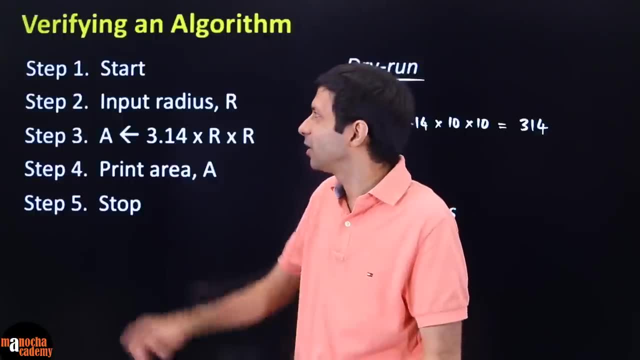 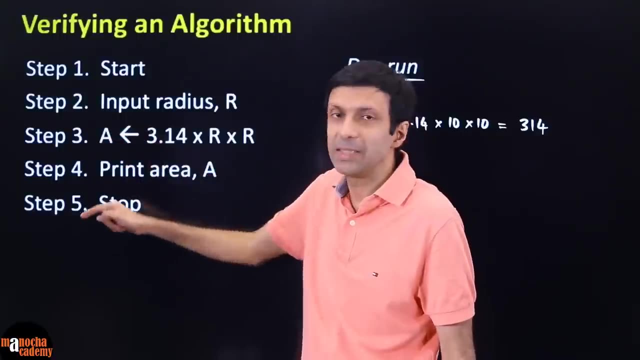 pen and paper without the computer. here your brain is the computer. so this kind of procedure is called dry run, and the important thing in dry run is make sure you keep your finger, or you keep ticking as you're doing these steps, so you keep going step by step, so that you do not miss out any single step. 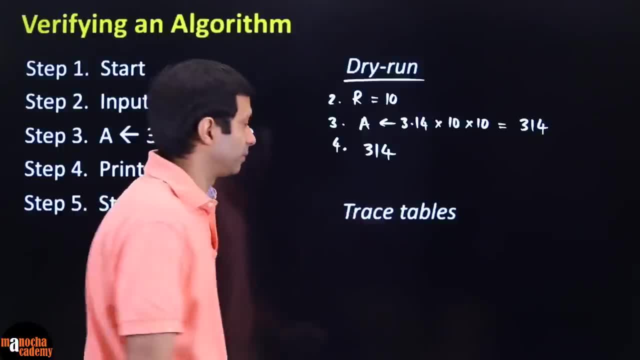 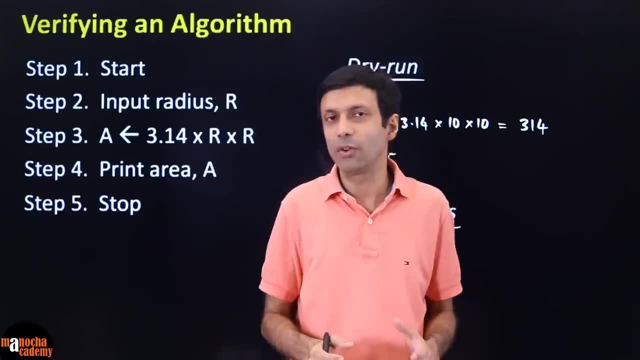 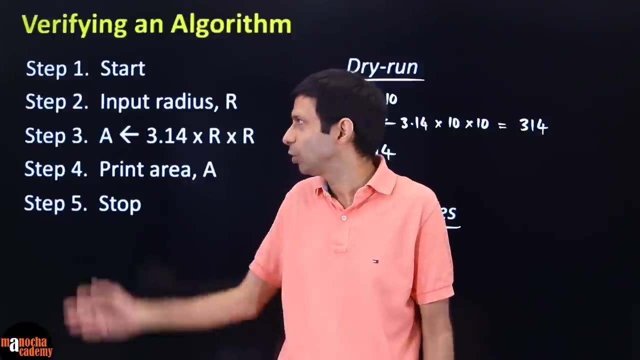 another way is using trace tables. what are trace tables? trace tables are basically, you know, rep, while you're running the program or while you're doing a run on pen and paper, seeing how the values of the variables are changing. because you can see, the important thing are the variables: radius. 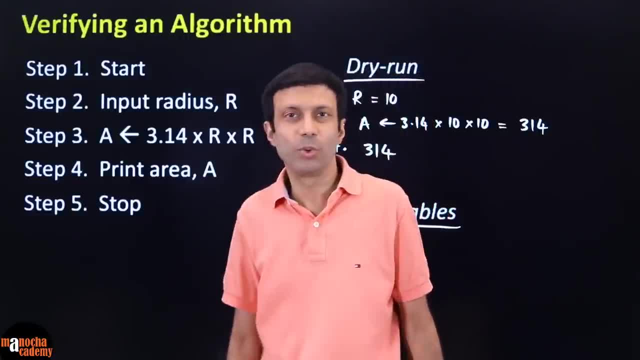 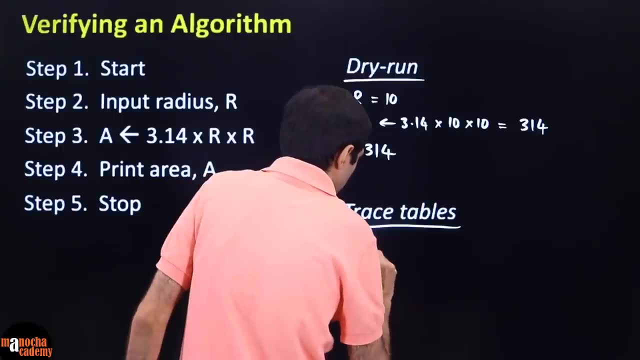 then area: these are the important things, right? so what will you do here? so again, you do start. you come to your first, second step, which is input radius. so you can see that variable and you can say value. so your variable is r. you've created a variable like this: 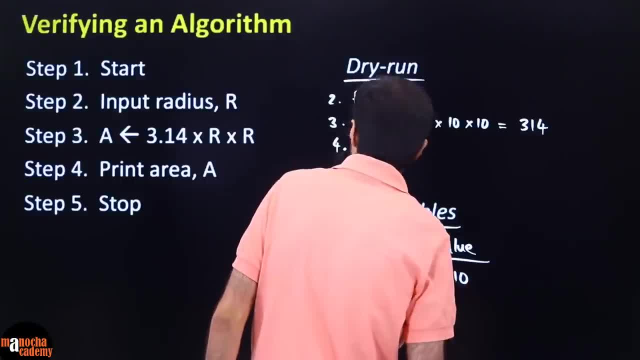 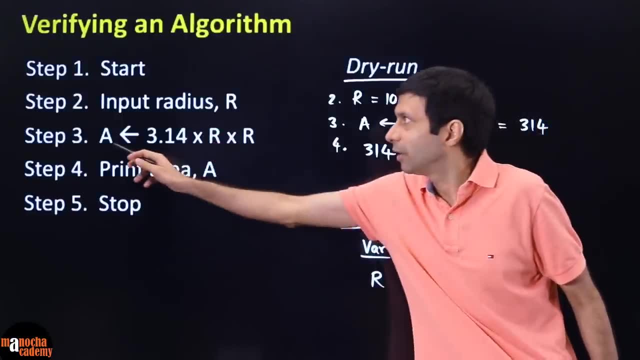 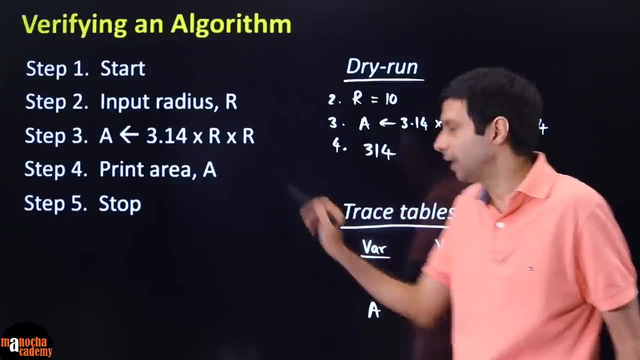 and let's say the input value is 10, so we'll put it in our table here. after that we move on to step number three. what is the next variable here, area? so we'll put the variable a, and what value will it take? 3.14 times 10 times 10. 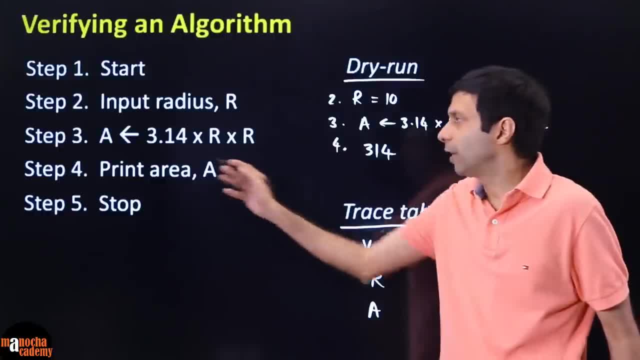 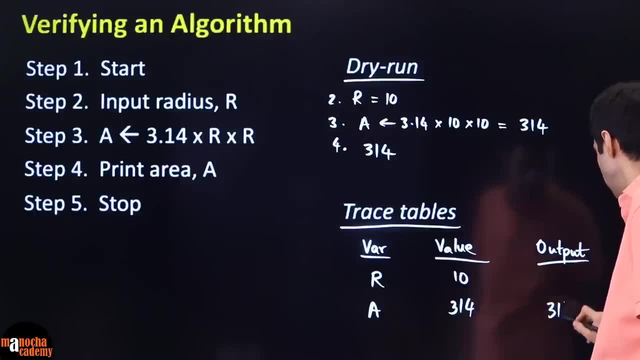 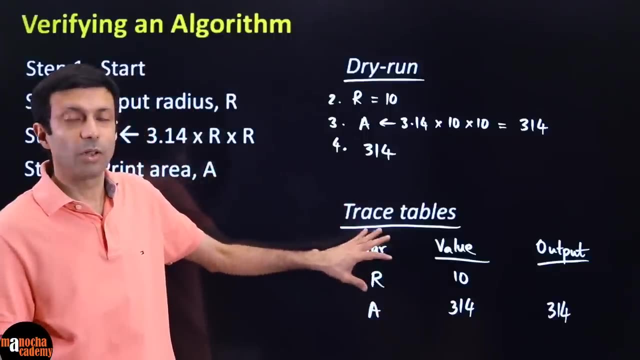 so it takes the value of 314, and then we are printing area so you can keep an output column here also. so after this stage the output will be 314. so this is known as trace table, where basically you are seeing that all the variables that are there in your 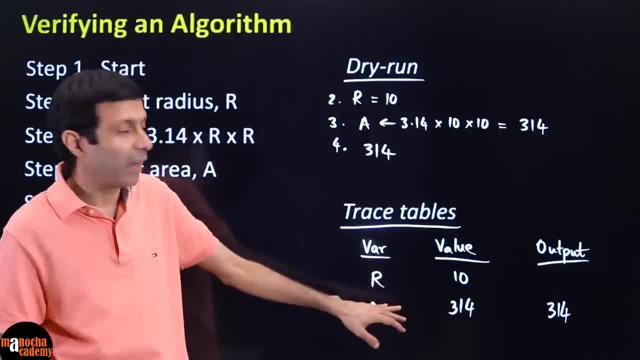 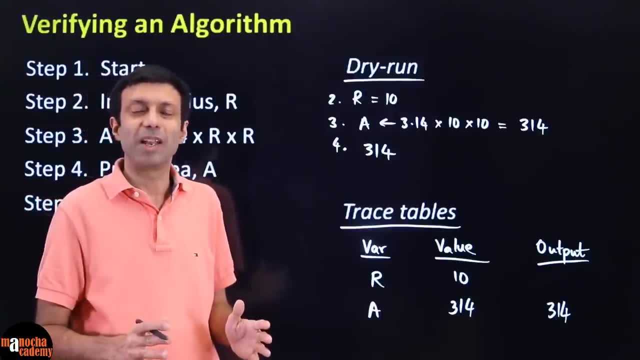 memory or in the computer's memory? what are the values, how are the values changing and what is the output? so this is how you verify an algorithm very easily, using pen and paper, without running it on a computer, and it's very important, especially for the complicated ones. 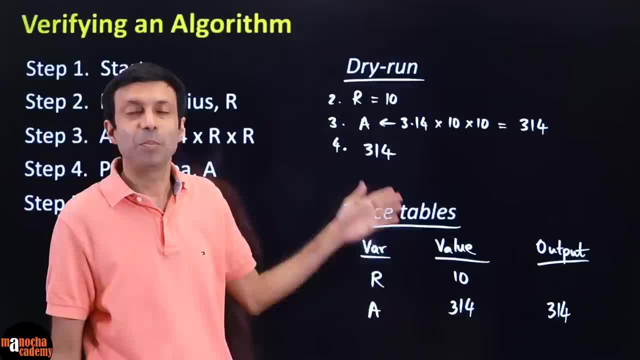 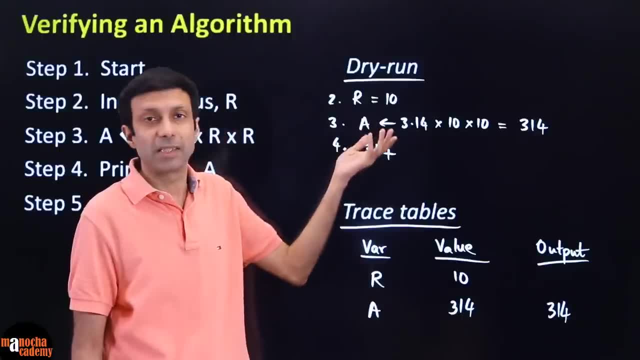 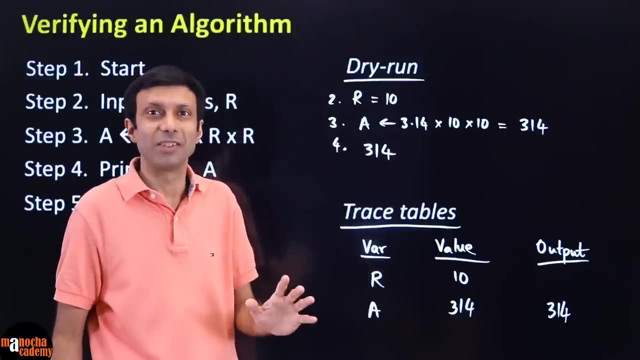 to verify it using some simple examples. sometimes, if the they have different edge cases or difficult cases, like if, let's say, some program can take a negative number, then you should try a positive number and a negative number and make sure it works for both cases. it's not good if the program is only working for one case, right. 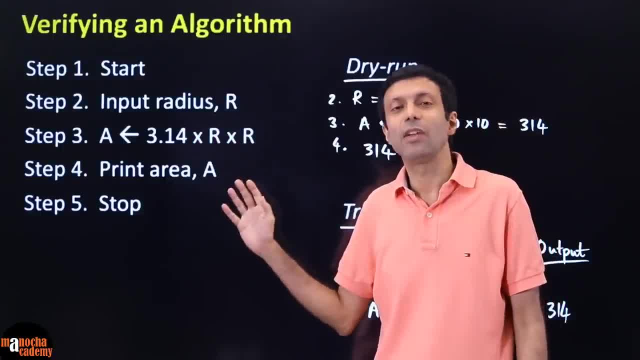 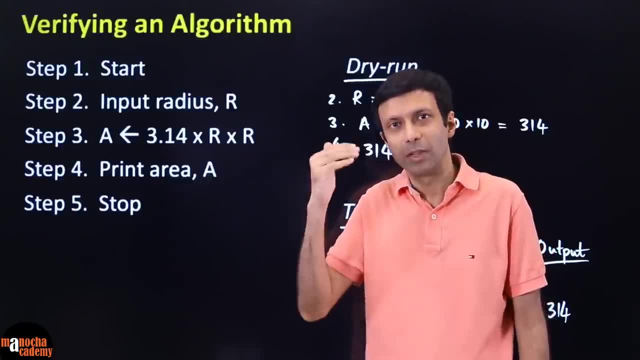 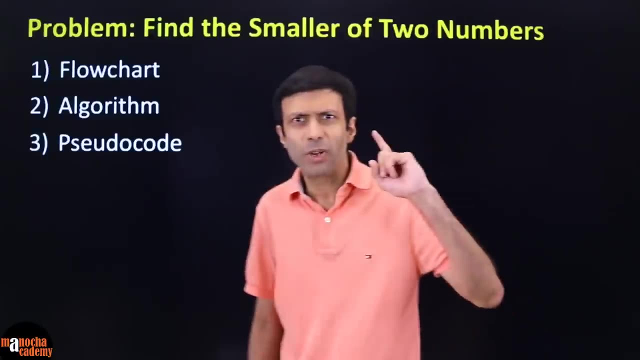 so this is what we call as verifying: checking if your algorithm or your flow chart or your pseudo code. so you can do this for anyone: checking if your algorithm- the step-by-step procedure- is right. so now we have learnt all about flowchart algorithm and pseudocode. are you guys ready to pick up your? 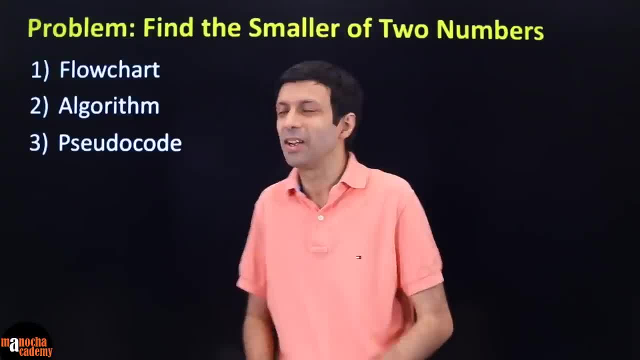 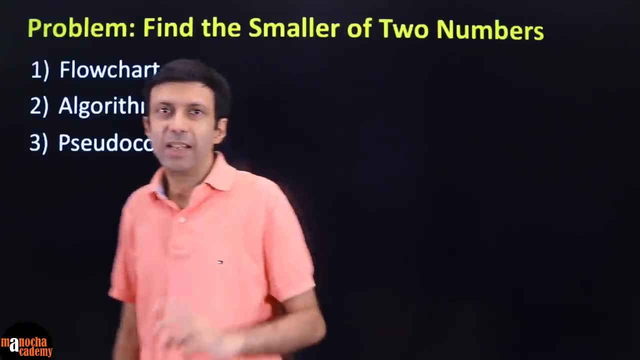 pen and paper and try these out practically. so let's go ahead and do it and we'll start off first with the problem find the smaller of two numbers. so simple question. let's say you want to input two numbers from a user. you want to find the smaller one, which basically? 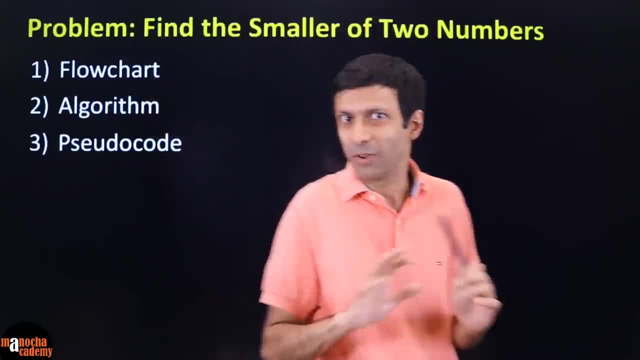 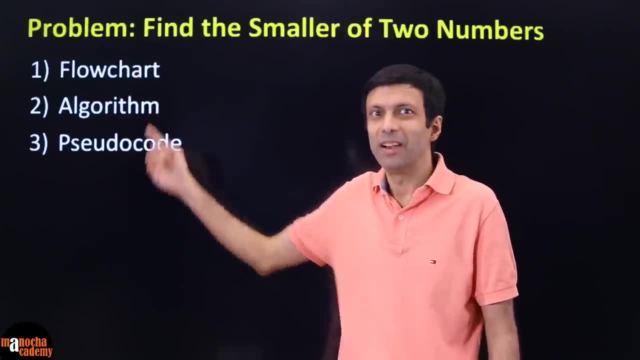 means the minimum. and now what we are going to do is: we are not going to write Java or Python code. we are going to write the recipe using flowchart style, algorithm style and pseudocode. let's start with flowchart first. so, before we look at the flowchart, let's quickly discuss the 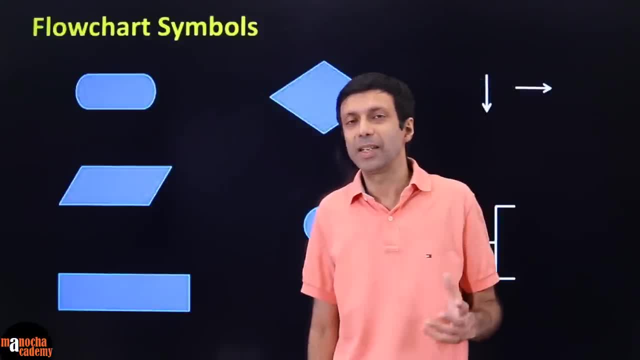 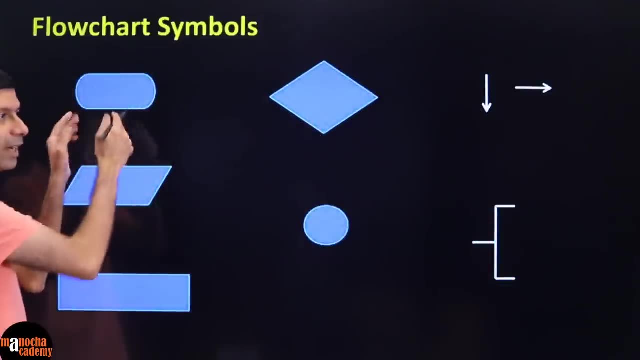 different types of flowchart symbols. I showed you a simple example. now let me formally write down the names of these symbols. so this first one, which looks like a rectangle, but it has this kind of curve, so almost looks like an oval, but not really an oval here. this is known as star. 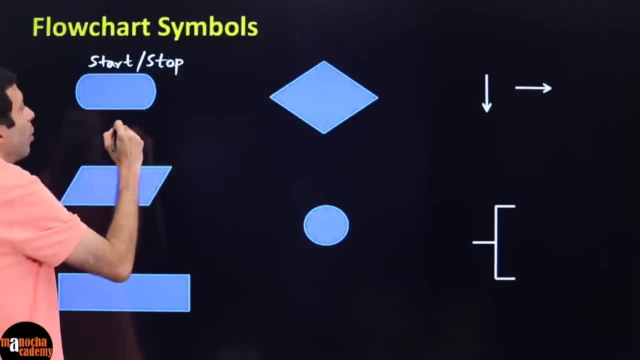 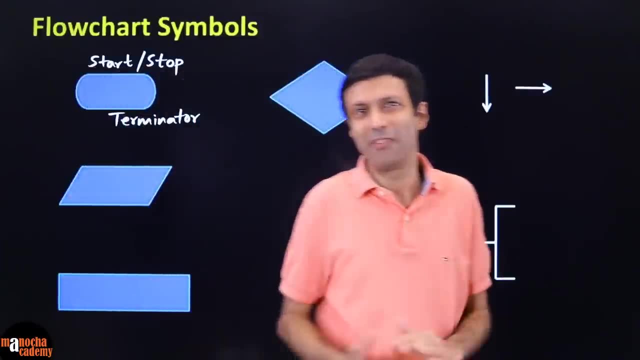 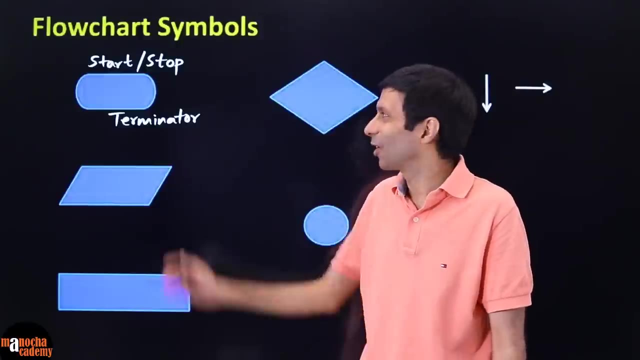 it's used for start, stop, so it is often called terminator. have you guys seen the movie terminator? I think it's one of my favorite movies. right, it was released, I think, when I was your age or something. so, terminator, these are called terminators because they start and stop the. 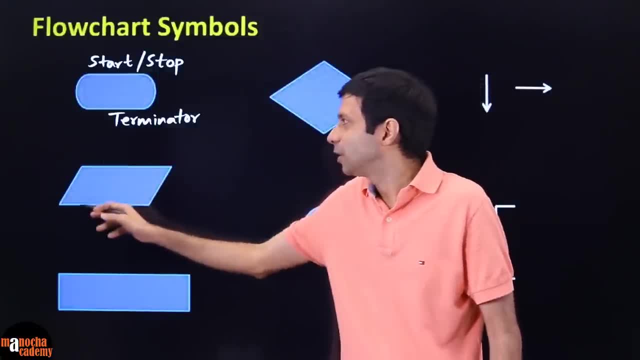 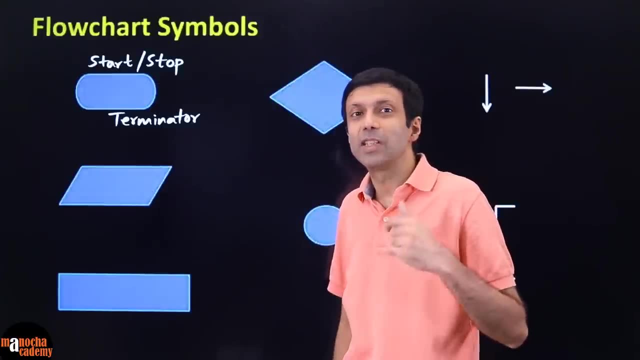 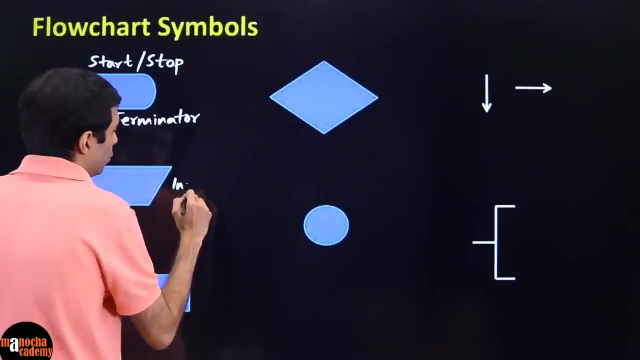 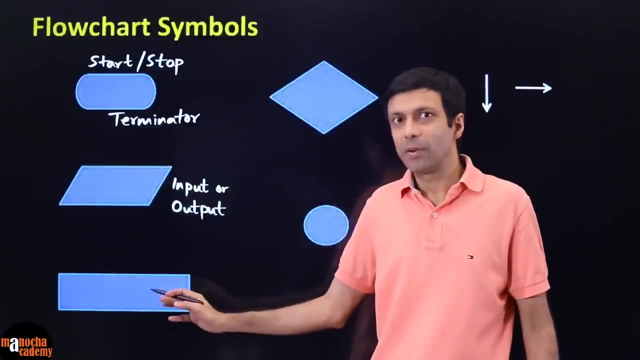 program. next one: what do we have here? this parallelogram kind of looking thing, what is this known as? so, when you have this parallelogram shape, this is for input, output, right, this is to do input or output. so this guy is used for input. so it's our input or output box. and the next one here, the rectangle one, remember, which contained: 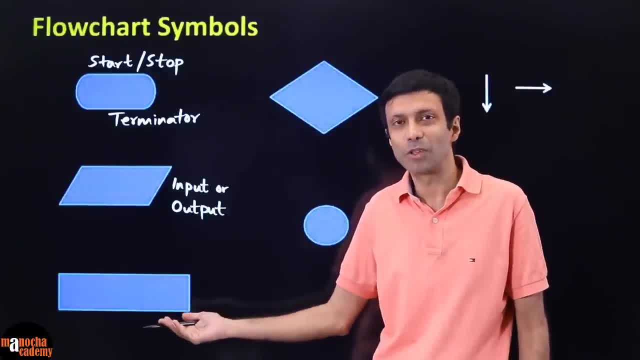 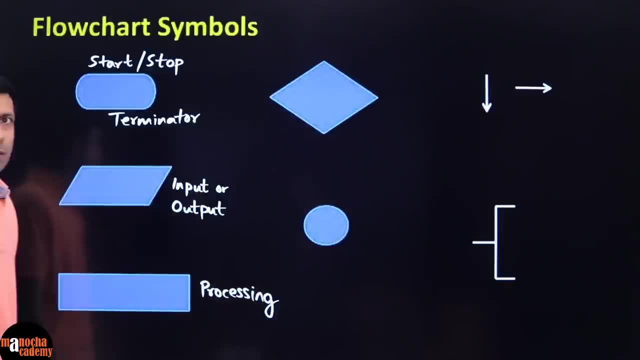 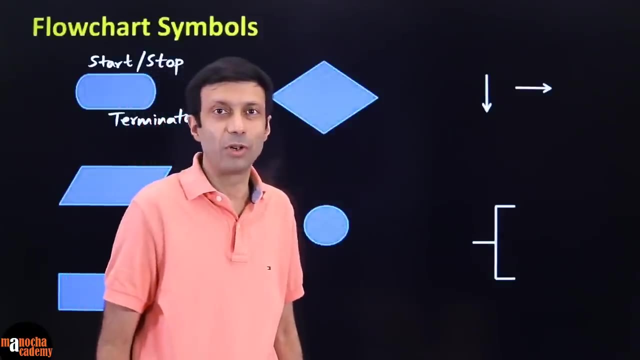 the formula. what is this? this is the processing box, or computation. so normally we call this the processing box used for processing. so you must follow these conventions, these symbols. so you must follow these conventions, these symbols. so you must follow these symbols. so the next one: if you have this diamond shape kind of thing, do you know what is this used for? and 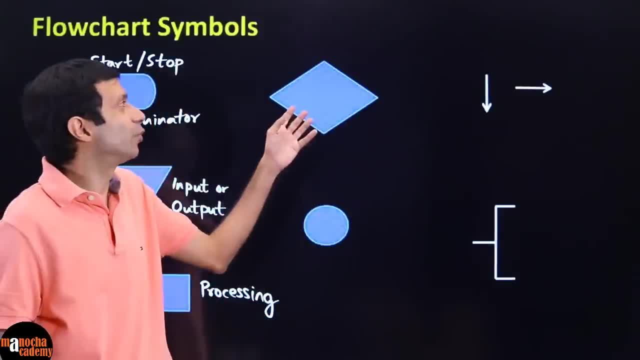 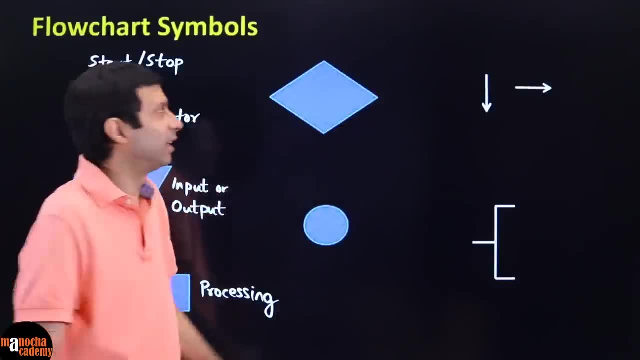 we will be using it in our examples. this is used for condition or decision. a yes, no, so you put your condition inside this and then you can create branches. so this is used for condition, or what we call as decision box. then you have this symbol where you just have a simple circle, this small. 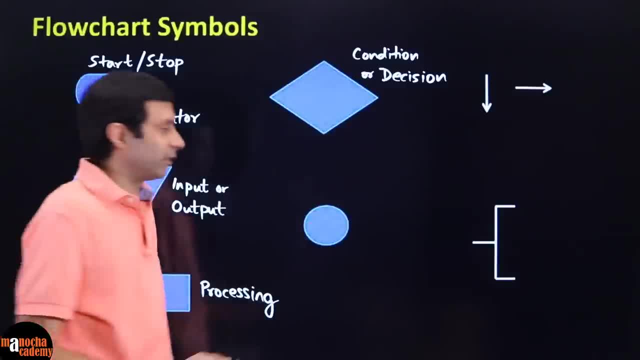 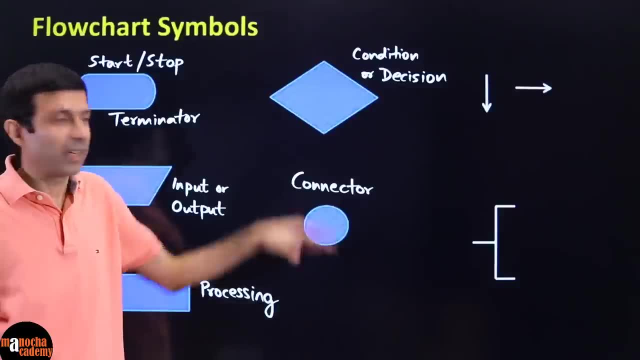 circle. so these are used as connectors. what is it used for? so this is used for decision box. so what is the connector used for? for example, you are writing a flow chart and then you run out of space, right? so you have reached the end of the page. now you want to continue to the next page, so 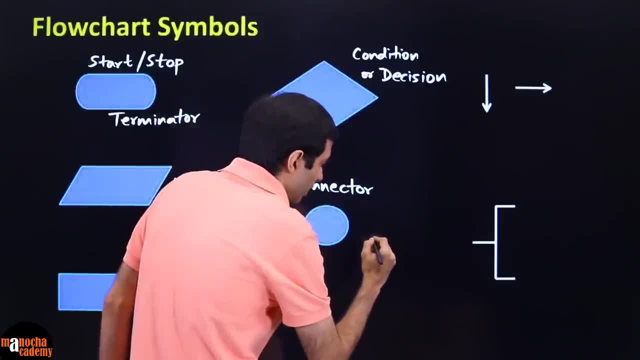 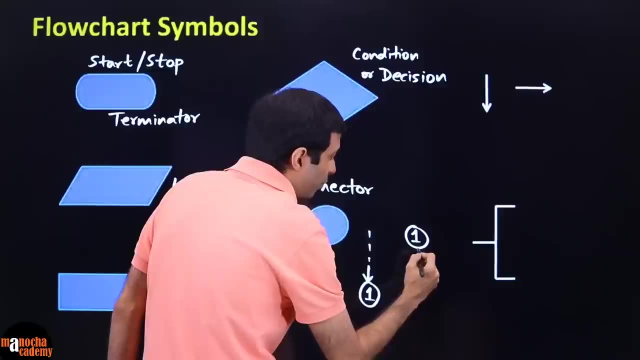 how do you do it? you use a connector. so let's say you're writing your flow chart and then you end with this connector and you can label it something like one or two. so you put the number one here and in the next page you continue. you put the connector again, write one, and then you continue. 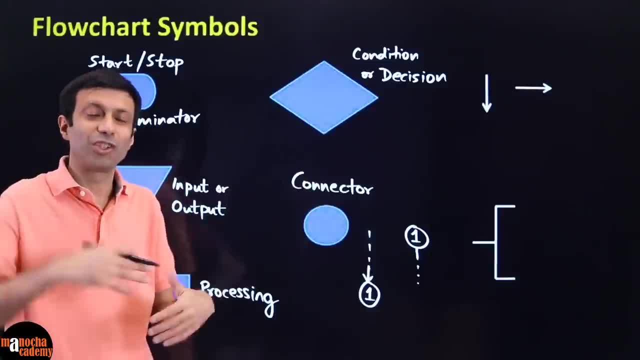 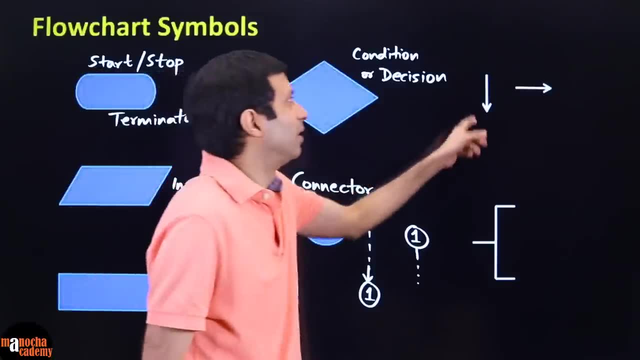 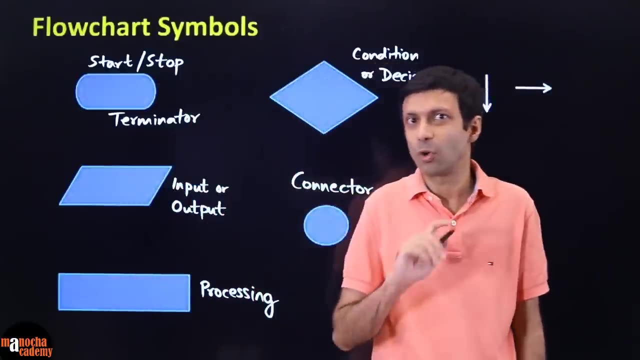 your flow chart. so connector is used to connect flow charts on different pages, so it's more like you know, continuing the flow chart. then you have these arrows. remember flow chart. the boxes need to be connected with arrows, not with simple straight line with arrows, because you are showing the flow 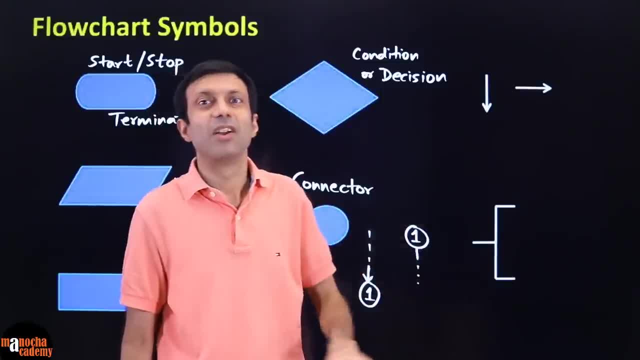 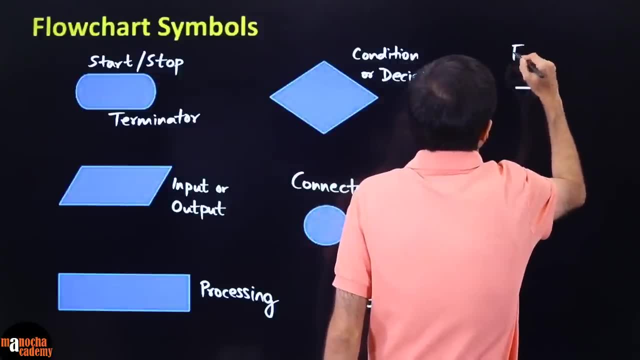 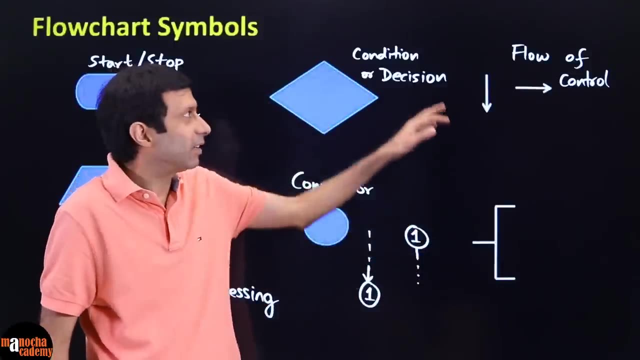 the direction of flow of the program. so these are known as arrows, which represent flow of control. so these represent for us, flow of control is our program moving downwards to the left, to the right. that's how you represent with the arrows. and this last one, remember I use this- this is to write. 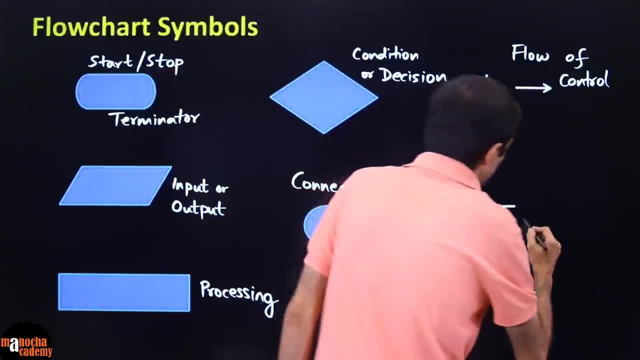 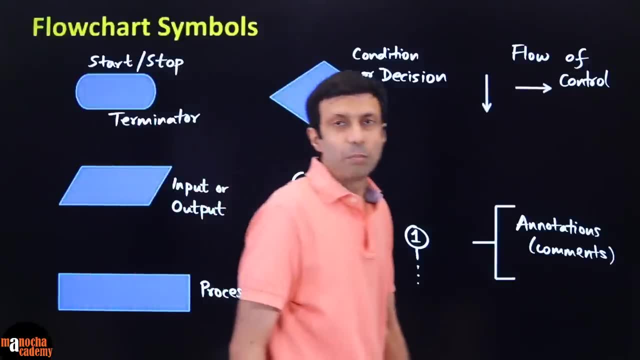 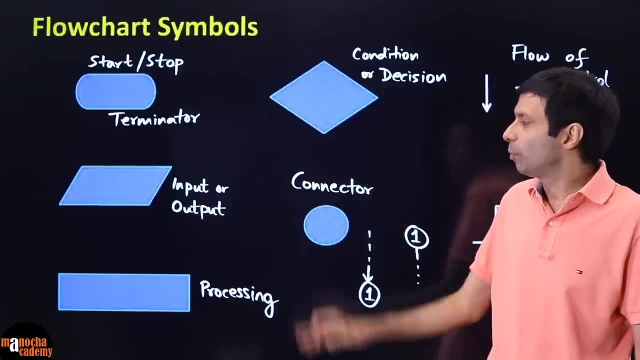 comments or your annotations. so this is used for annotations, comments to your flow chart. so these are the most important ones. there are, of course, more flow chart boxes and symbols, but these are the most important ones that are done and we'll be using them today. so are you. 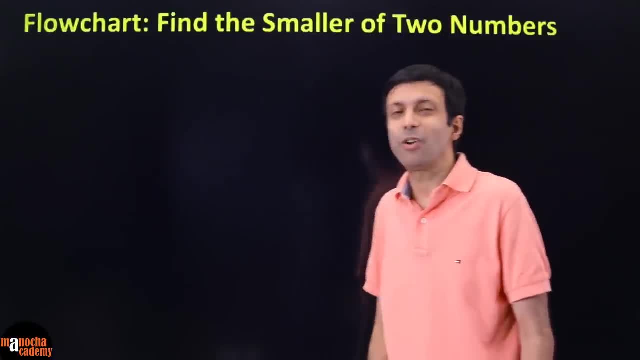 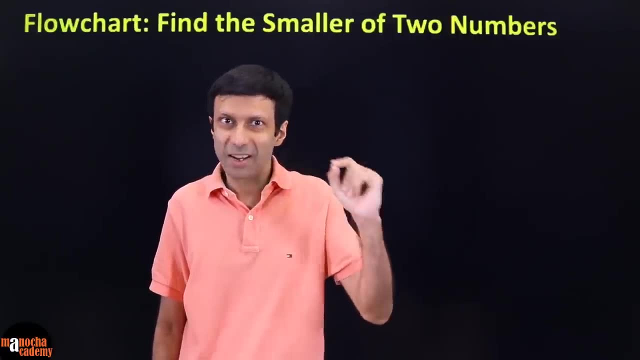 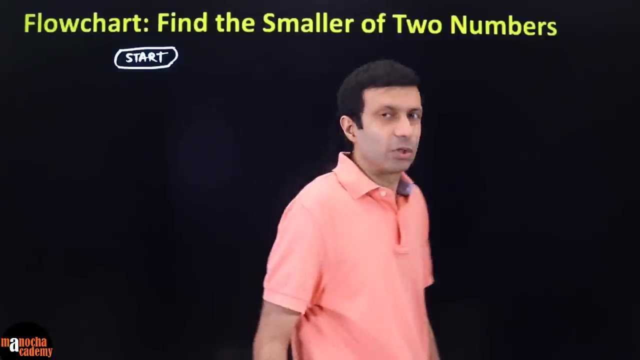 guys ready to draw the flow chart for find the smaller of the two numbers. so that's our question. so how do we start? remember, flow chart is simple. it starts with the terminator start, so let's do that first. so we're going to write start and please put it in this sort of box right now, when you want. 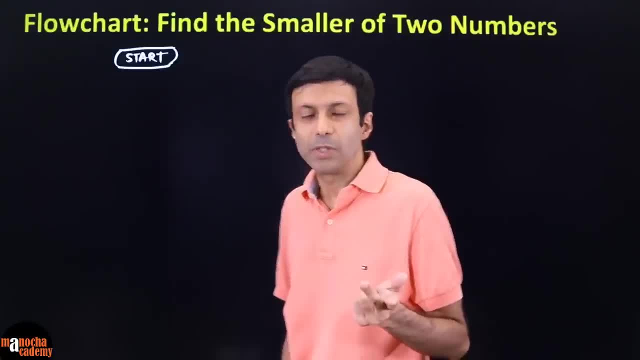 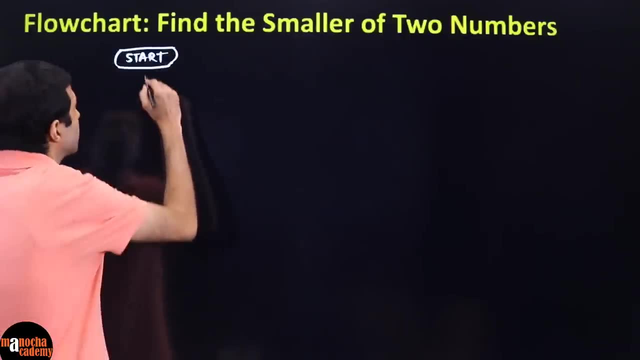 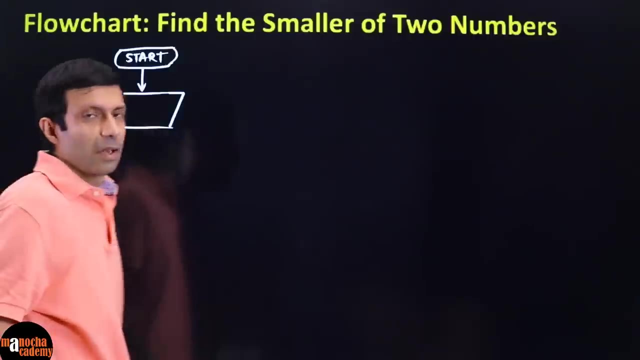 to draw the flow chart for find the smaller of two numbers. clearly you need to input two numbers from the user and then find the smaller. so we need to input two things here. so let's make the input box first. so please draw the arrow and input is shown using this parallelogram kind of symbol. now you 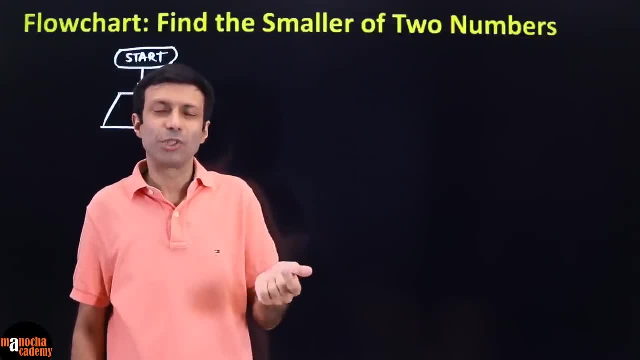 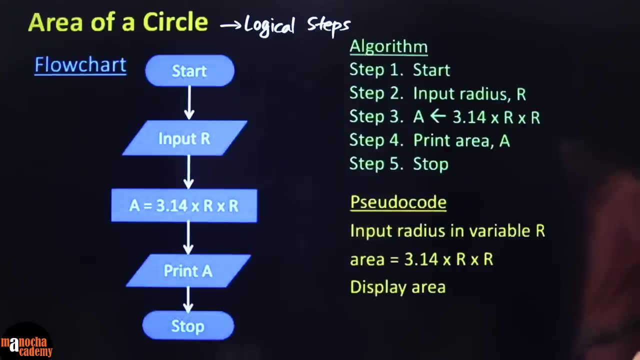 can draw two boxes and write input a and then input b, or you can do a shortcut and simply write input a, comma b. so see, we are trying to do a flow chart like this. now sometimes you'll see in the books they use all uppercase letters, sometimes lowercase in flow. 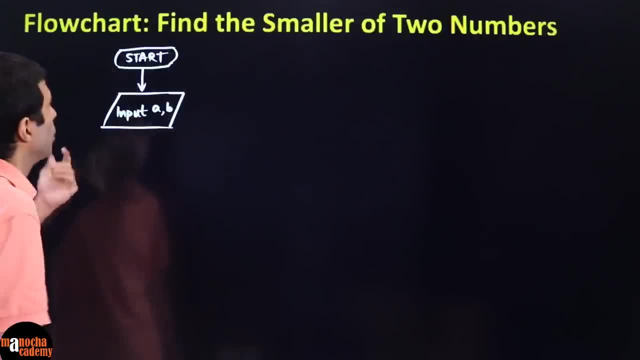 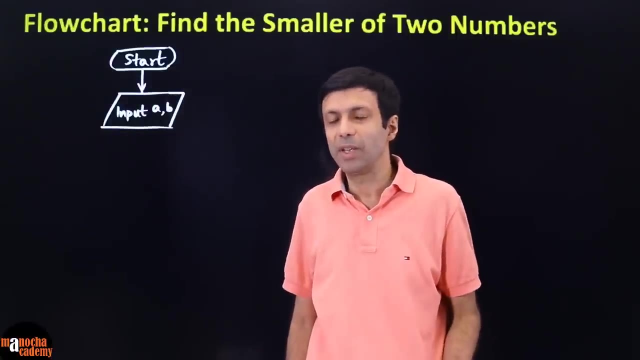 chart, doesn't matter whatever style you like. so since i've used some lowercase here, i can, you know, write, start in lowercase as well, just to keep it consistent. and please connect these box with the boxes with the arrows. so our input is done. we have input two numbers: a comma b. 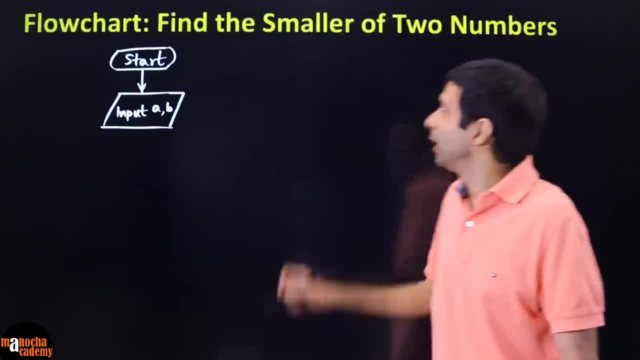 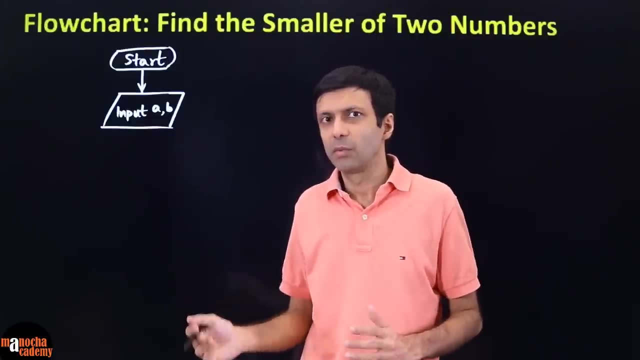 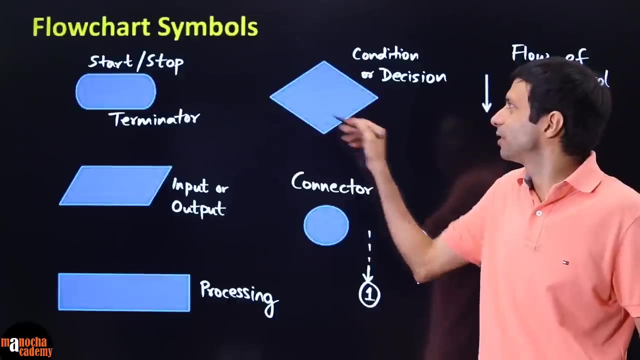 now what is the next thing we need to do? we need to find the smaller of two numbers, and obviously we can print it out. so how do we do that? which symbol should we use here? so now we have to ask a question: who is smaller or who's bigger? right, so we'll use this, you know. 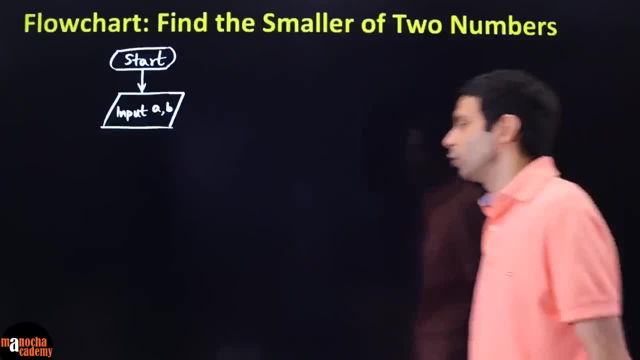 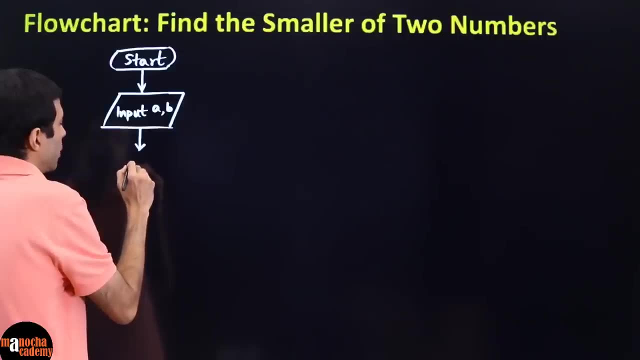 decision or condition box. so we are going to use that. so the next thing will be it will flow into the decision box where we are going to ask the question: is a less than b? and you put a question mark and then you can draw this decision box around. it is a less than B. so again see, 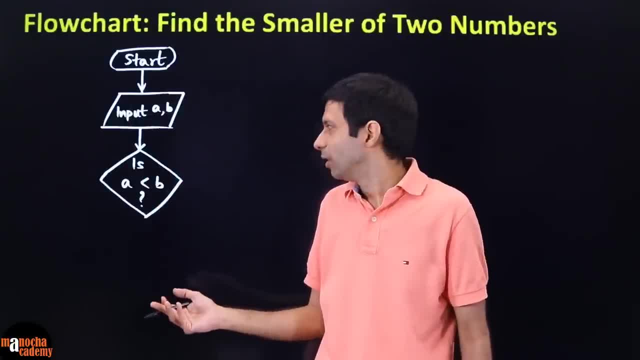 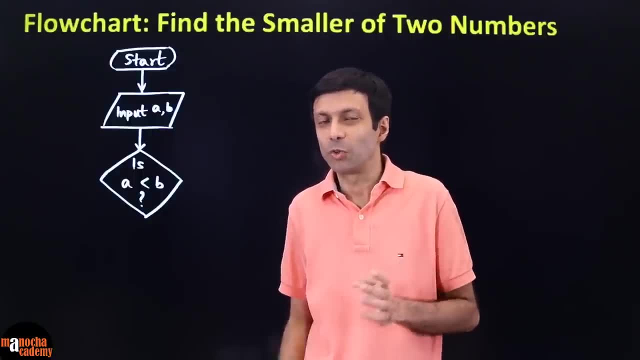 written in simple English, right, not any fancy code. so now, if is less than B, there can only be two answers, either a yes or a no. so from a decision box you can have a yes or a no. computer doesn't like maybe, and all right, it's binary. yes. 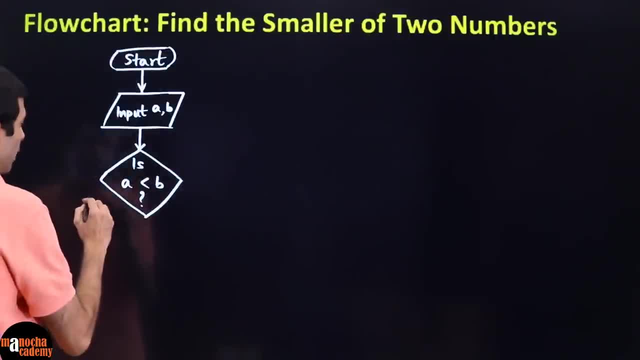 or no. so what will you do here? so you can have two things coming out, either a yes or a no, so two things flowing out. now you could flow the two things out of here as well, so you could have your yes and no here whatever style you like. so 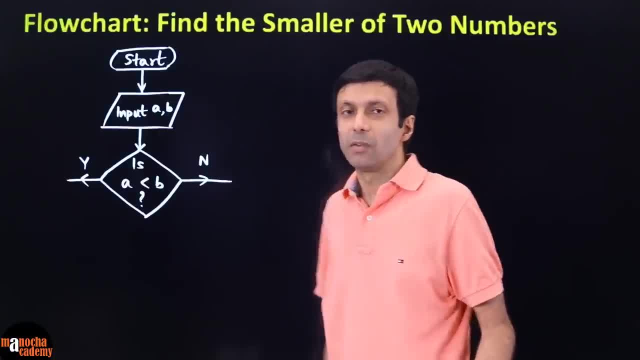 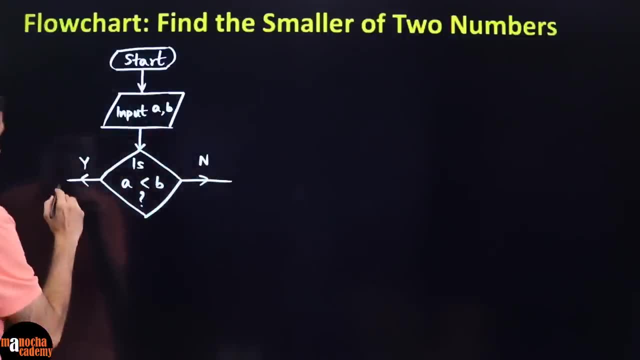 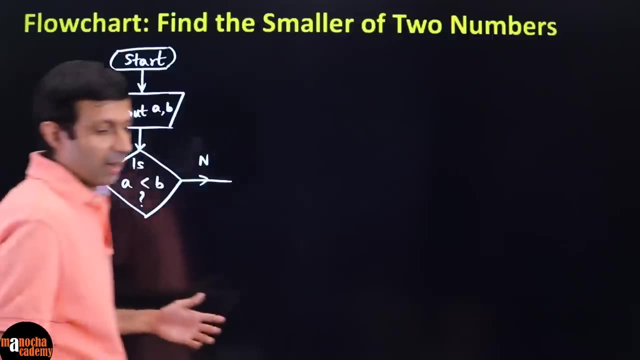 if a is less than B, what value will you print? we want to find the smaller, the minimum number, so obviously we are going to print a, so let's write that down. so once we have this, you're obviously going to, so you'll be printing a, and if the question is, a is. 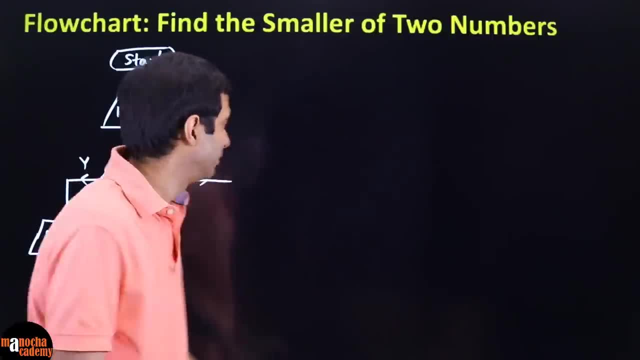 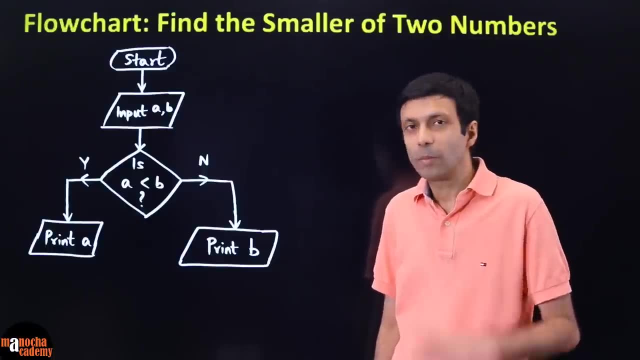 not less than B. who will you print? obviously the value of B clear, and we put this in parallelograms because we are doing an output now. now some of you might be wondering what about the case if a is equal to B? so let's say both of. 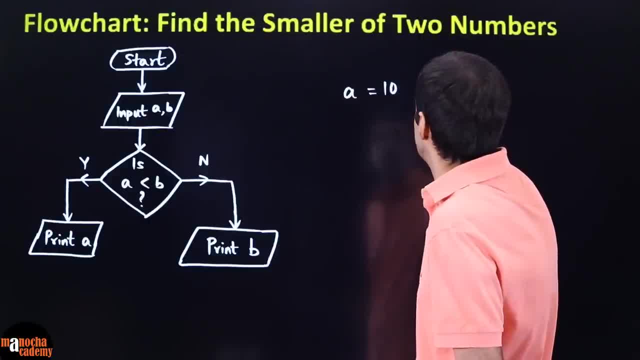 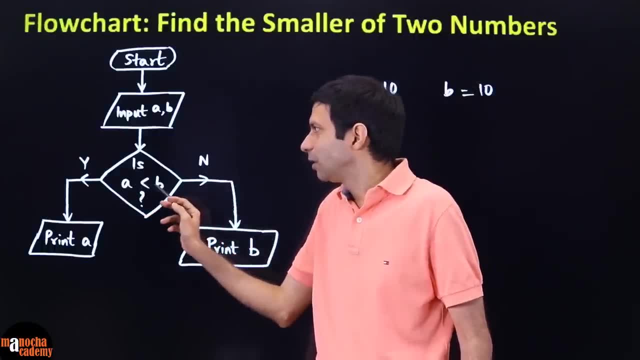 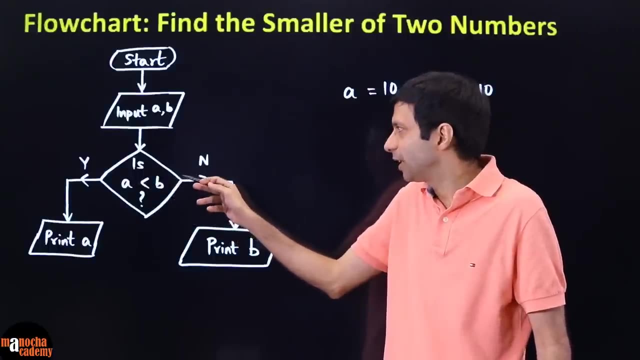 them have the value 10. so let's say a is 10 and B is 10. where will this flow chart take us? so when you reach this question: is a less than B? is it going to be a yes or a no if both are 10? because 10 is not less than 10. so obviously the answer is a no. 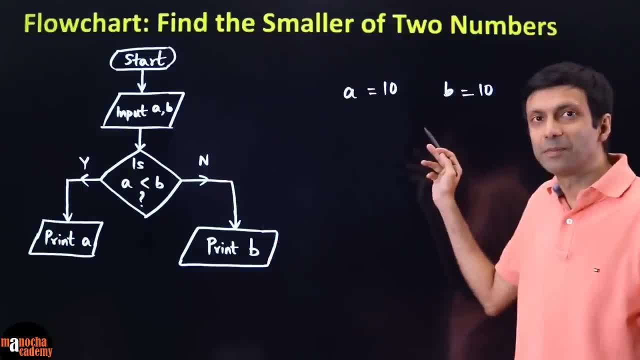 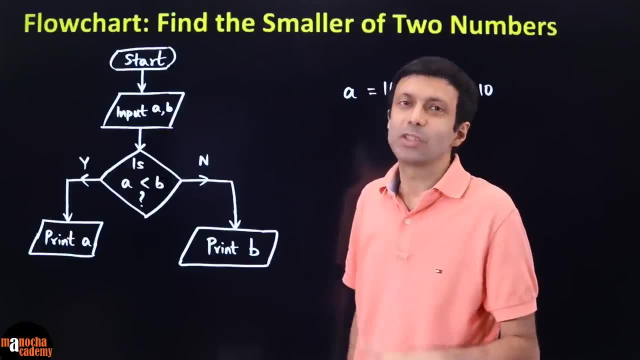 it'll go here and it will print B, which is 10. but it doesn't matter whether you print a or B, because both are equal, so both are correct. we don't need a third case here, because if both the numbers are equal, any one of them is the minimum. 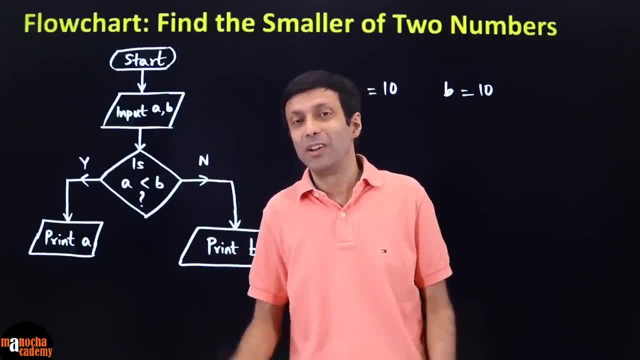 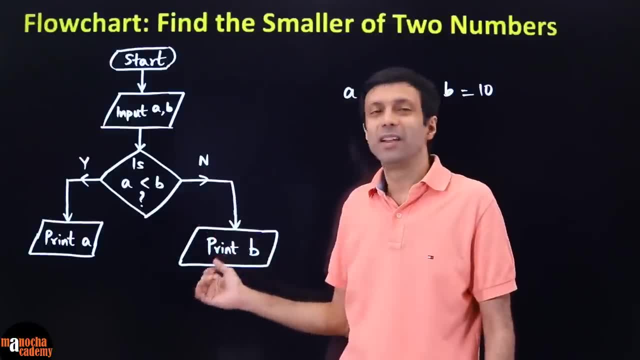 see, this is where flow charts help you. this is where thinking of the logic helps you to get the right answer. make sure your logic is right before you code, and this clear from here that you are still going to get the correct answer. now, how do you finish it off so? 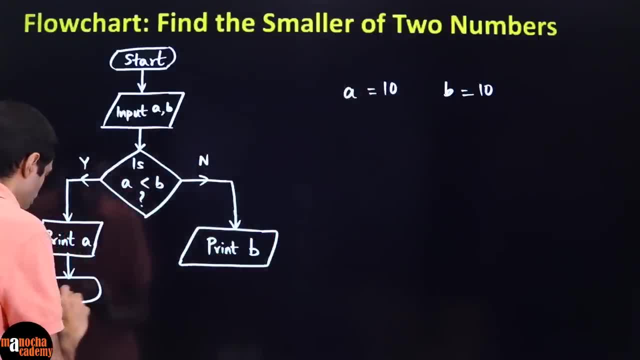 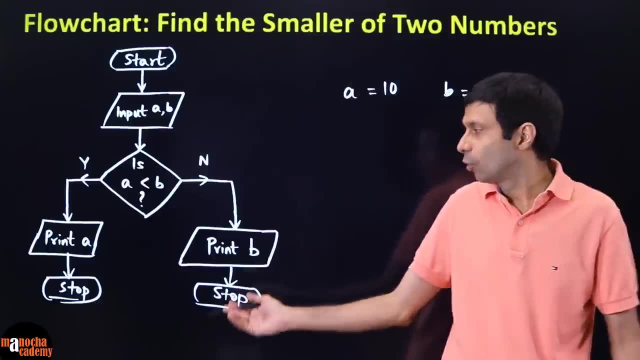 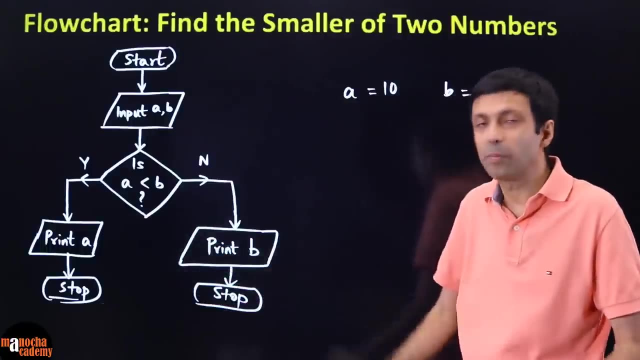 one. you know, one way is to write this, so you do a stop here and similarly, you will create a stop here. but is this a good flow chart? no, because there should only be one start and one stop. this is not a good style. please do not do it. you. 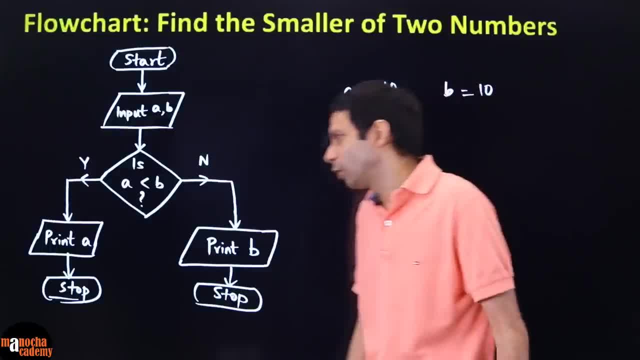 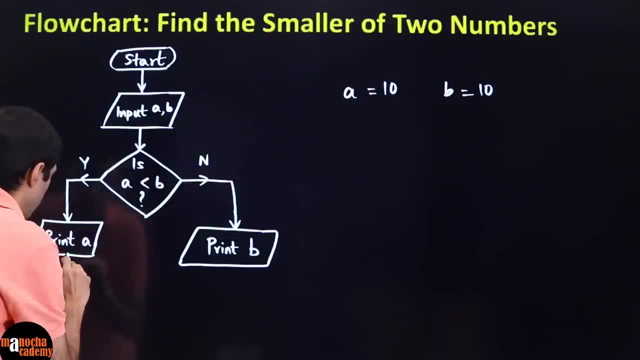 cannot have two starts. two stops looks very weird. so what do you do here? you just connect these two. so please do not create two stops. so what you should be doing is just join these two, so the flow of control will go this way, and then you create your stop here. 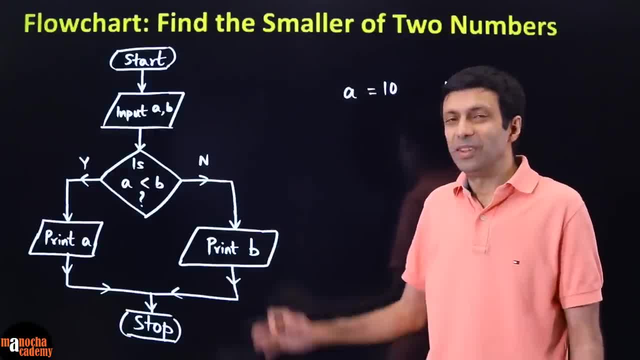 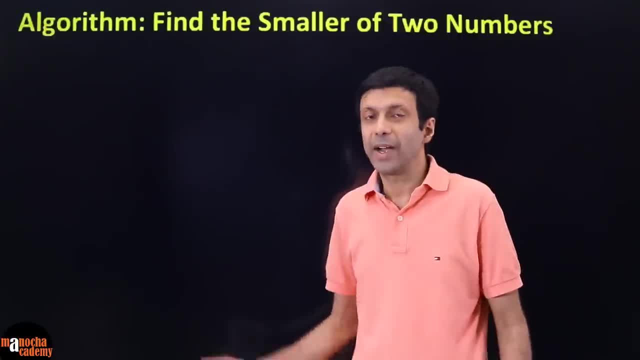 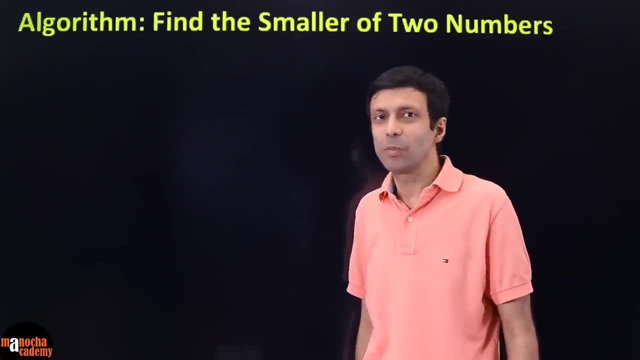 there you go. so this is how we write our flow chart. is this flow chart absolutely clear to you? next, we are going to write the algorithm for the same question, because we're going to practice all the things- flowchart algorithm, pseudo cod. so what is the algorithm going to be? so remember. 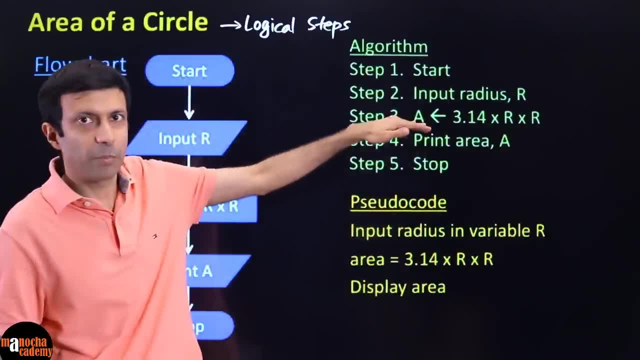 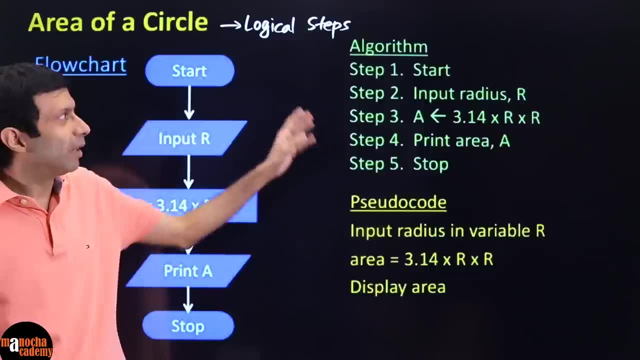 algorithm means step-by-step right- step 1, step 2, step 3, so you need to write it in this style. please think how you write the algorithm and again, you're sort of writing it in English and expressing the formulas if needed. so in the algorithm. 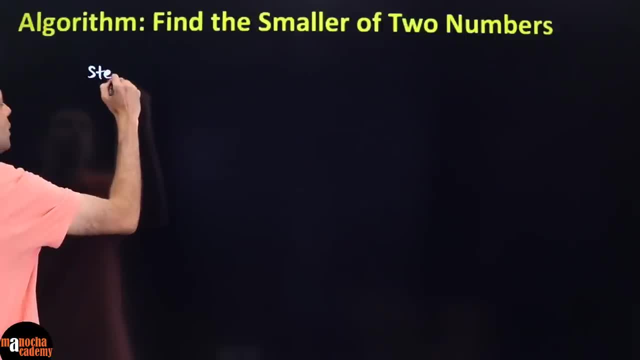 again, we're going to write the step-by-step because it's a step-by-step procedure. So step 1, we are going to say start. sometimes you know this start stop is ignored in the algorithm. but better to write it down so that shows the start of the program. 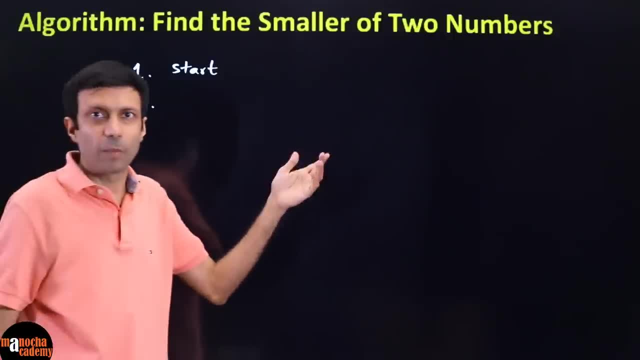 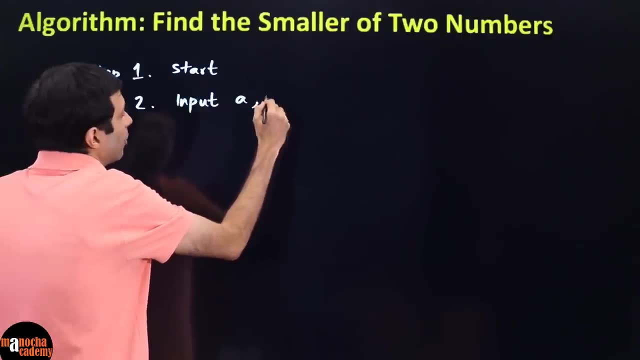 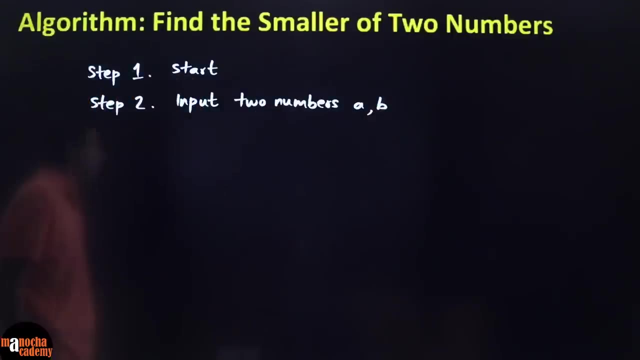 What will be the next step? Input the two numbers a, b. now you can write input a, next input b, or you can put it in one line so you can say: input a, b, or you can even say: input two numbers a, b, right. 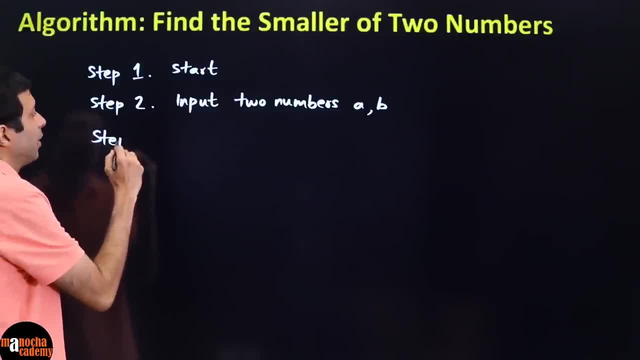 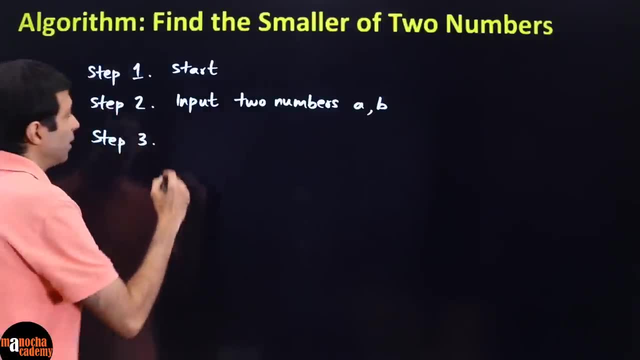 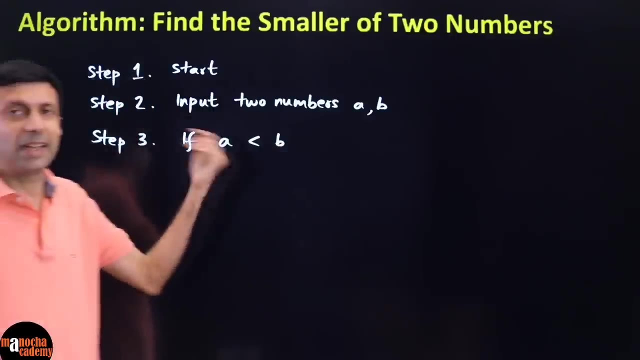 And then what will be your next step? Step 3, you want to find the smaller of the two numbers. so again here, you are going to give the decision. so what you are going to say: if a is less than b, you are going to ask this question: right, is a less than b? then print a, else or otherwise. right, whatever style you are following, else, print b. 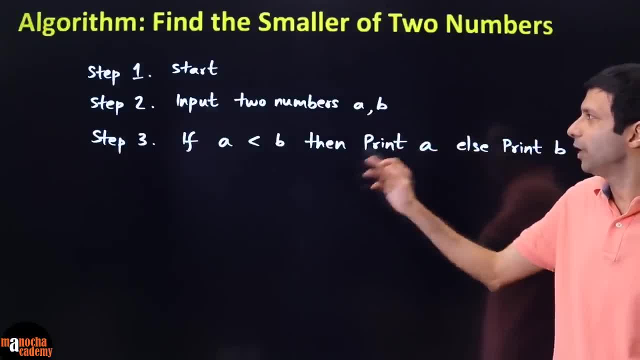 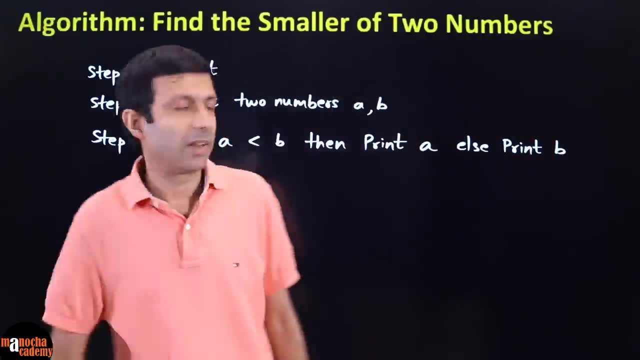 So this is our decision. So this is our decision. step: you can see clearly. we have written: if a is less than b, then print a, otherwise print b. So there you go, that's our algorithm, and then we can end it with step 4, stop. 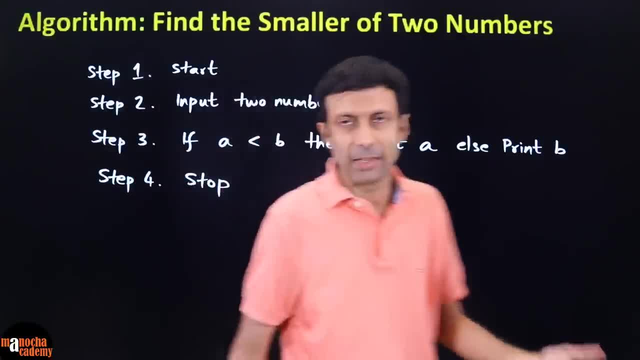 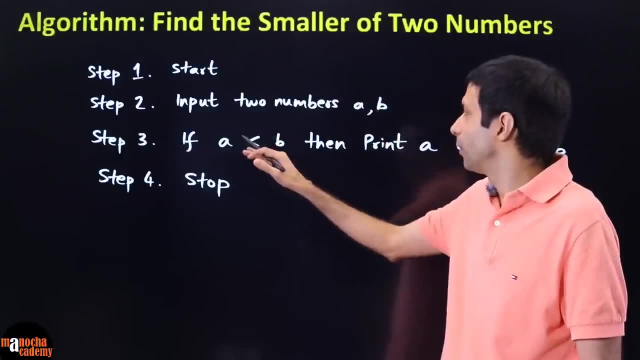 So this is how you write your algorithm. of course, it could be written in slightly different styles. you may not want to write two numbers. you can just say input a, b or x, y, whatever. and this is how you express the if condition. 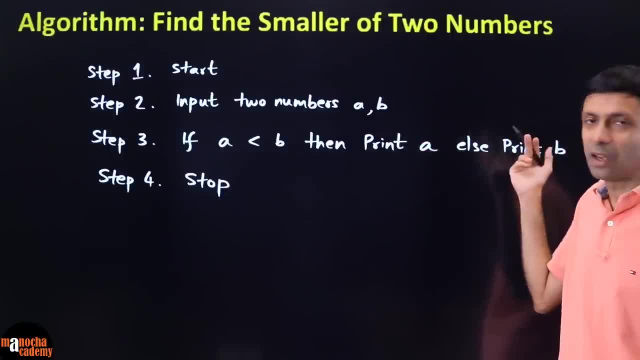 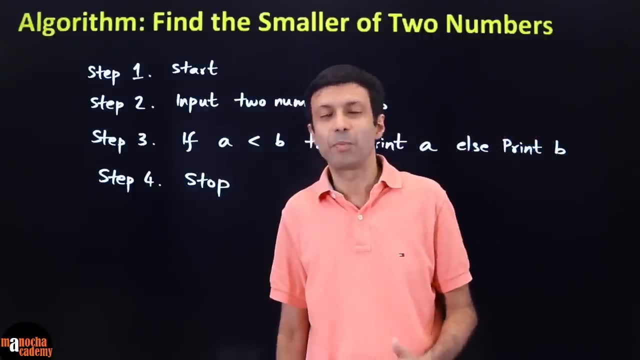 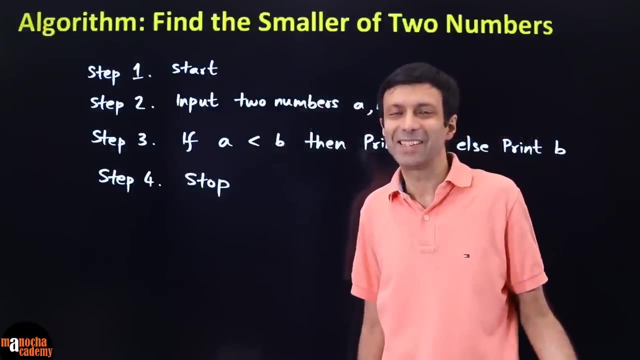 You can put it like this In one line: if this, then this, otherwise, or else do this. So do you guys agree? this is the correct algorithm for our required program to find minimum of two numbers. If it is maximum, you will just simply change the sign to greater than that's it. 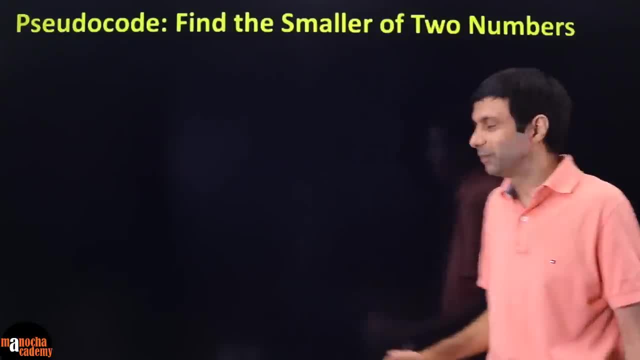 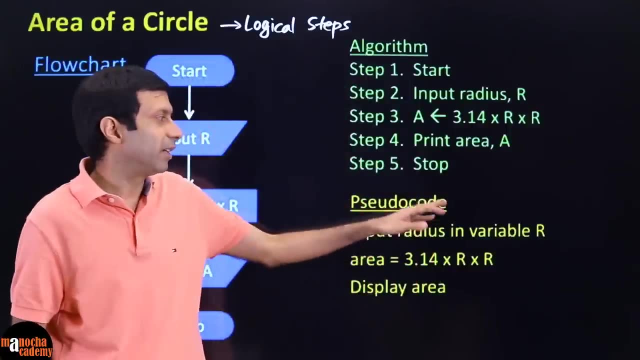 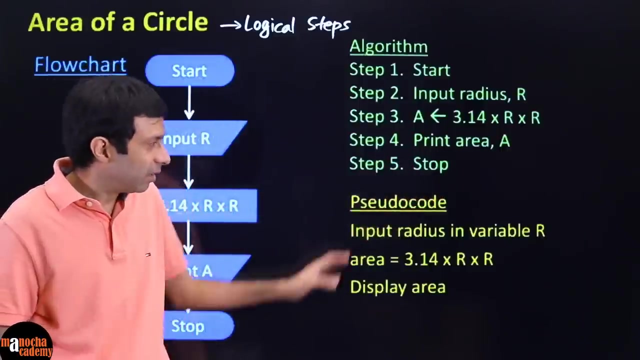 Now let's try to write the pseudocode. So what is the difference here? So remember, pseudocode is informal way of writing code, right where you say things like input radius invariable. or you can say: input two numbers in variables a, b, then again you do your, you know whatever computation or decision and do your printouts. 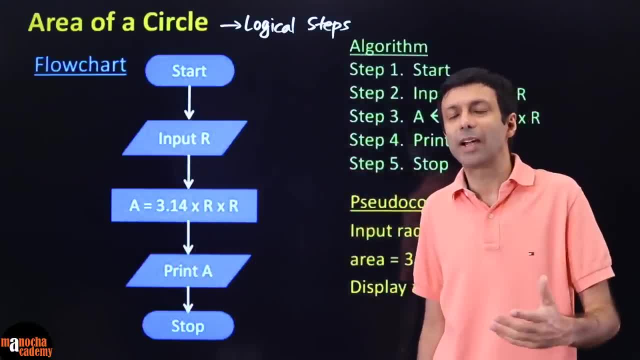 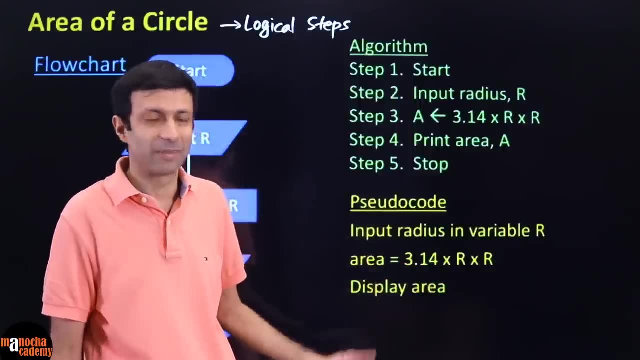 So it's an informal way where you're not following any particular language. you're trying to write it in sort of simple English and express some formulas, if needed, and express your logic. So let's go ahead and write down the pseudocode to find the smaller of two numbers. 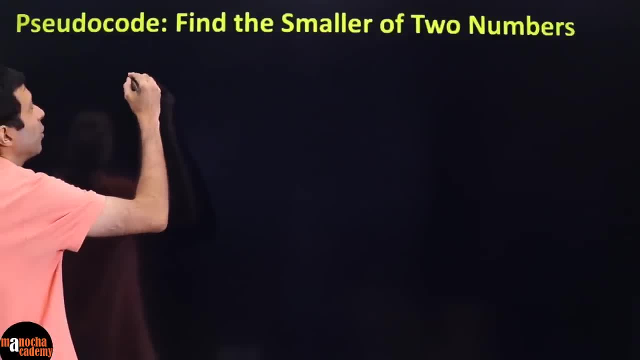 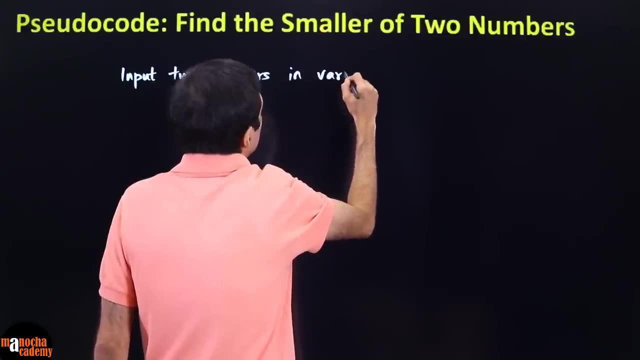 So here usually we don't write One, two, three, we just simply write the code here. So what will it be? Input two numbers in variables a- b, or you can use capital A- B notation, whatever you like. 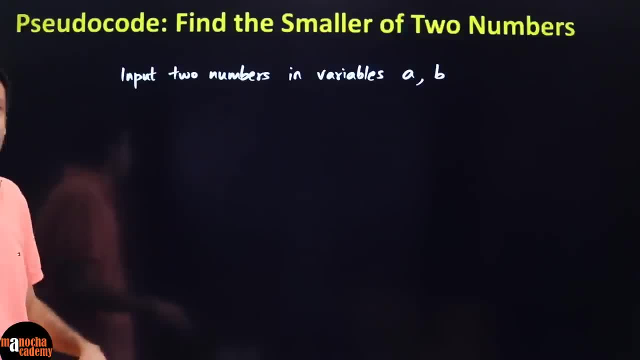 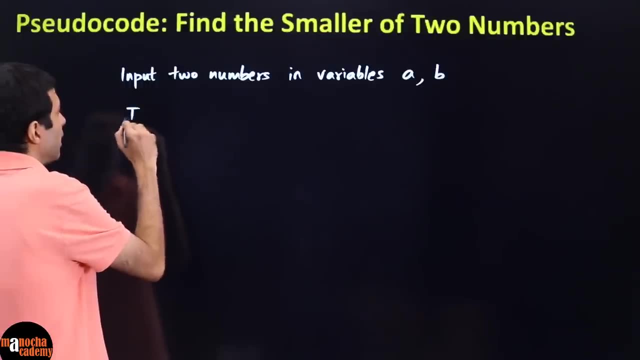 So that is your first thing. You have taken care of the input. Now you're going to write that decision. So we write it more like an informal coding style here, So we can say something like: if a less than b. If you want, you can put a bracket here as well. 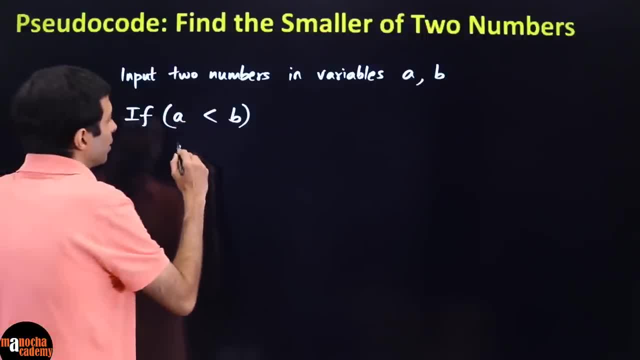 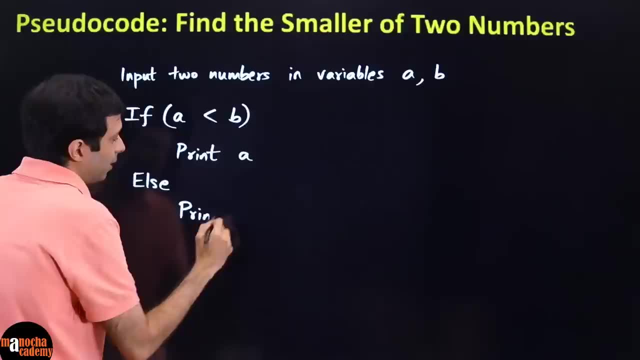 So if a is less than b, then what do you do? Then you print it or you can write: display a Else print b. So this is actually very similar to Python code, except in Python code you have certain colons and stuff. 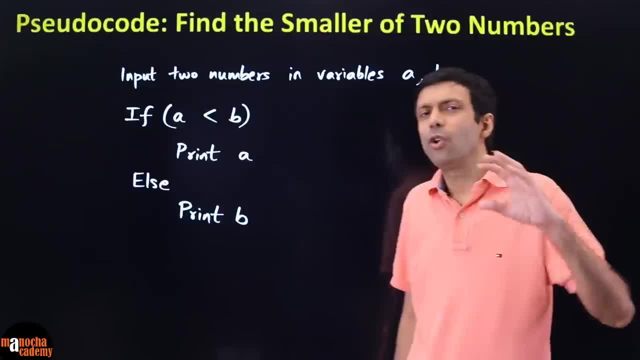 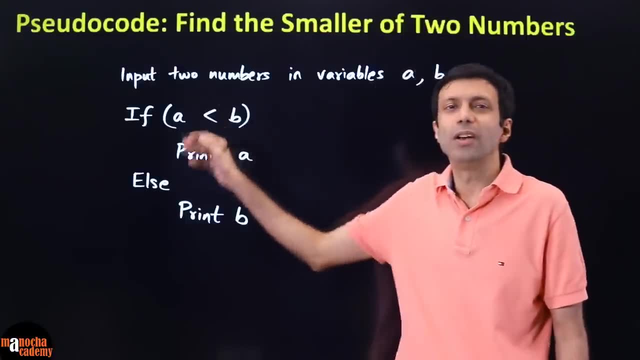 But you can see we are writing our logic in a simple way, not caring are we coding it in Python, C++, Java or whatever language. So we don't care about semicolons and putting all those curly braces for ifs and else We just write it in a simple logical style. 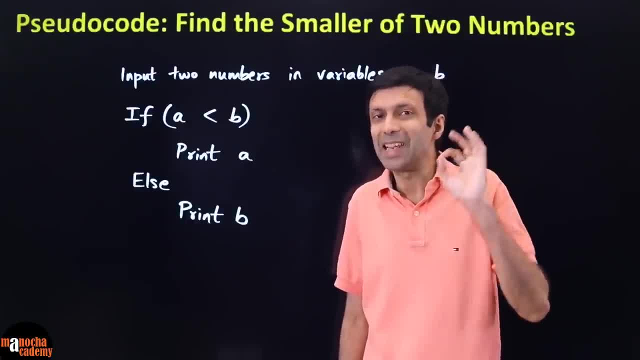 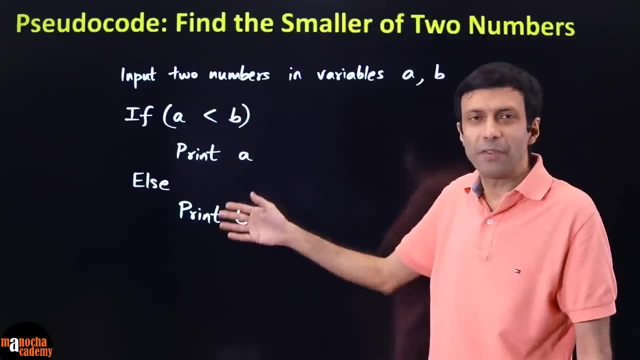 Again, there is no right or wrong way of pseudocode because, remember, it is informal way, So your way might be different from mine or what is being taught in your school, But use whatever convention and try to keep it simple and easy to read. 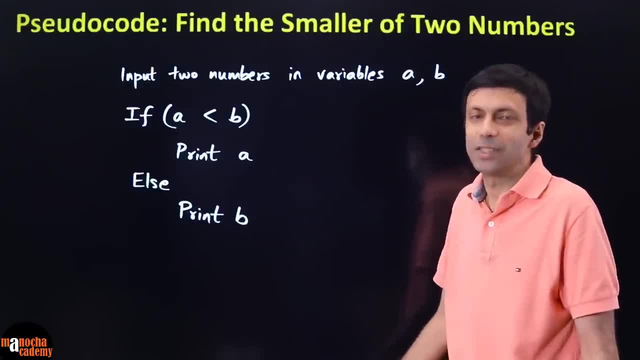 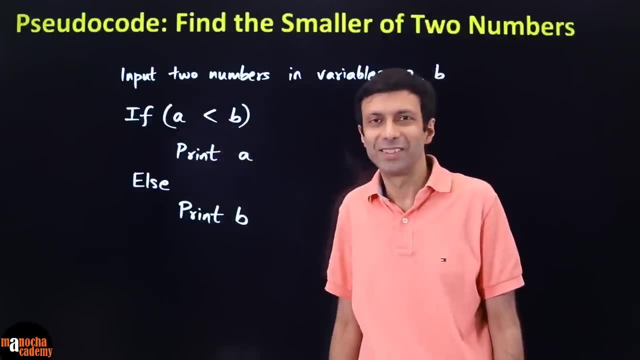 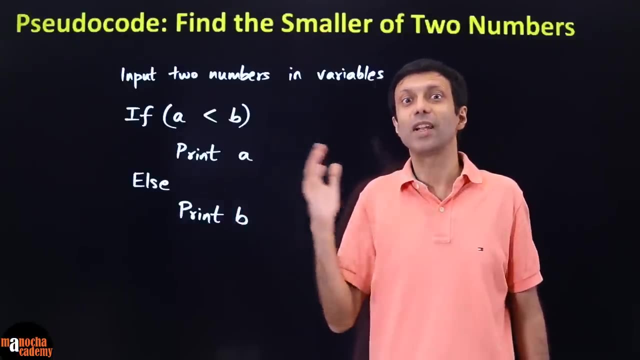 So there we print it out, and there you're done. The code is ended here. So that's our logic. You can see we are making the output depending on the condition here. So is this pseudocode simple and easy for you now. So once this pseudocode is written, it's very easy to translate it into real code in a particular language. 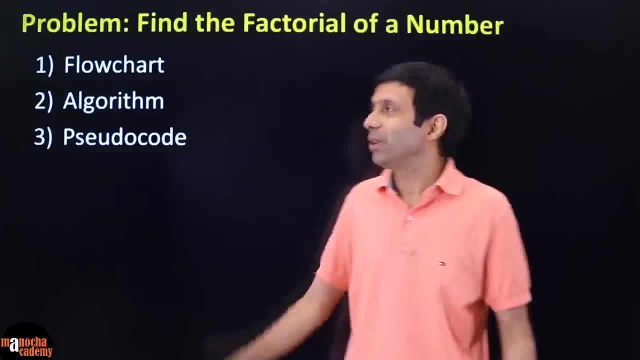 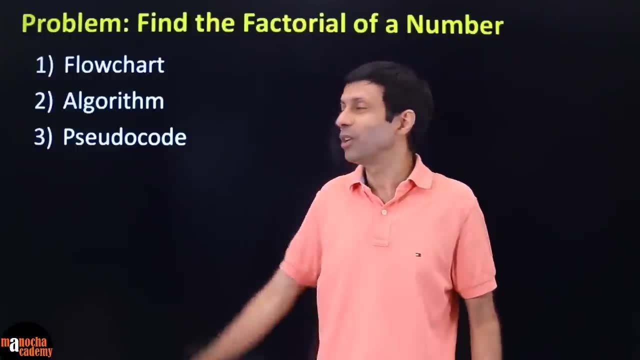 So those were simple examples. That was a simple example. And now let's try a more interesting example which says: find the factorial of a number. And again, we are not going to write code, We are going to use flowchart algorithm Or pseudocode and pseudocode, all the three styles to express the logic here. 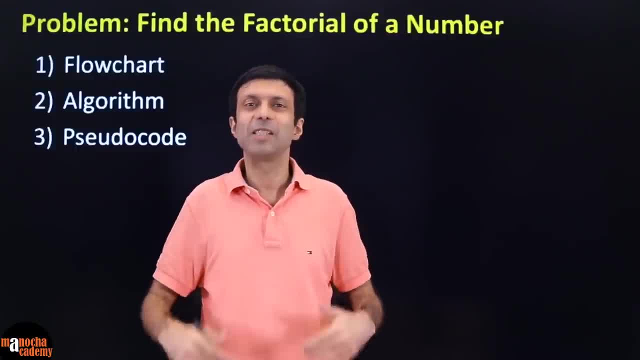 But first of all, what is factorial of a number? Do you guys know? this is a mathematical term. So what does factorial mean? So factorial is a mathematical term, which means that, let's say, you want to find factorial of a number four. 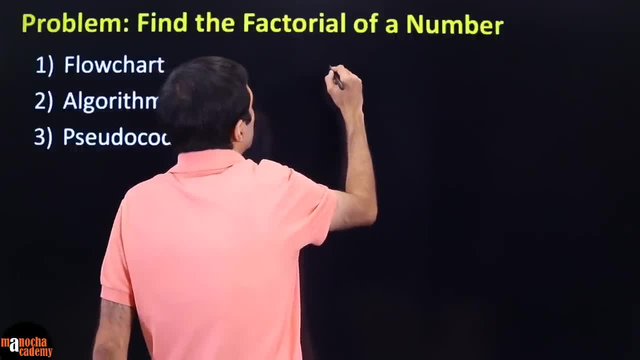 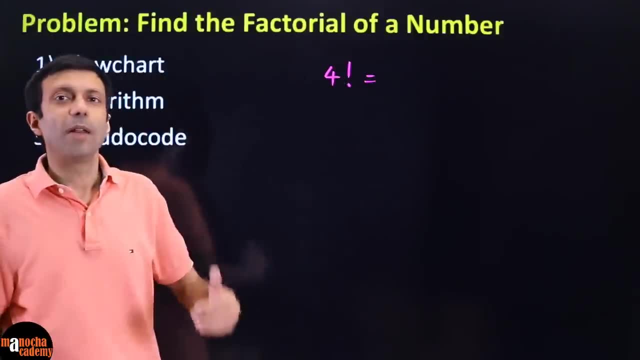 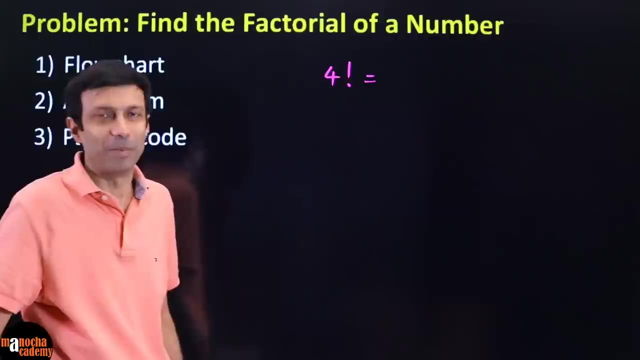 So how do we represent it? Factorial of a number, Let's say four. factorial is represented as four exclamation, And it basically means one Multiplied by two, multiplied by three, multiplied by four. So you multiply all the numbers till that number. 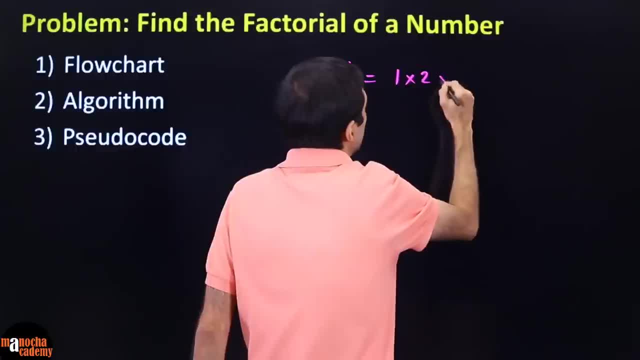 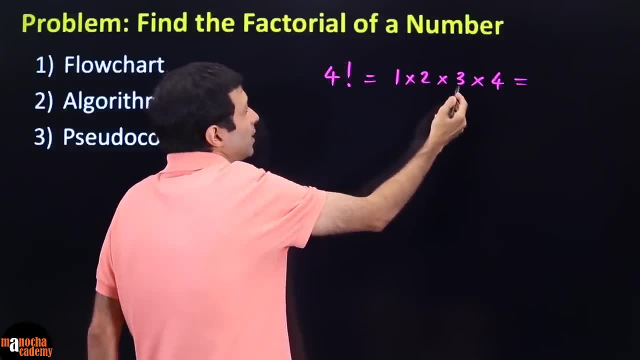 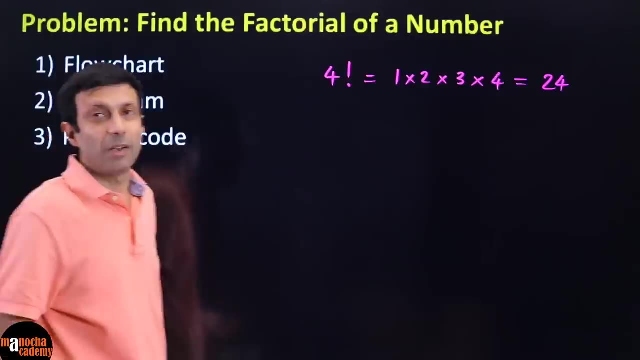 So four factorial is basically one times two times three times four. So what is the answer going to be? One times two is two. Two times three is six. Six times four is twenty-four. So four factorial is twenty-four. Similarly, what is five factorial? 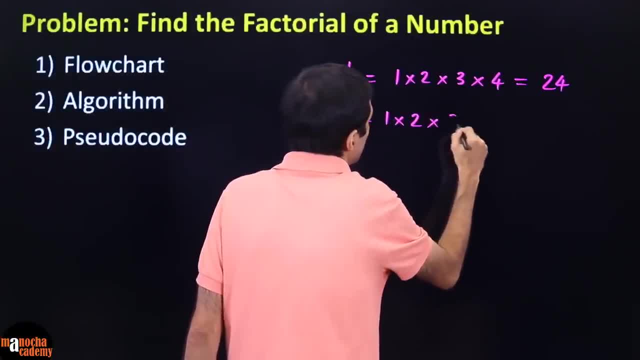 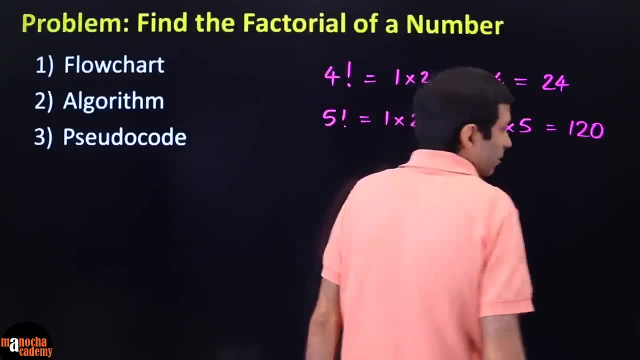 Five factorial is going to be one times two times three. Five factorial is going to be one times two times three times four times five. So this is going to be one hundred and twenty. Please multiply and check. This is the meaning of factorial. 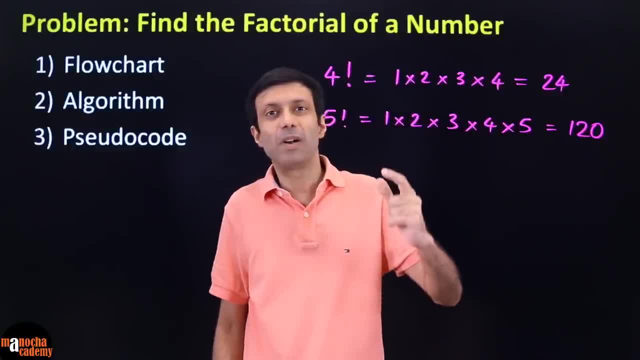 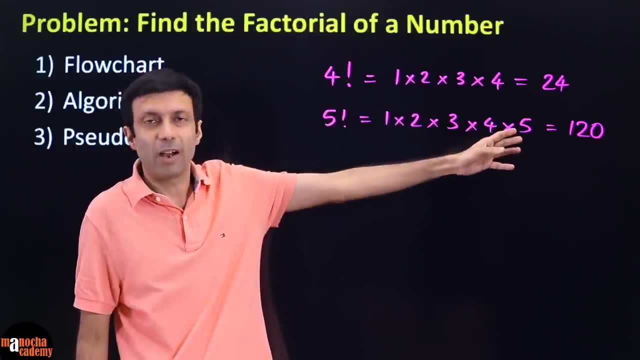 So if anybody asks you now what is factorial of a number, You know you keep multiplying the number till you reach it And obviously you can see the numbers become big because you're multiplying. So five factorial is pretty large. One hundred and twenty. 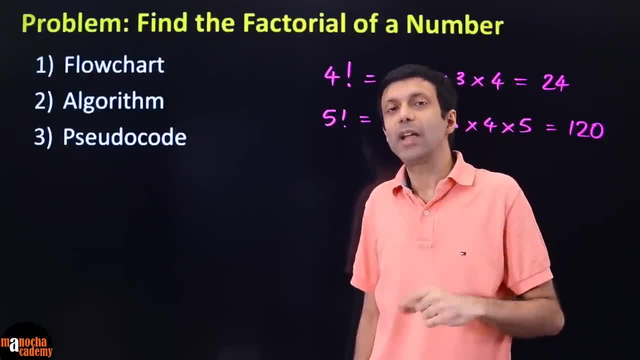 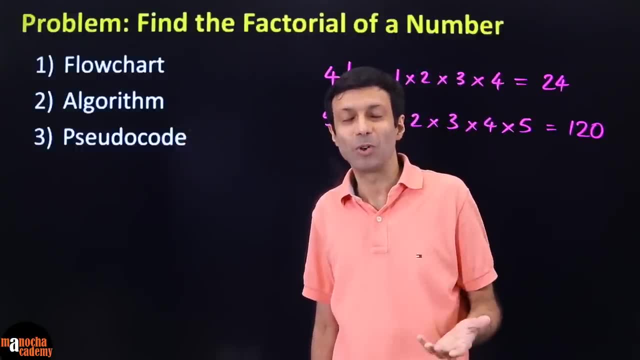 So let's see How will you write a program To find factorial of a number. obviously you input the number from the user. So let's start off with using flowcharts to think about the logic. So what is the first thing in flowchart? 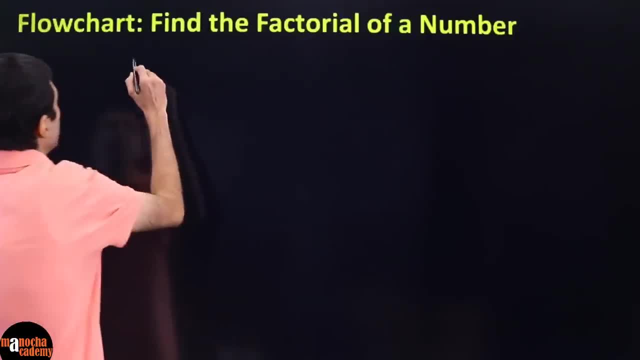 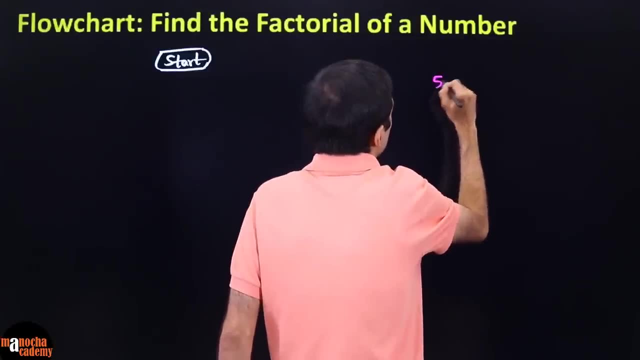 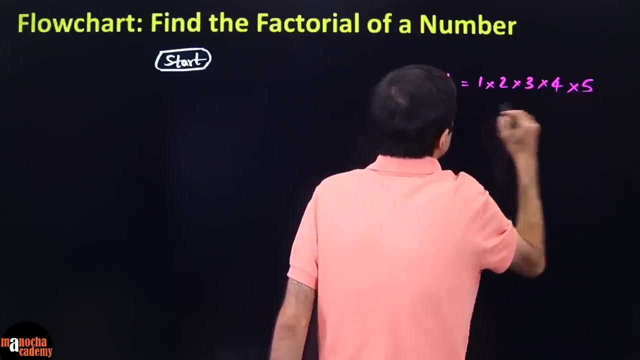 Obviously we will start with start, So we simply write start here, And let's keep this example on the side. So five factorial is one times two times three times four times five, Which is basically one times two. So that you guys remember this example. 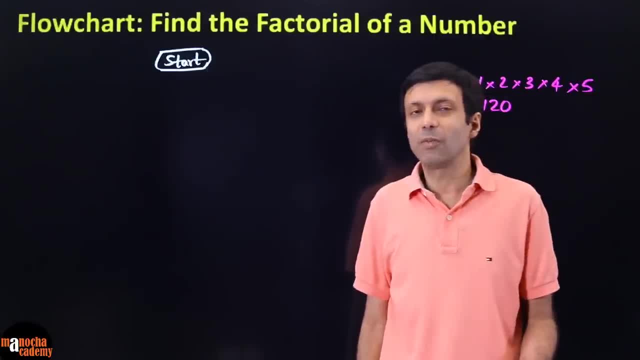 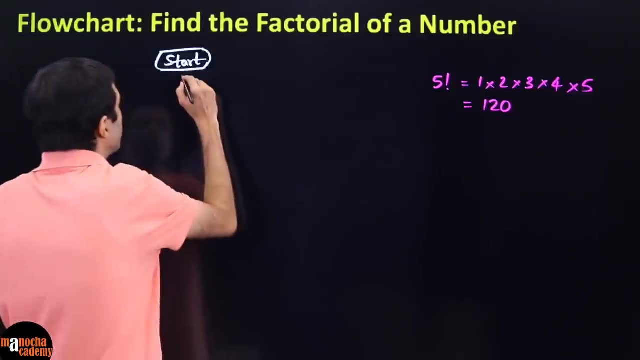 So first we do start, Then the next thing will be to input the number whose factorial we want to find. Let's call that number n. So the next step in the flowchart will be to input n. So here, for example, I am using capital letters for variable. 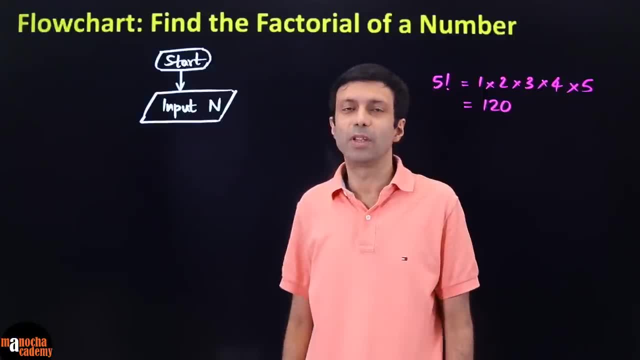 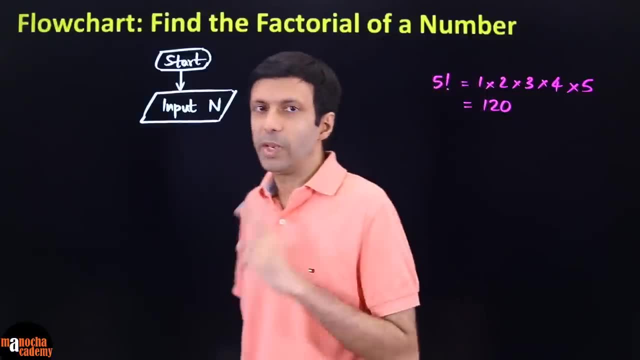 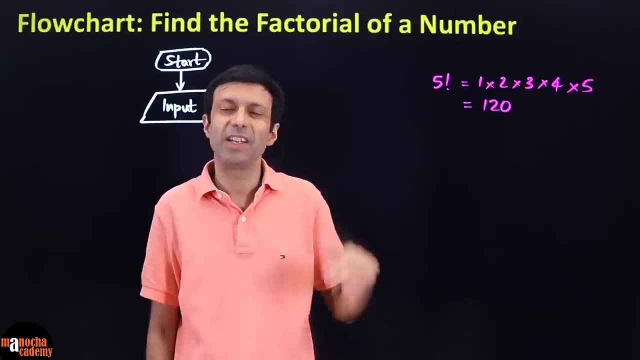 Doesn't matter, Whatever you want. So we are going to input the number n. Now, once we have input the number n, what do we need to do? We need to multiply all the numbers from one to n. Yes, One times, two times, three times four. 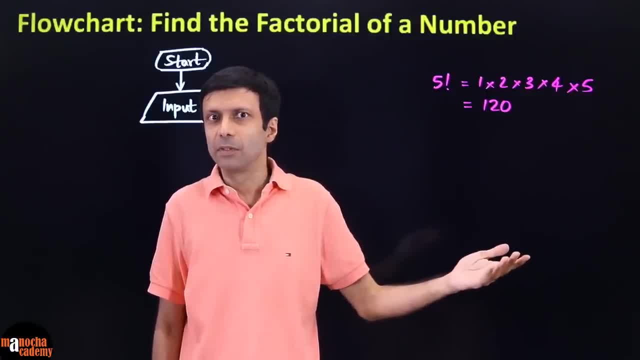 And keep on going till n. So how do we keep on going? Because we need to start from one. That means we need another variable to keep as a counter. Do you guys agree? So basically we can think of: we need a variable, let's say i. 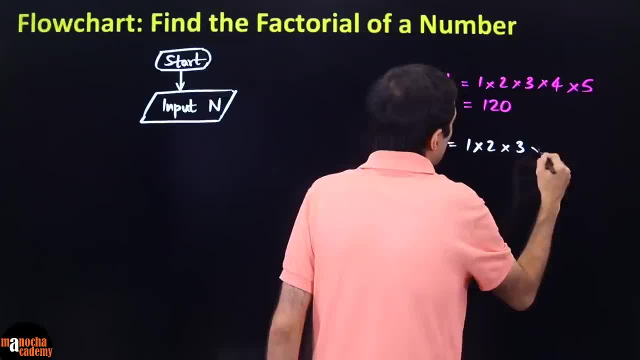 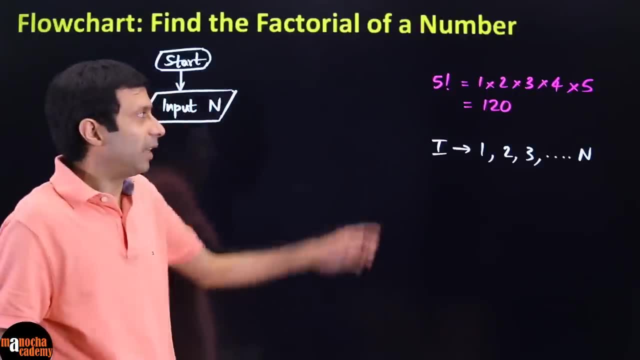 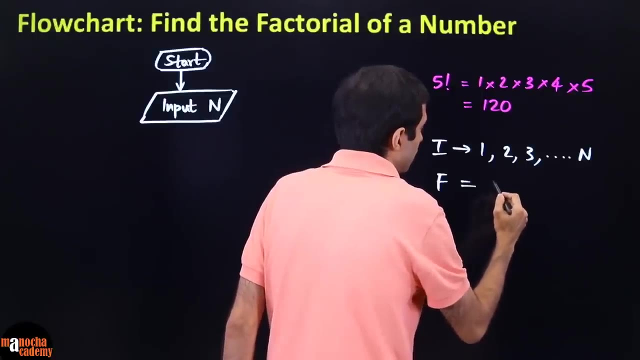 Which goes from one, two, three, All the way till n. So this i is basically changing, Yes, And then we are storing that multiplication, let's say in the factorial of the number which we can call as f. This stores the factorial. 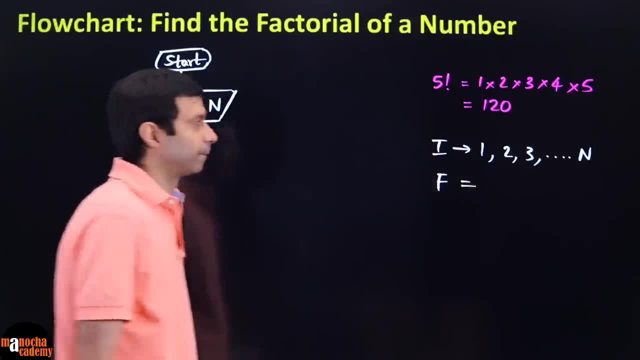 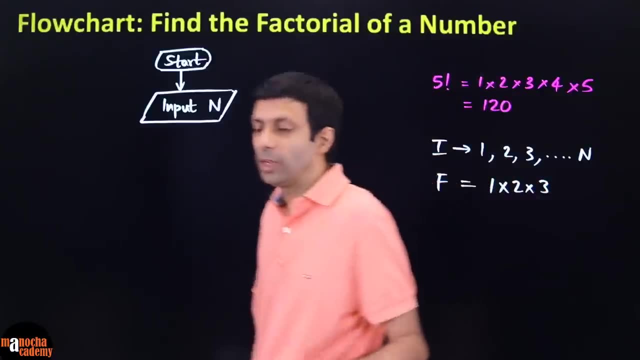 So when you are multiplying the number, it keeps storing that. For example, if you have multiplied till three, it stores it till here. Yes, So after we do the input, what is the next step? We are going to create these variables. 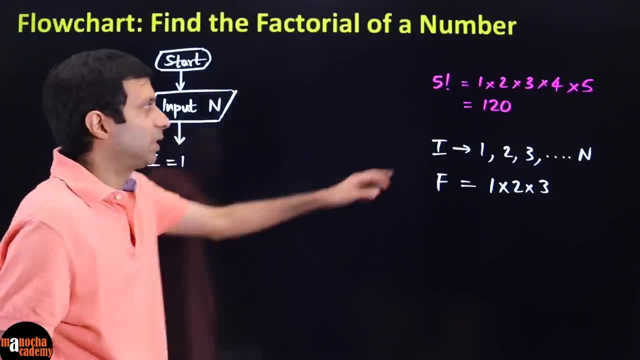 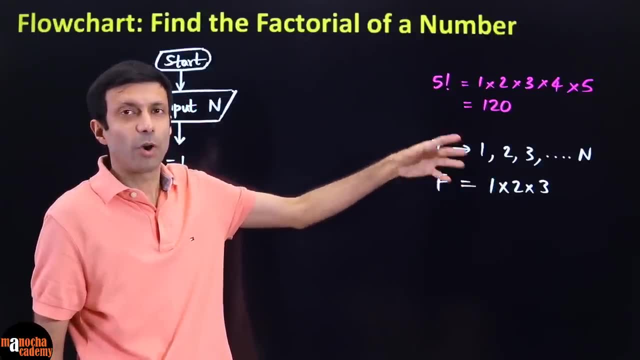 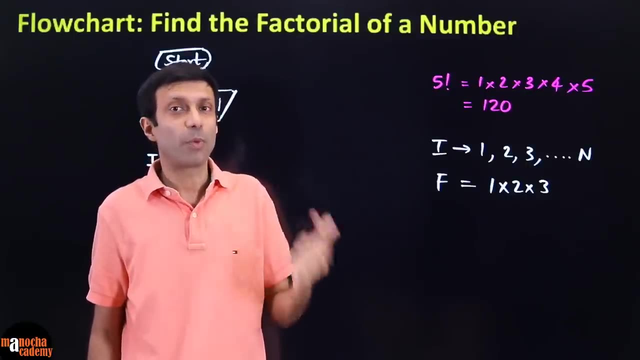 i is one, Because we start from one And this factorial which is going to save the factorial, Since we are doing a product. just like, if you want to find sum of numbers, what does the sum start off with Zero? But now we are doing a product. 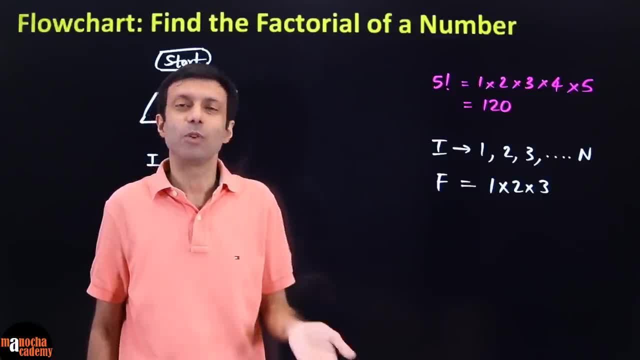 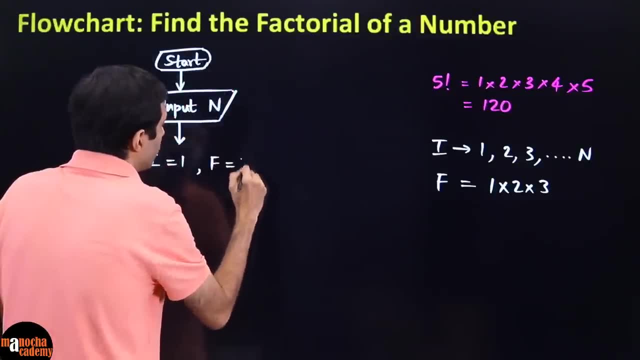 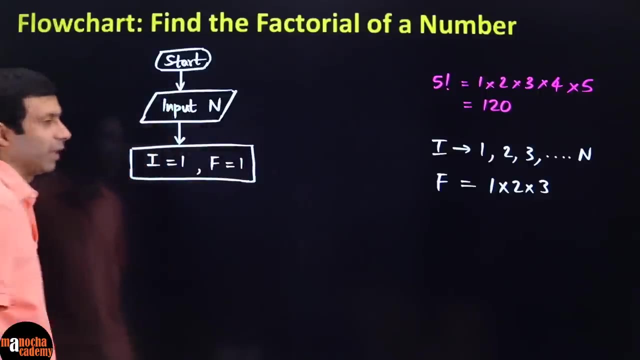 If you start off with the initial value of zero, whatever you multiply is going to be zero, So be careful here. So our other variable, f, will also be one. So this is our processing box, because we have not taken these as input. These are the computer variables. 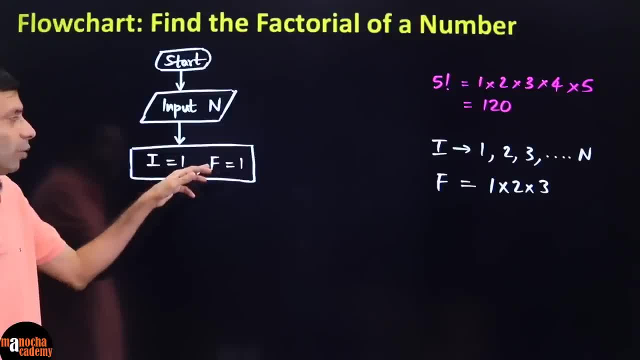 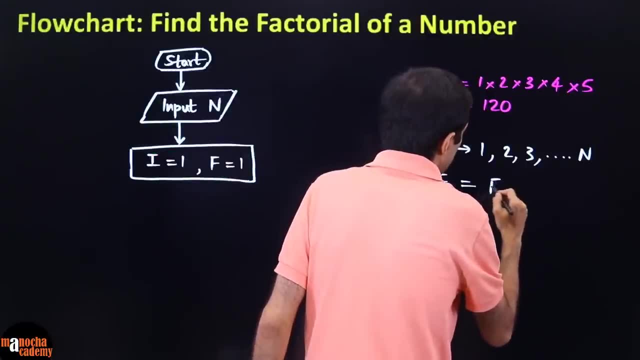 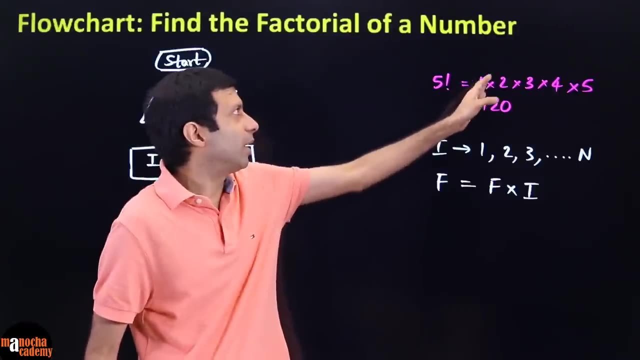 Now what is the next thing you will do here? So to calculate the factorial. what will be the formula? The factorial is basically the current factorial times. the next number i, If you look at the logic here, suppose you are doing one times two times three. 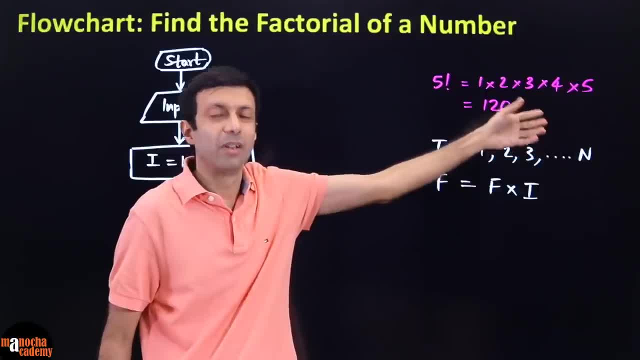 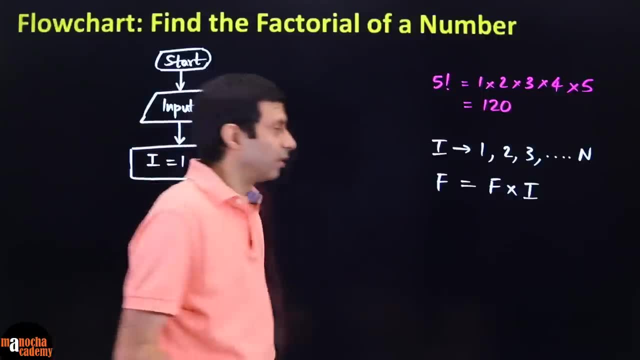 So you keep stored that in f, Then you multiply it by four, Then again you store that in f, Multiply it by five. So can you see the formula? just like sum equals sum plus i, Let's say you want to find the sum of numbers. 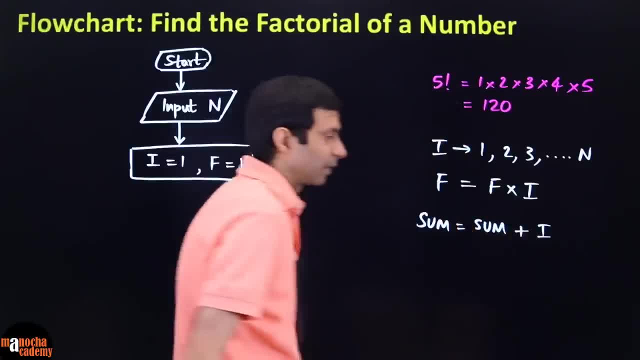 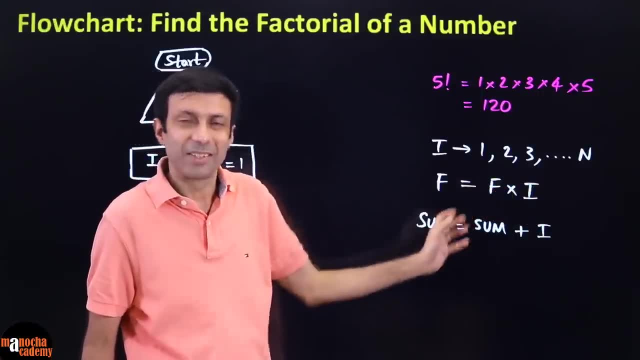 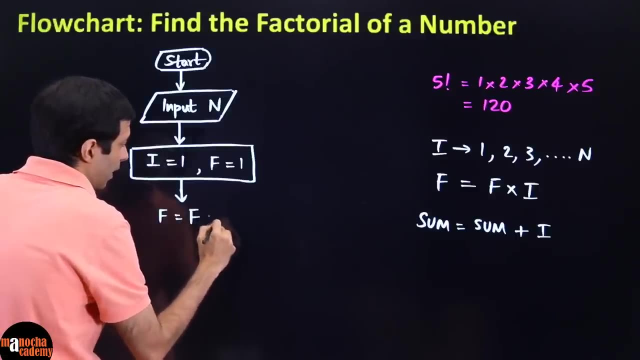 Just like sum equals sum plus i. This is to find the sum of different numbers, To find the product. what will you do? f equals f times i. Same logic here. So what we are going to do over here: f equals f multiplied by i. 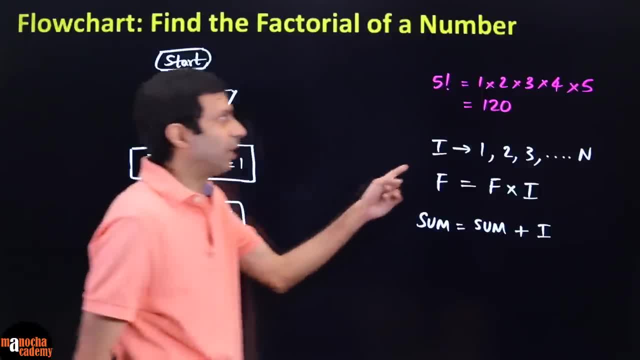 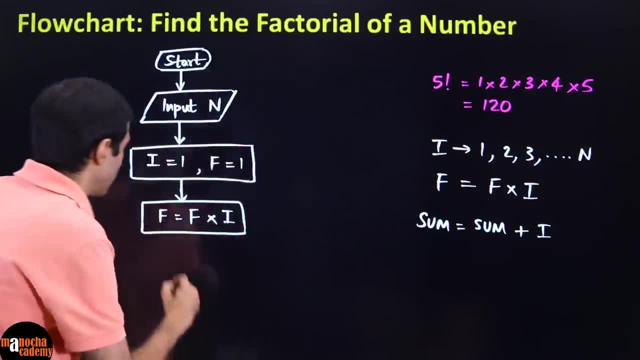 But now what is the next step? You need to keep on increasing the value of i- One, two, three, four, five. So i just started off with one. So what is the next thing we are going to do? We are going to say: i equals i plus one. 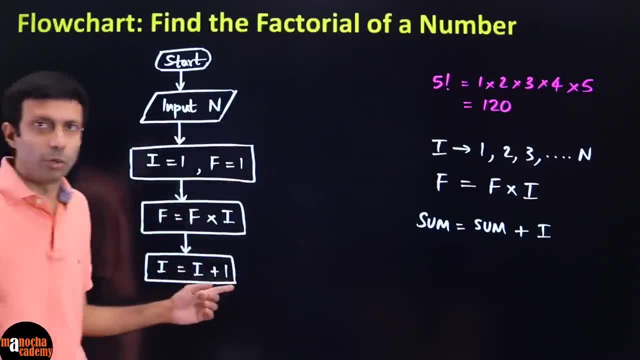 That means increase the value of i. Now, what do you do? So, once you have increased the value of i, you want to go back to the formula. You want to loop back and go here And go here And keep doing this. 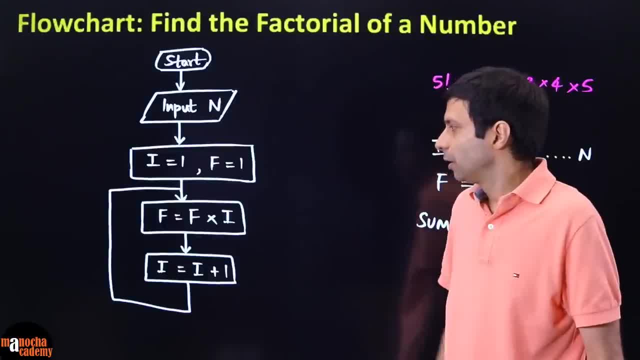 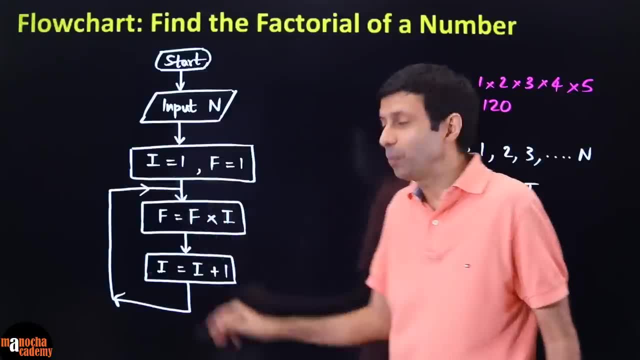 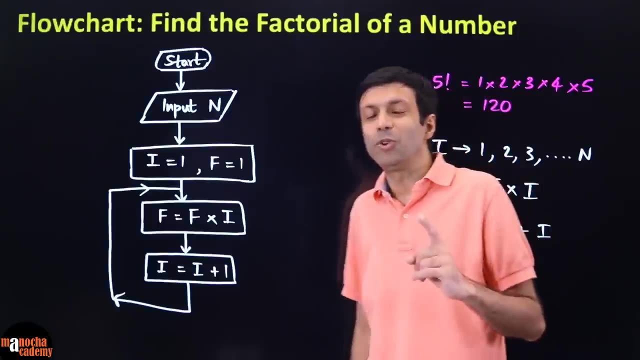 But if this is your logic, the problem is you are never stopping. Can you see? You are in an infinite loop here. You are not stopping. based on the value of i. When should you stop? When you have reached n, Because you need to do the multiplication one, two, three, four, five till n. 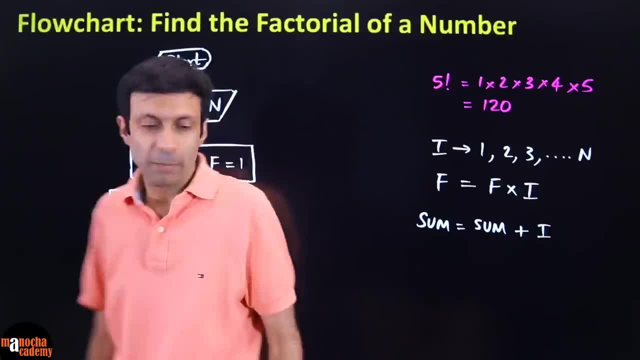 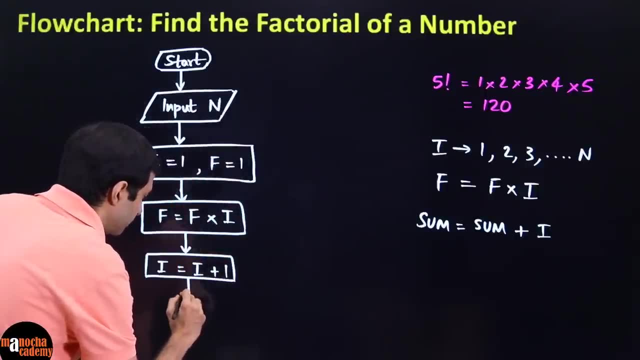 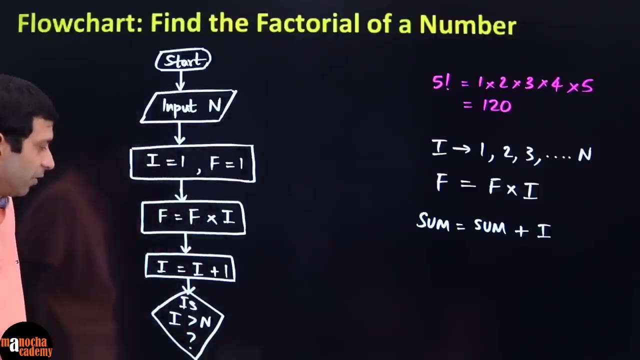 So you need to ask yourself the question. You cannot simply loop back here. We need to ask ourselves the question: After increasing i, is i greater than n? So ask yourself this question: Is it greater than n? If the answer is yes or if the answer is no, then you simply loop back. 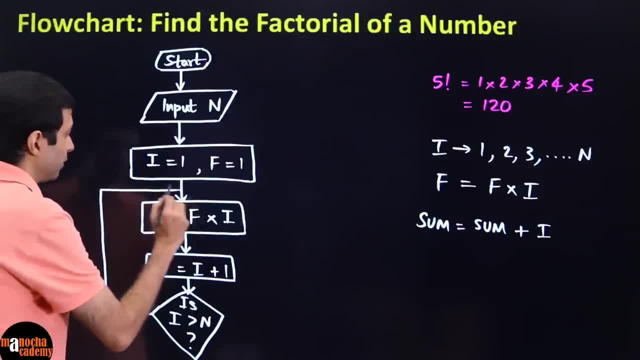 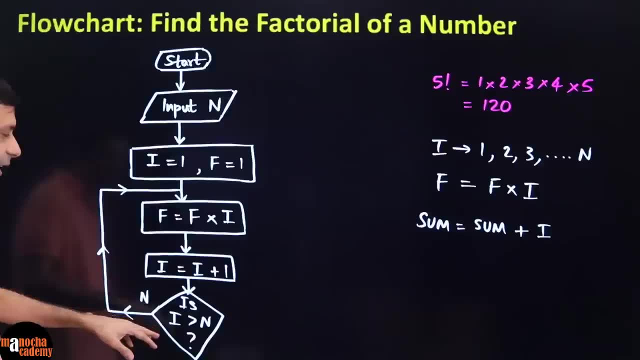 So you are allowed to go back and continue this multiplication. So if your answer is no, you are going to do this, But if your answer is yes- i am greater than n- then what happens? You will simply come out right. 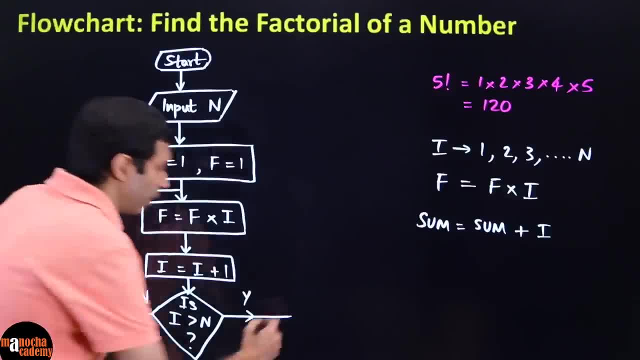 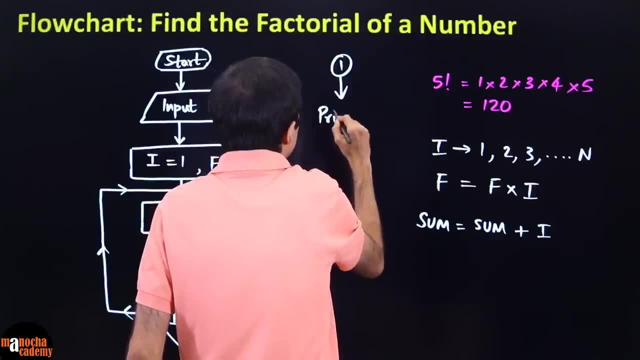 You will come out of this loop And see, since I have run out of space, maybe I can use a connector here. So I can call this connector 1.. And finally, we will print the value of the factorial f which is stored in the variable f. 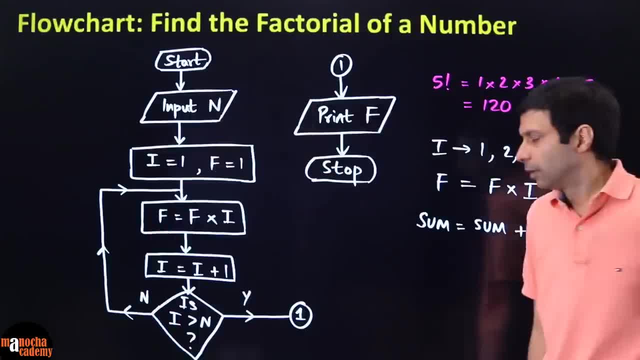 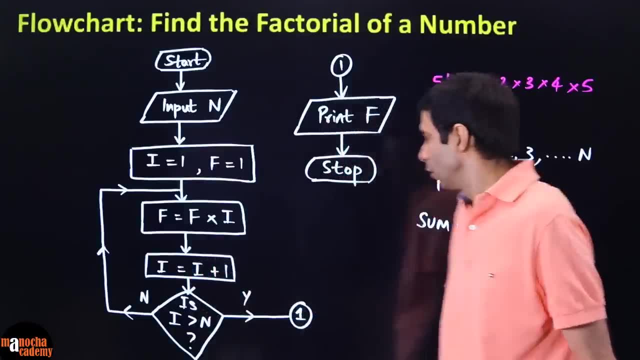 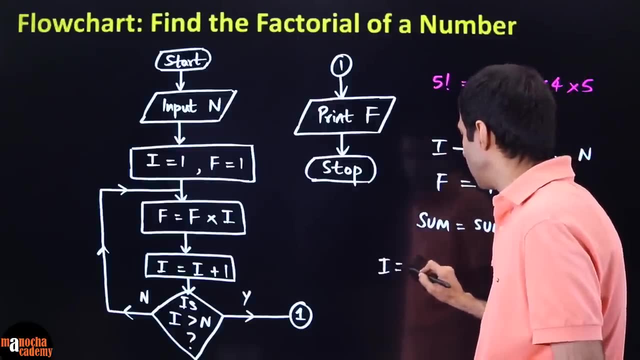 And then we will end the program. See, I am checking. i should continue to be n, right? So let's check if our flowchart is correct. So, for example, let's do a dry run here and see this. So let's say we have, we start off with i equal to 1.. 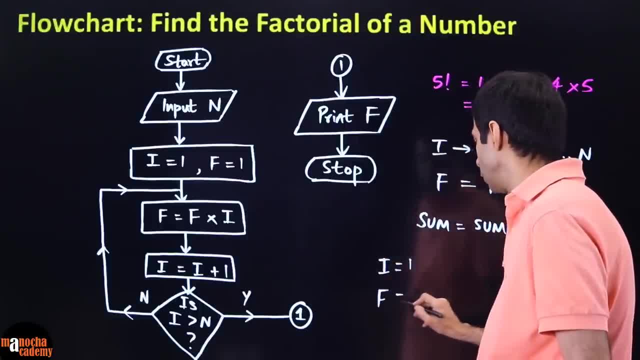 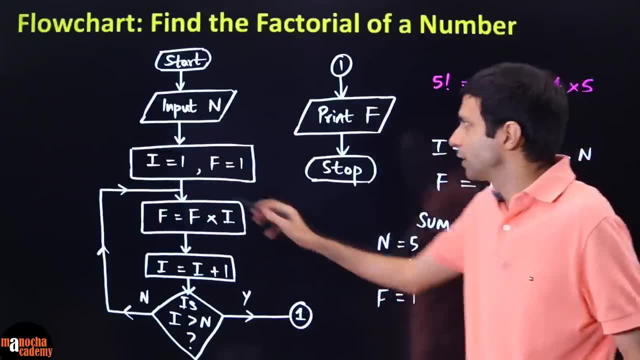 And factorial f is also 1.. So then what happens? And let's say the input number is 5.. So first time, what is going to happen? f equals f times i, So 1 times 1, it remains 1.. 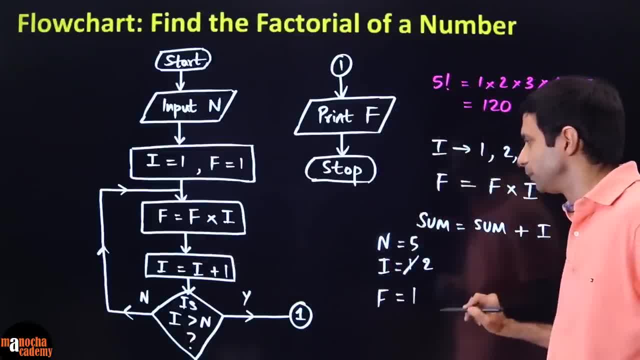 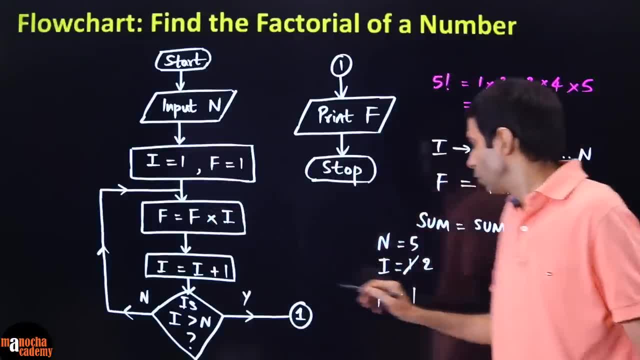 Next time i equals i plus 1.. i becomes 2.. So it asks the question: is 2 greater than n, which is 5?? The answer is no, It goes back. So now the factorial becomes factorial times i. So 1 times 2, factorial becomes 2.. 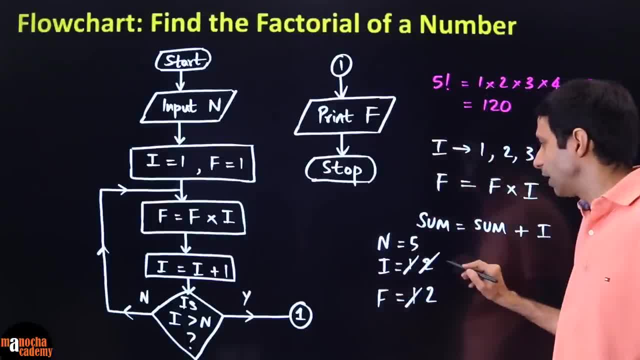 Then again we do: i equals i plus 1.. i becomes 3.. Again we ask the question: is 3 greater than n? No, We loop back. So factorial becomes 2 times i, 2 times 3, 6.. 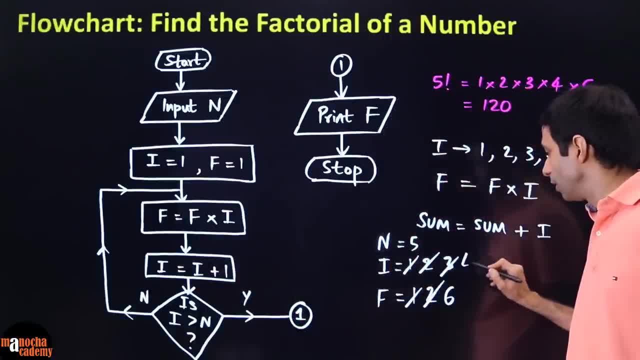 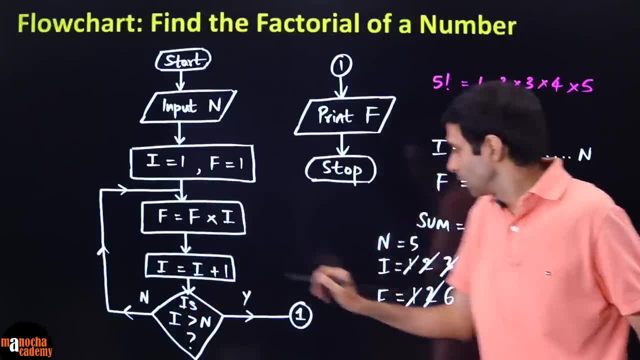 Again we do. i equals, i plus 1. i becomes 4.. Again, 4 is not greater than 5.. So we loop back. Factorial is factorial times i. So what do we do? 6 times 4, 24.. 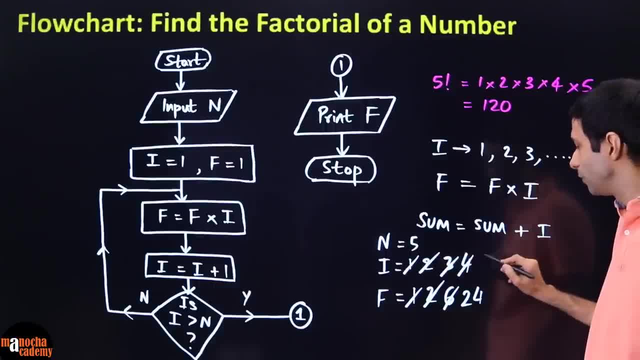 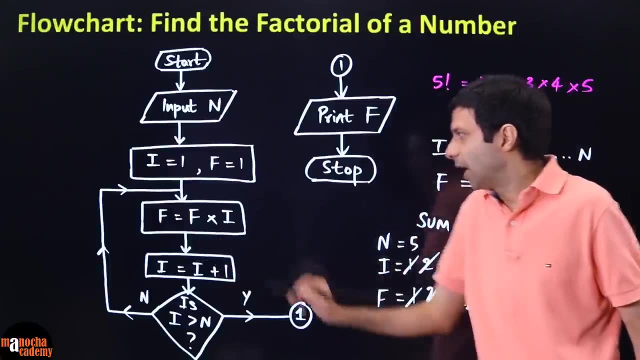 i equals i plus 1.. i becomes 5.. Again we ask the question: is 5 greater than 5? No, So we go back. Factorial is factorial times i, 24 times 5, 120.. Again it says: i equals i plus 1.. 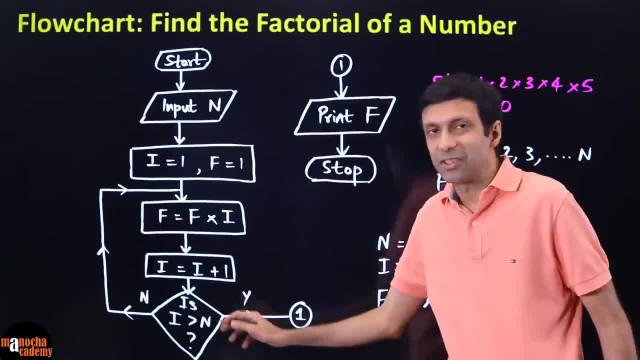 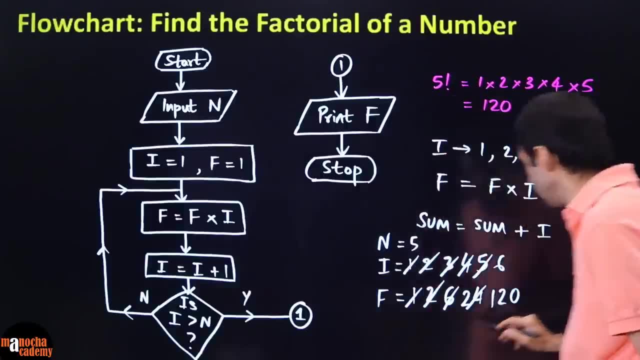 i becomes 6.. This time 6 is greater than 5.. So it will come out. It prints the last value of the factorial, which is 120.. As you can see, 120 is the value here That will get printed out. 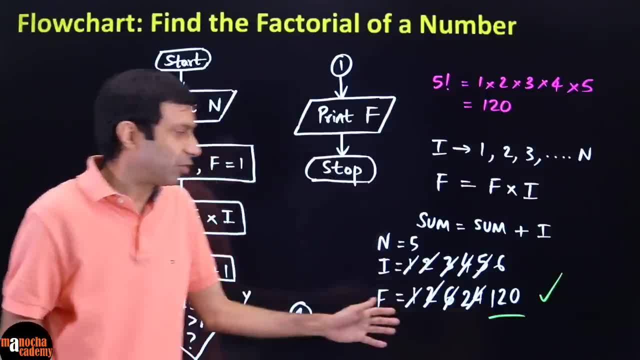 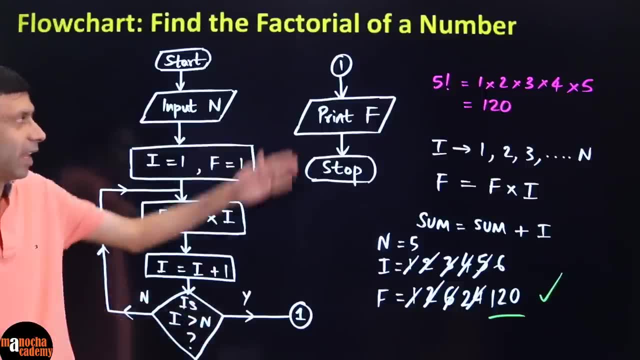 And then we stop. So can you see, we did our test run And it worked out perfectly. So your condition is very important. You need to check: is it greater than n? Then only we stop. If it's equal to n, we let it go. 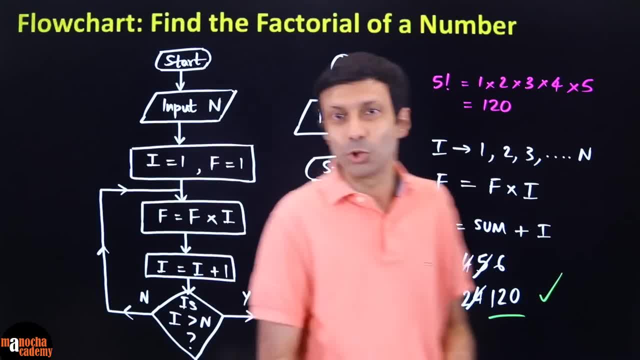 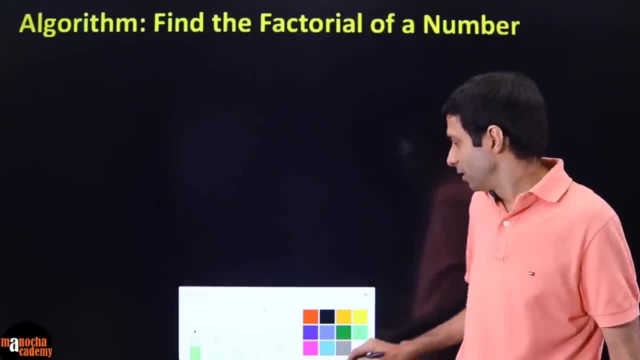 Because we want that multiplied here. So is this flow chart clear to you guys Now? similarly, if you have to write the algorithm for finding the factorial, So how do you guys do it? Again, this is step by step, So we will write down the steps here. 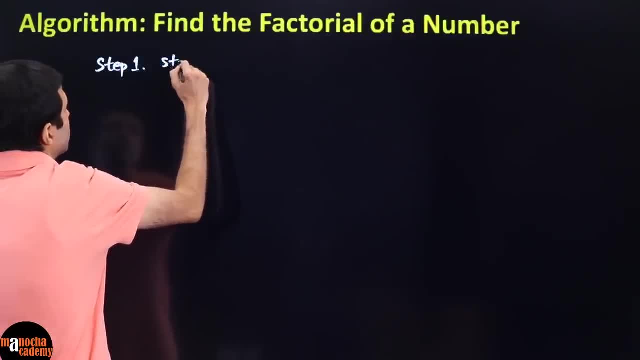 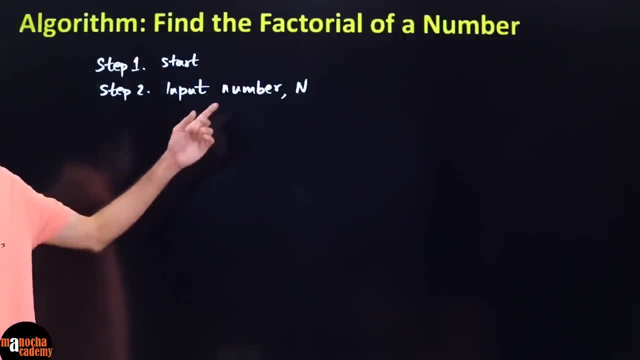 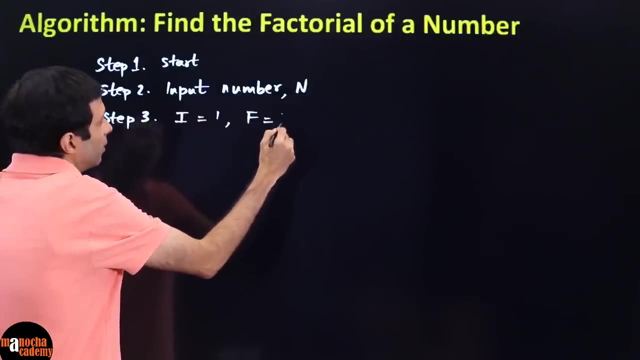 For example, step 1, start. Step 2 is input your number whose factorial you want to find Step 3, you assign these values: i equal to 1, f equal to 1.. If you want, you can break this down into two steps. 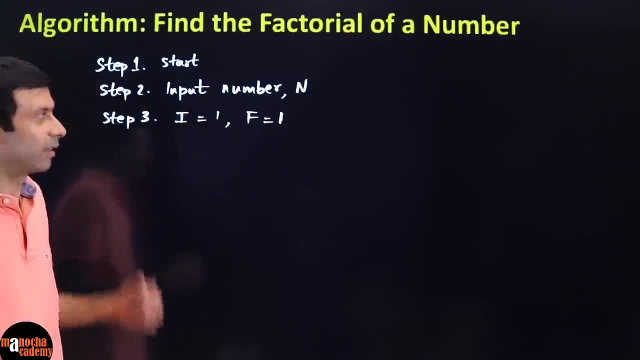 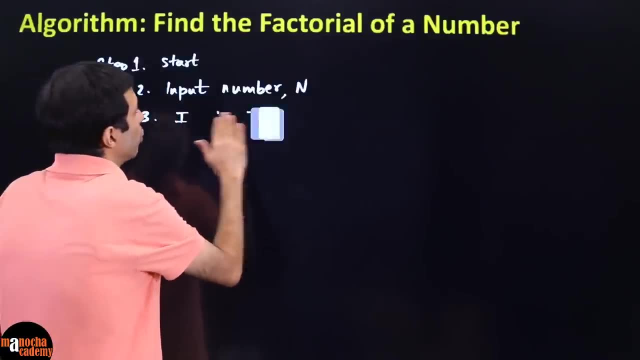 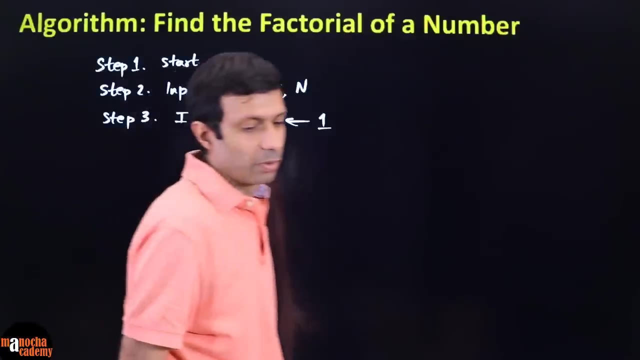 Where you are doing this: initial assignments. Okay, Sometimes we said, when we are showing assignments in this algorithm, we tend to show it will The arrow. So whichever style you want to follow, Then what is the next thing we need to do? 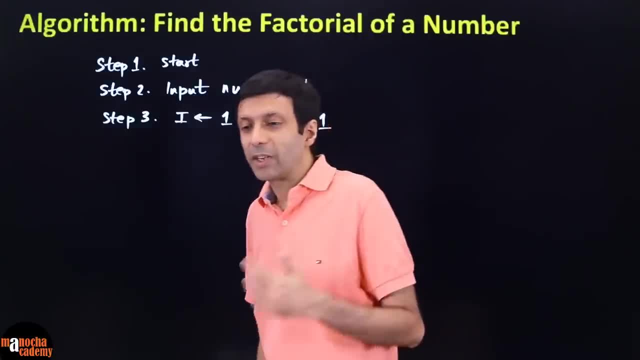 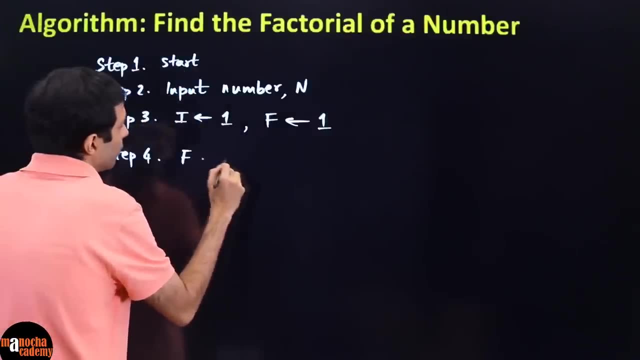 Now we need to write the formula to find the factorial. Factorial is you multiply the current value with the next i. So we are going to write the formula. Step 4, factorial f is f, the current factorial multiplied by the next number, i. 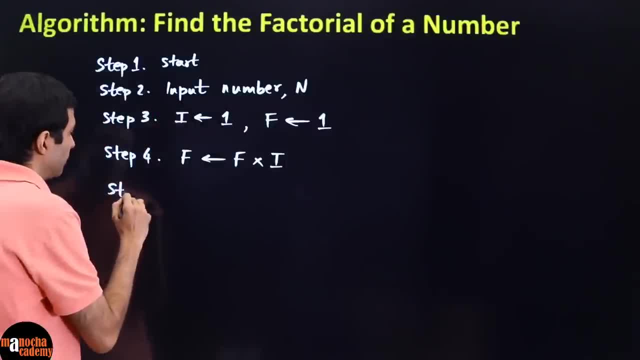 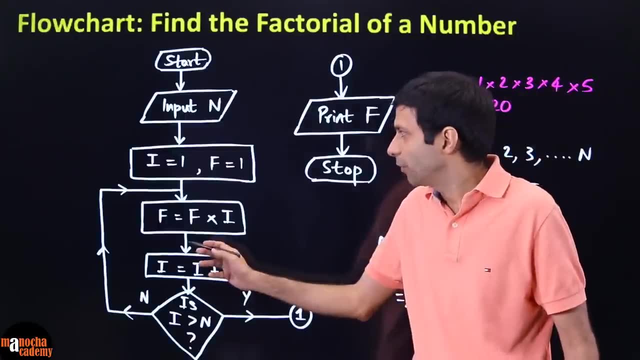 So we did that. Next step will be to increase the value of f. Yes, Or another thing we could have done is we could have checked the value before increasing it. So depends on how you are writing the loop. So here we can do. 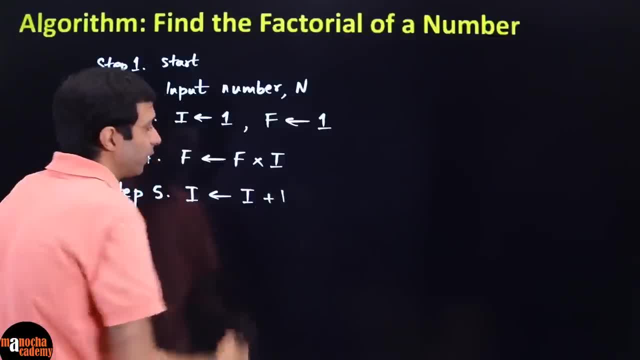 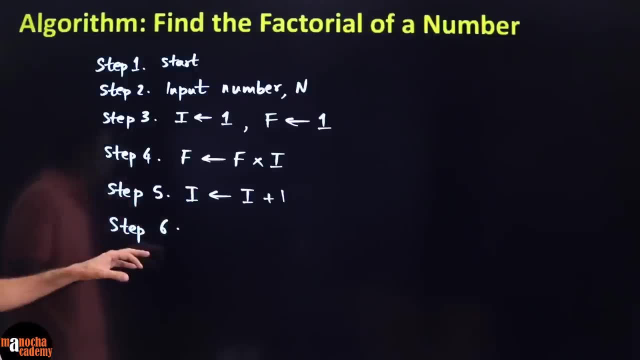 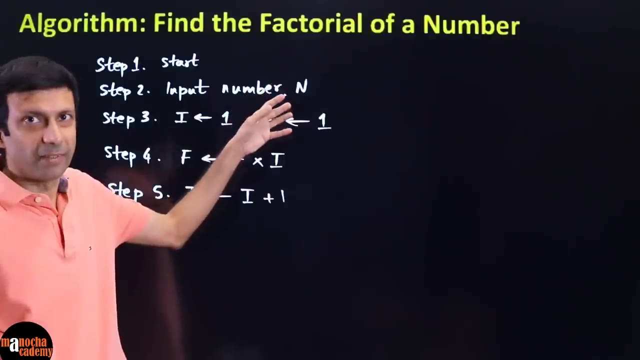 i equals i plus 1, which means increase the value of i And then put it back in i. Now what will step 6 be, As long as your value of i is less than or equal to n? So what can we say here? 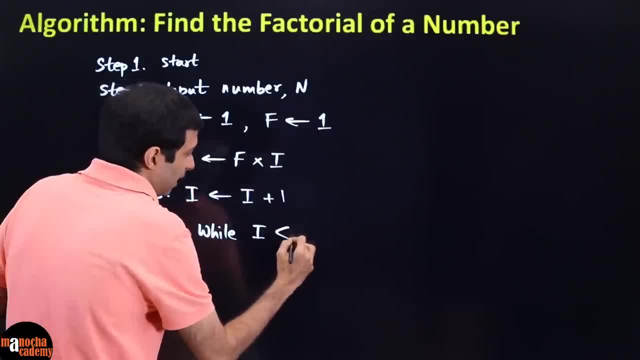 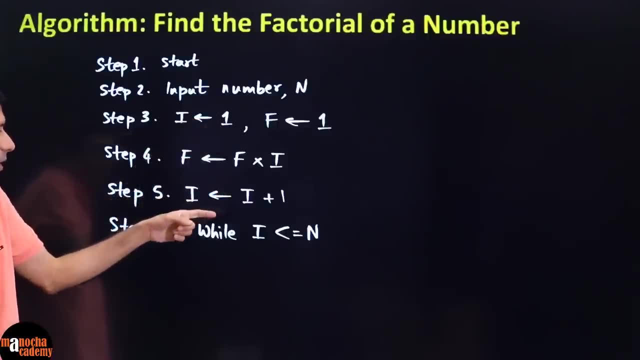 While i is less than or equal to n, you need to keep repeating these steps, right? So as long as i is less than or equal to n, you repeat steps 4 to 5.. Or 4,, 5,, 6, right. 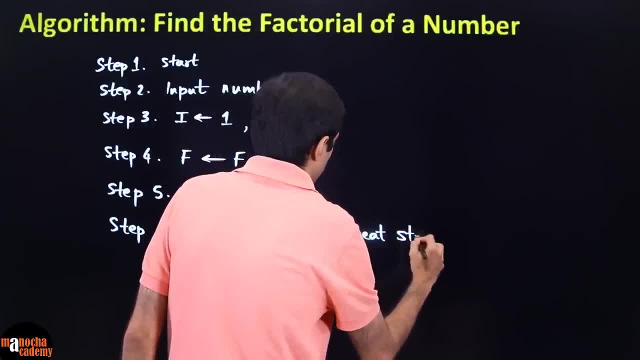 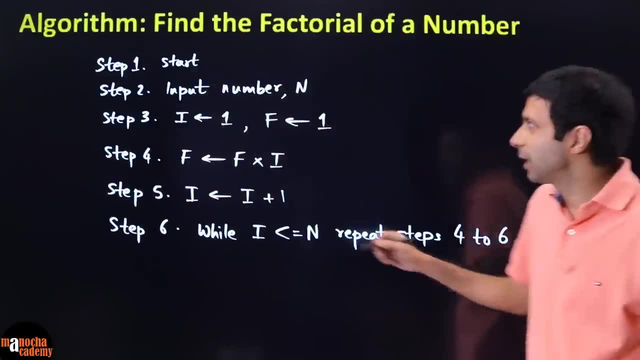 So, while i is less than or equal to n, repeat your steps 4,, 5 and 6.. So see, algorithm helps us to tell which steps to repeat This: multiplication step, increment step and again the checking step. So keep doing this. 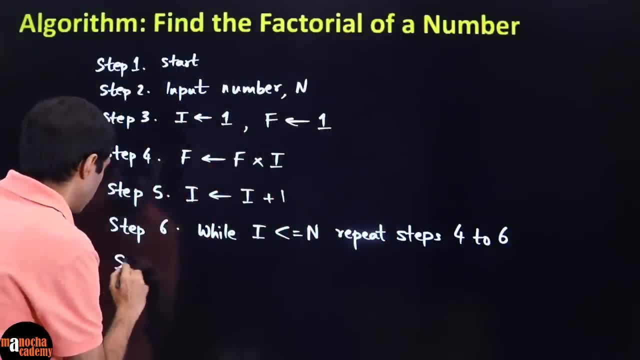 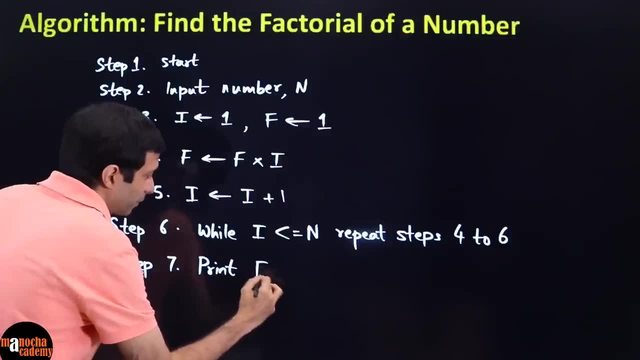 And then, once it is more than n, obviously you will come out, And please don't forget to print the value of the factorial. So we will print out f And step 8 is stop. So there you can see. we have written the algorithm of the same program. 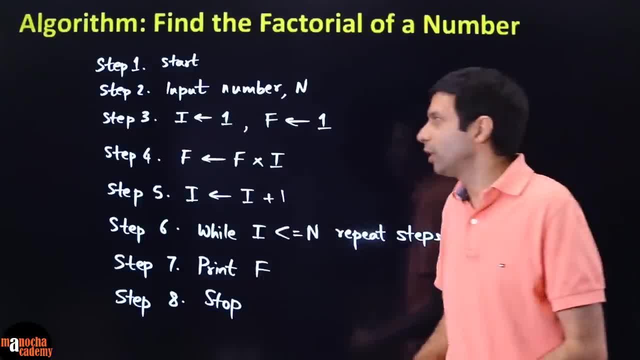 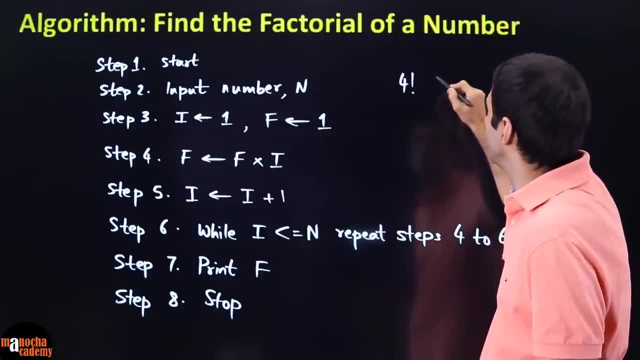 the whole logic is. so the whole trick in factorial is you keep multiplying the number with the next i. So, just like you know, when you are finding 4 factorial, what do you do? 1 times 2, see times the next number. 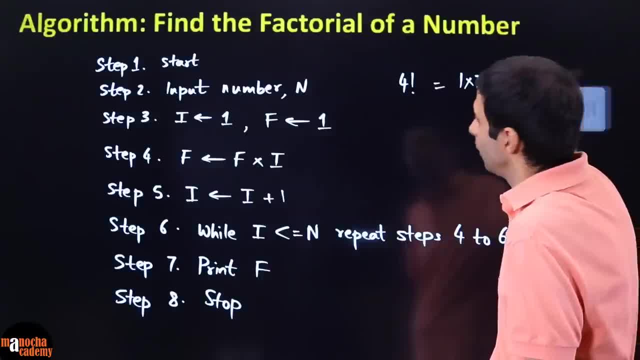 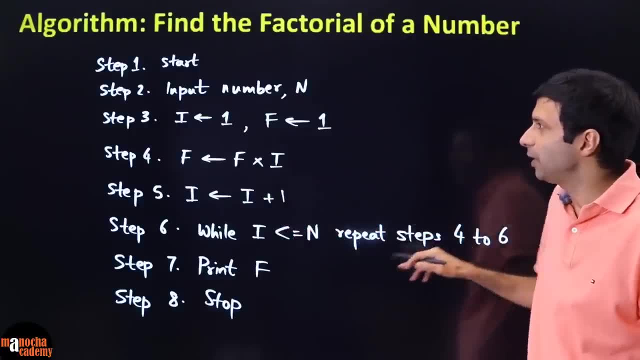 3 times the next number, 4.. So same logic here. you keep multiplying it with the next number, keep incrementing your i and do this. repeat these steps 4, 5 and 6, as long as your i is less than or equal to n. 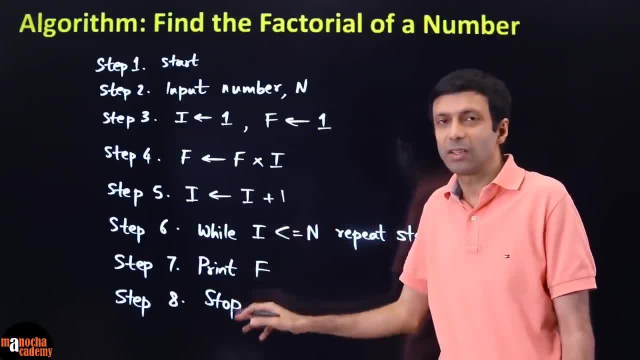 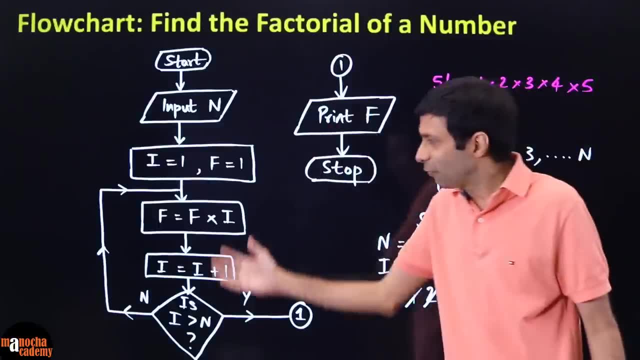 The moment i becomes bigger, you print out the thing and you end the program. This is how you write the algorithm. So yes, I think many of you might be thinking flow chart is easier. definitely because it is a graphical. 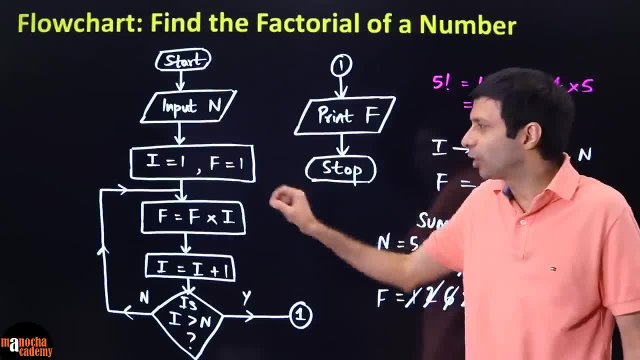 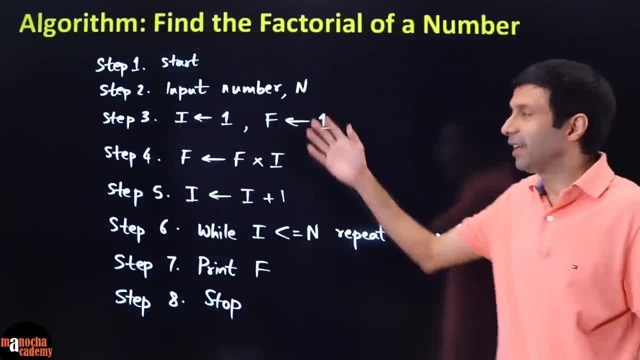 pictorial representation. but the problem is, you know you have to draw these boxes, all these arrows, so it is little more time consuming but definitely more visual than writing these steps. And last thing we are going to try is: 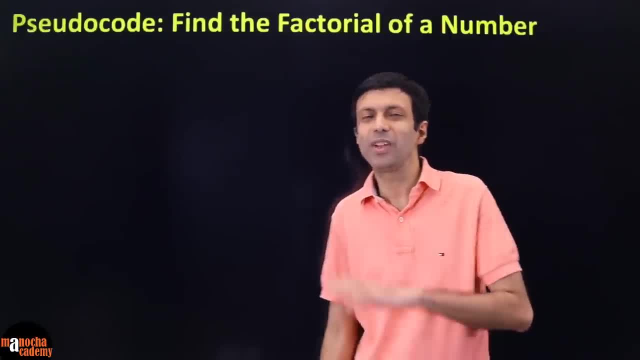 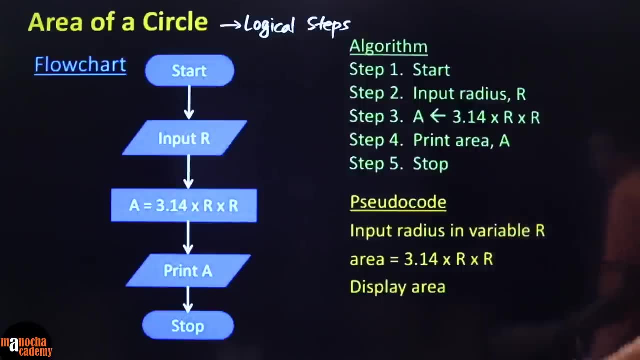 writing the pseudo code of the same question So that we are clear about all the styles and you can decide which style you like. So in pseudo code, remember what was it like? Pseudo code: looks like a program, right, Informal program. 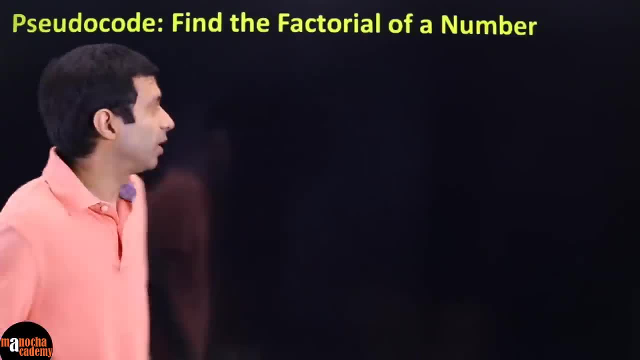 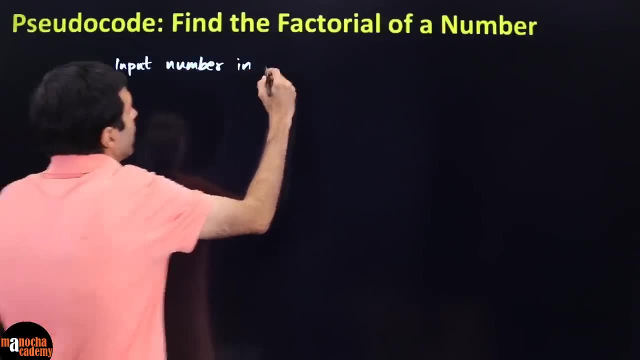 So let's go ahead and write that. So pseudo code of our factorial is going to look like. so what is the first thing you are going to do? Input number in variable n. again, you can use small or capital, depending on the convention. 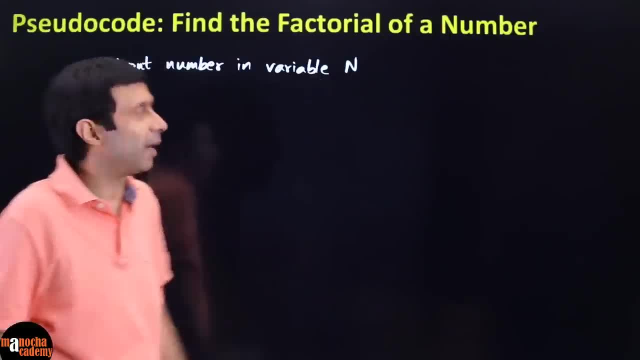 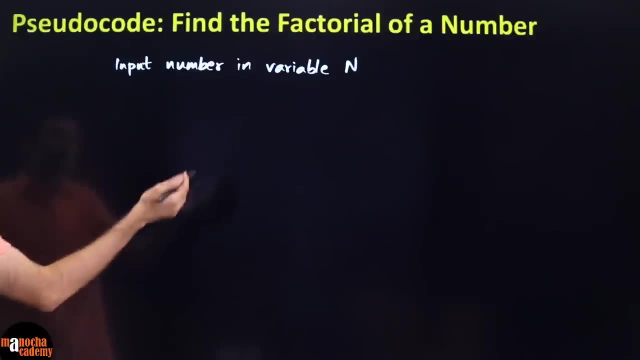 so here I am using capital, just to keep it consistent. so capital n is our number whose factorial we want to find. So what will be the next step? So we will of course assign the values here. we will say: i equals 1,. 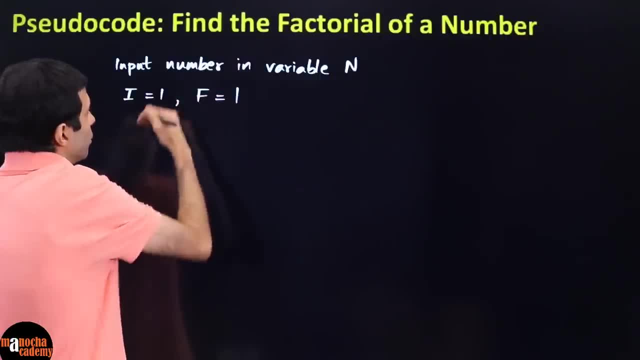 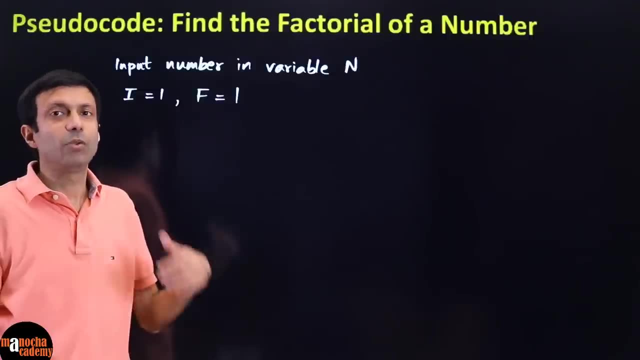 and our factorial is 1,. you can break this down into separate lines also, if you want. So what is the next thing you are going to do? So, basically, you need to do the check that, as long as i is less than n. 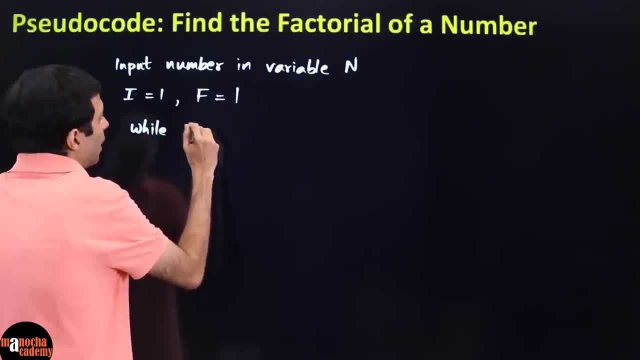 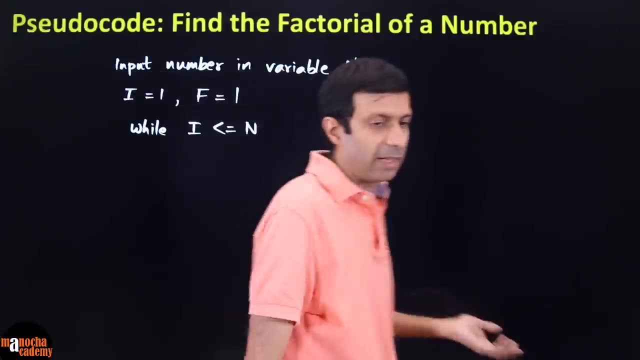 so you can say: while i is less than equal to n, so in this kind of style you might be thinking of writing the check first In flowchart. we wrote the check later, so it depends on your logic how you are writing it. 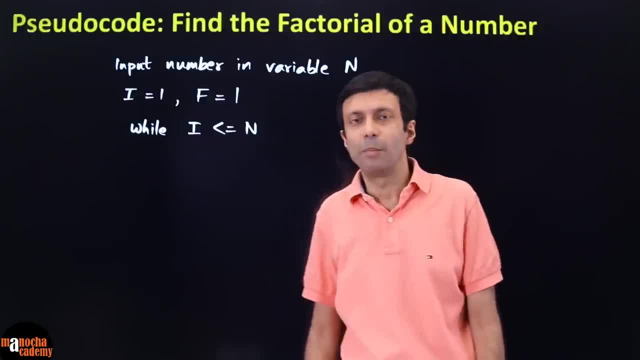 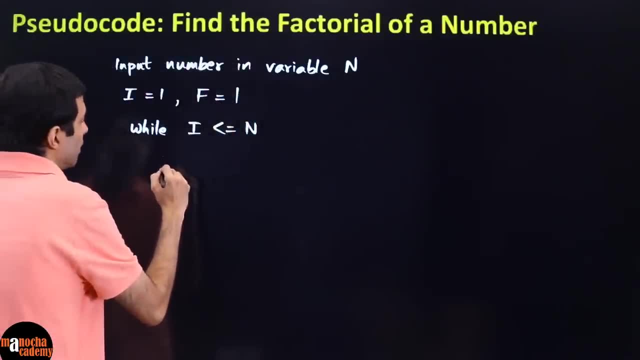 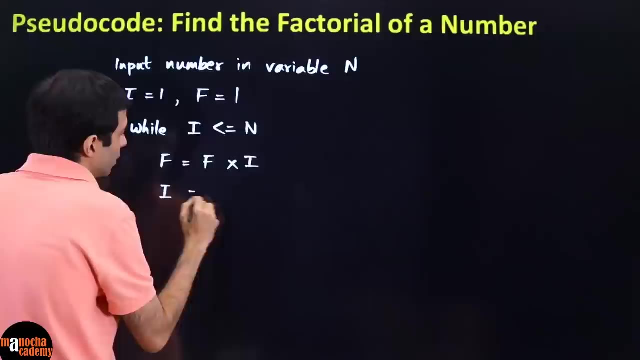 So here you are saying that your first checking is your number less than equal to n. As long as i is less than equal to n, you will continue doing this. So in the factorial you will multiply f equals f times i and i equals i plus 1.. 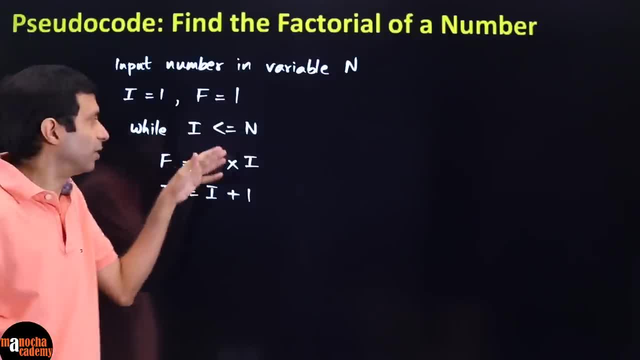 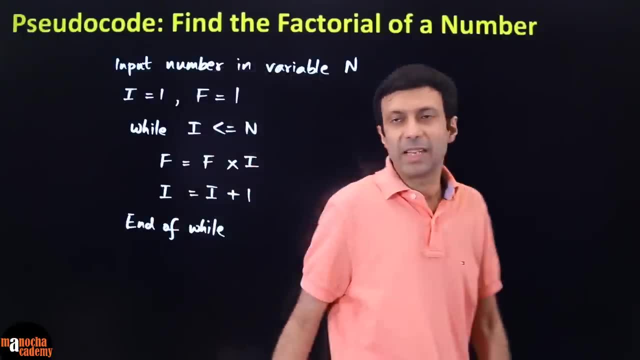 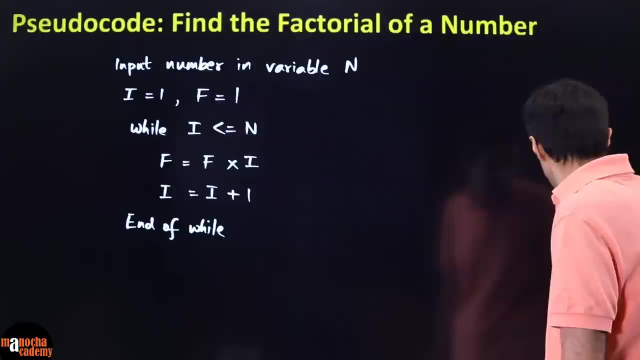 So these you are doing inside this while condition and sort of your while loop ends here so you can write end of while Again. this is informal style to show that this is where my condition or looping started. So you can see clearly there is a loop thing here. 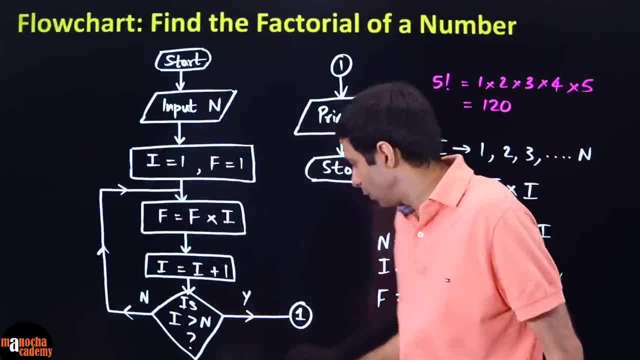 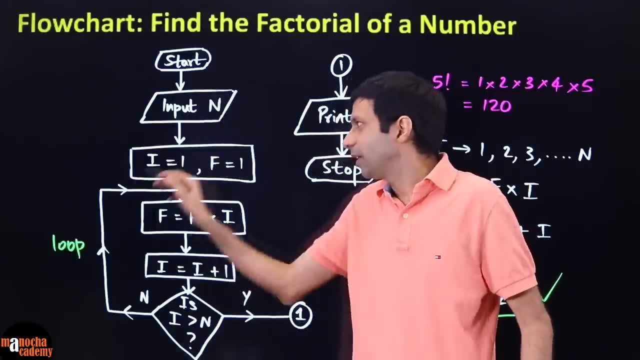 because you are repeatedly doing the steps. So can you guys see that we are in a loop, just like we say playing a song in a loop, repeatedly playing it, So repeatedly you are doing the steps, but it's not an infinite loop. 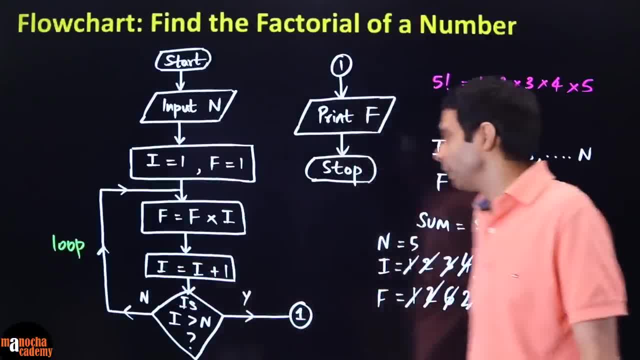 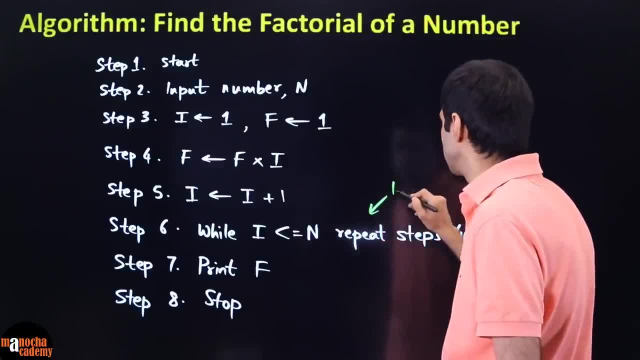 you are not going on and on. there is some condition here. Similarly, in the algorithm you can see there is a loop here, because we are saying: repeat the steps 4,, 5, 6, as long as this condition is true. 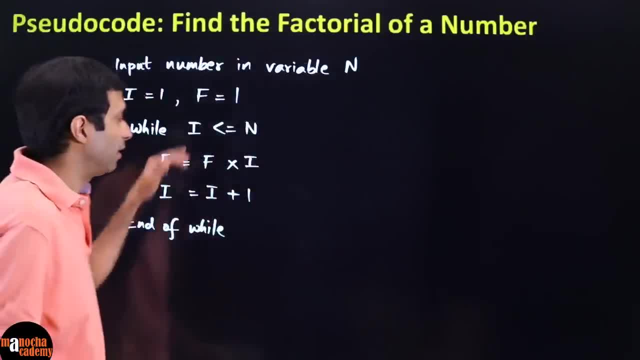 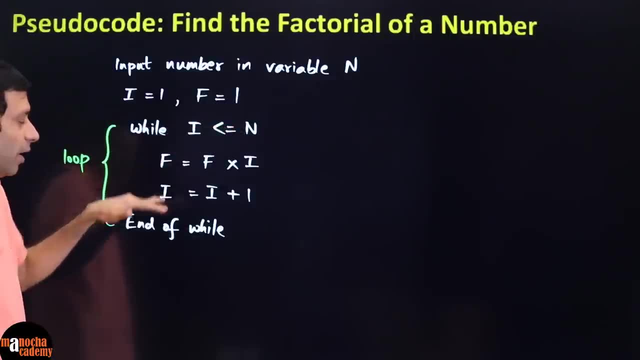 Same thing we are saying here. can you see, there is a while, there is a kind of a looping here going on. Keep doing this as long as i is less than equal to it, And then you come out of that. once you come out of your condition. 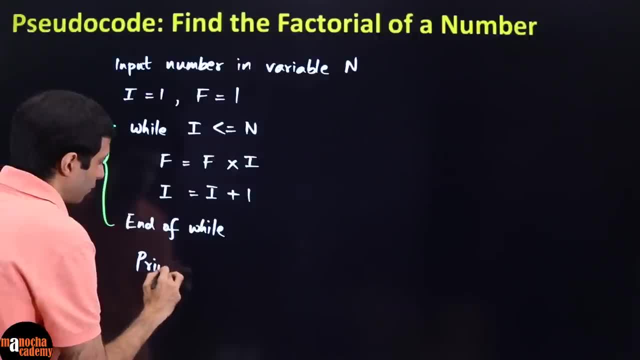 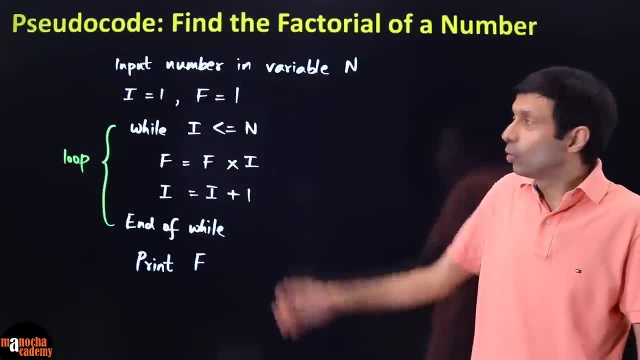 what will you do? You are going to display or print the value of- not i- the factorial f, and that's when you stop your program. So again, you can see, the nice part about this is: this is quick code, rough code. 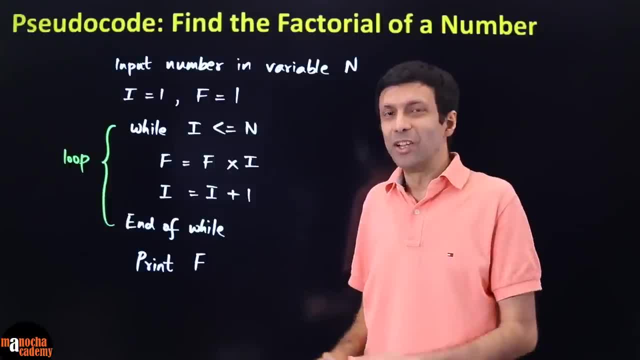 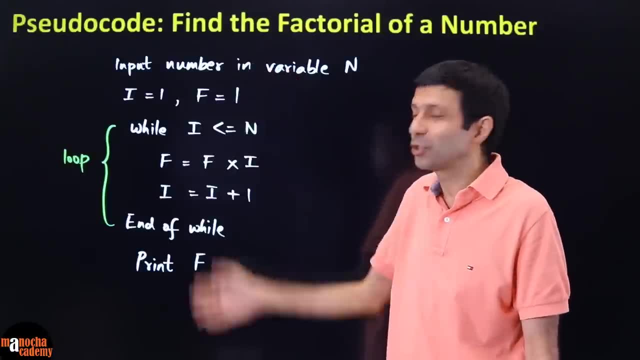 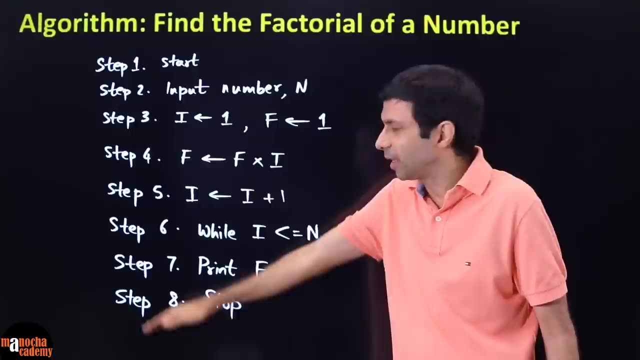 but it is very close to almost writing the code, So pseudo code. the advantage is you can quickly translate it into Java or Python code because you have almost written code Algorithm. the advantage is it is very clear, step by step. You have outlined all the steps in a systematic fashion. 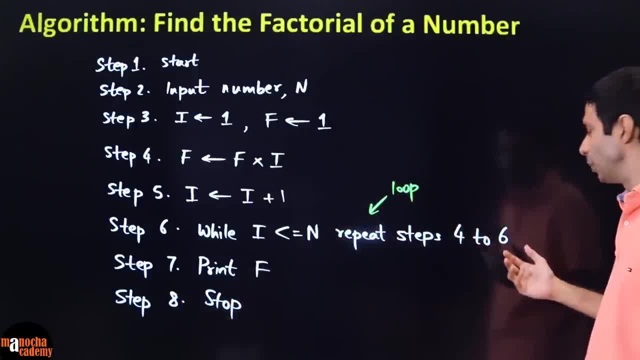 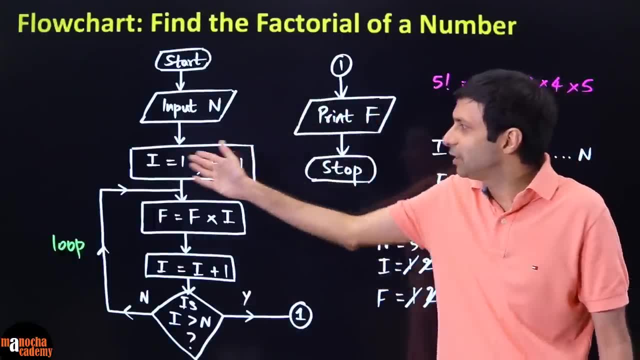 and you can easily address the step using the step numbers And flow chart. of course, lot of hard work drawing all these boxes, but very visual and pictorial and you can clearly see the flow of control. So that's why always remember to put the arrows. 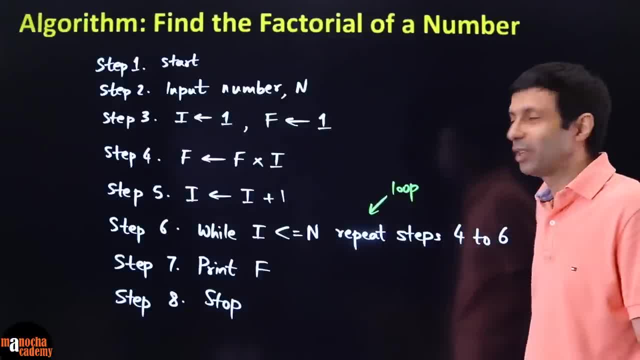 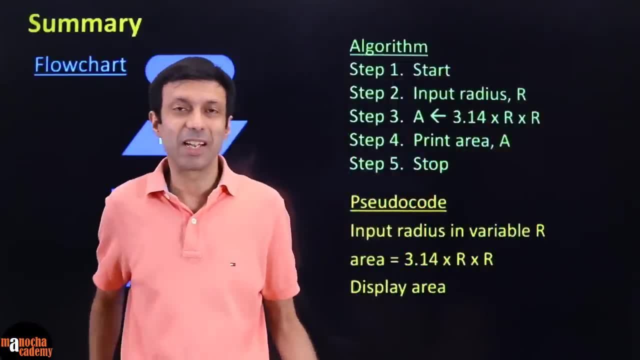 So which one did you like? Flow chart, algorithm or pseudo code? What is your favorite here? So here you can see. this is the summary slide. like we discussed, We have discussed all the different ways of putting down or writing our logic. 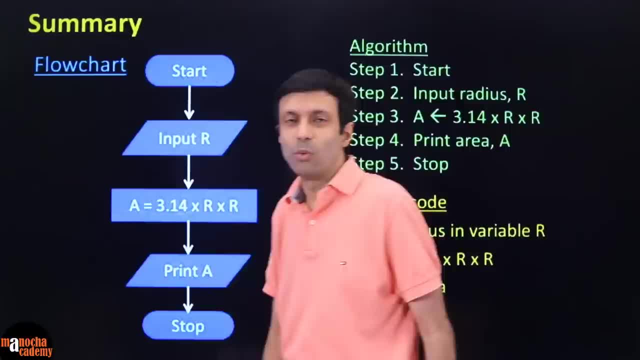 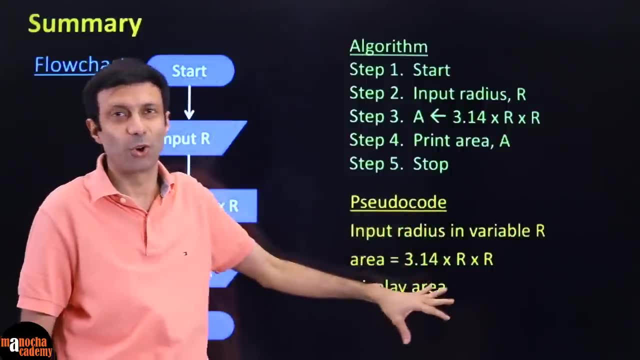 We can use flow charts like this. We can write it in a algorithm step by step style, or we can write this informal pseudo code. But good idea to practice all of this and, of course, when you are doing you know you are writing a real program.